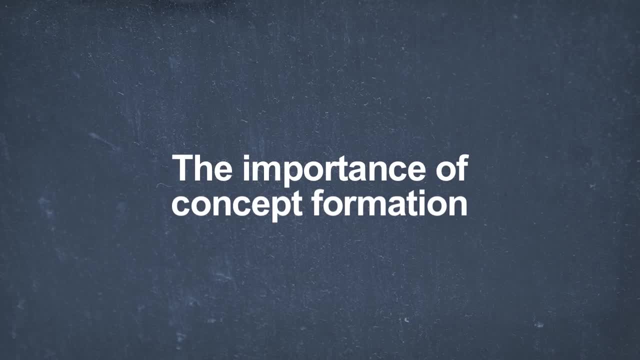 is condensing her introduction or, as I put it in the book, introducing her introduction From another point of view. I don't care for this subject, believe it or not, crucial as it is, because it's very technical. I'm speaking here personally, I'm not trying to bias you. 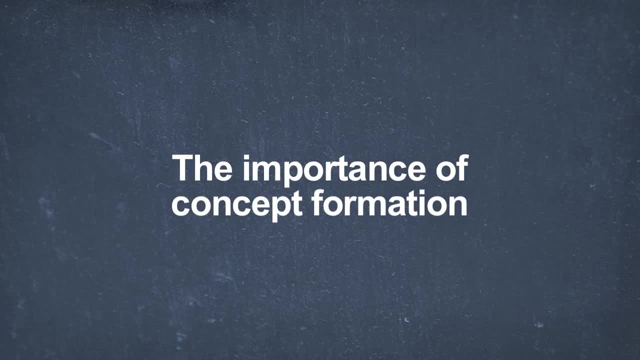 for information. but I went into philosophy because primarily, things in Atlas shrugged like Reardon discovering the connection between sex and economics, That really got to me What I call the mountaintop view, standing, you know, facing the totality and seeing these. 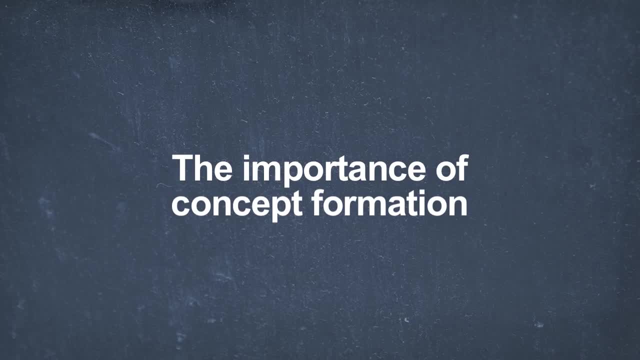 tremendous integrations, these broad-scale connections taking all the disparate parts of the world and making one comprehensible whole of it. But the other half of things- thinking, integration- is one, The other half is differentiation, distinction. What's the difference between unit of measurement and unit of a concept? What's the difference between? 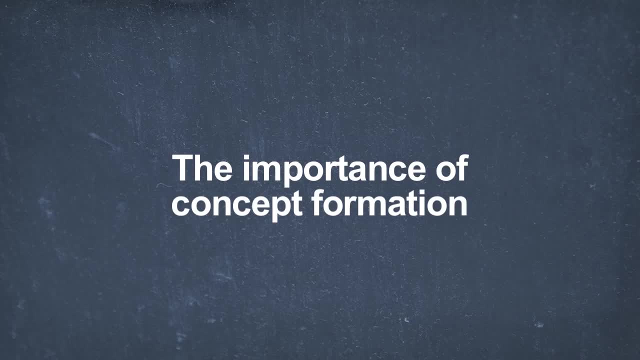 implicit measurement and numerical measurement, et cetera. That's the more technical side, and I never had any special interest in that because I'm not a mystic. so you can't integrate until you differentiate, So you can't really discriminate against one side of cognition. 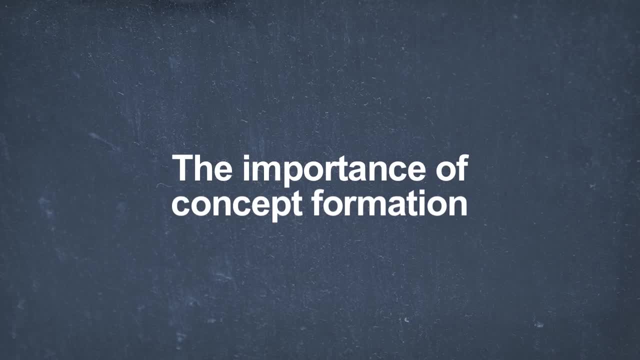 as against the other. Cognition is differentiation and integration. but I have a definite personal bias between synthesis and analysis. I much prefer synthesis, That's like the cashing in. Analysis, to me is just the grubby work of getting the elements clear. so then you. 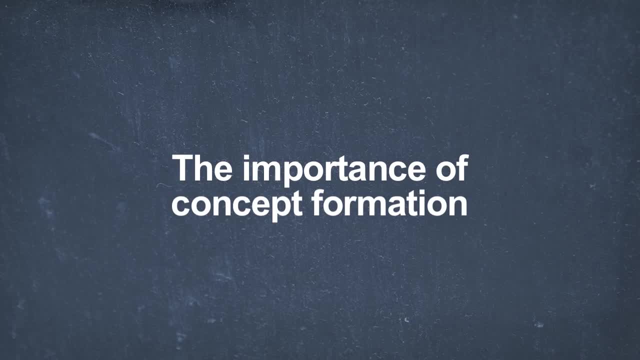 can have the grand synthesis. In other words, if I were to go bad, I would be a mystic, not a linguistic analyst. So I tell you in advance that that's my bias, but nevertheless, I was convinced that it was indispensable. I'm saying this, however, now, because if you're 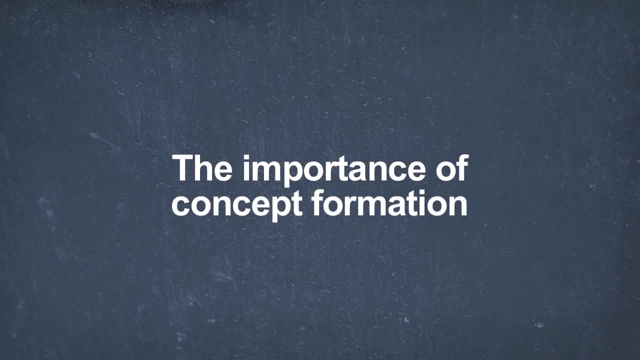 interested. If you're interested in that kind of super-technicality-on-technicality, I want to refer you to the second edition of the Introduction to Objectivist Epistemology, in which a whole bunch of professors who really want to be professors- and that's not a crime, it's just not what I want it to be- but who? 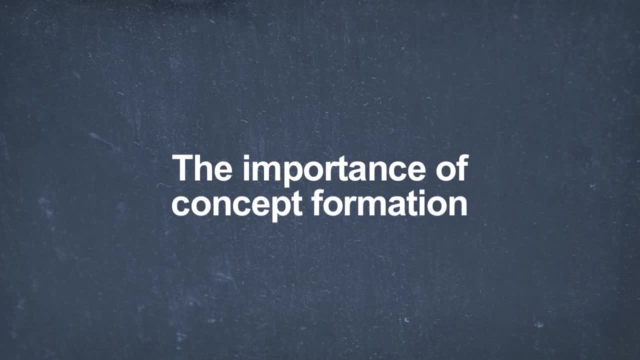 like technicalities and distinctions within distinctions and so on, put to her questions as detailed as they could and I'm going to refer you wherever possible to that And I'm going to refer you to that book where she has already answered it rather than bogged. 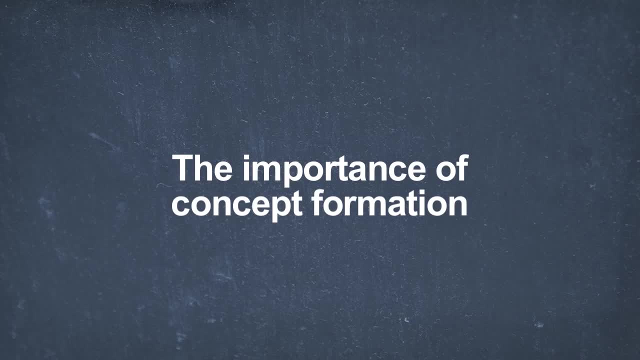 down here in super-professional hair-splitting. I want to keep the overall perspective that this is part of a total philosophy and not get lost in a morass Now. having said all that, I have to say that this chapter is the essence of objectivism this subject, So I 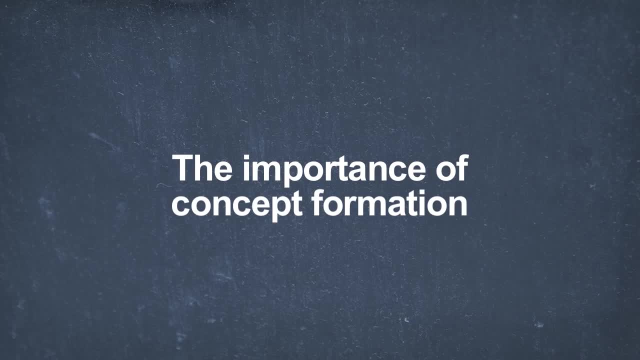 have a certain conflict: Chapters 1-2.. Chapters 1 and 2 are simply the preparatory. They lead up to it, They establish reality, what we're given automatically, that we have a choice. But then this is the core of what. 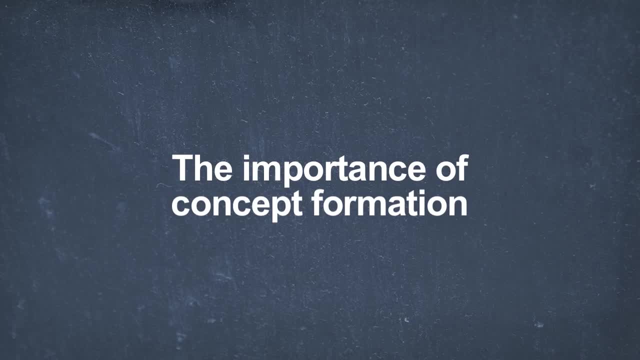 is the distinctive objectivist approach and everything from 4 on all the rest of epistemology, objectivity, logic, reason and then all of the evaluative branches and ethics and politics are all consequences and applications. And I make a big point throughout the book when 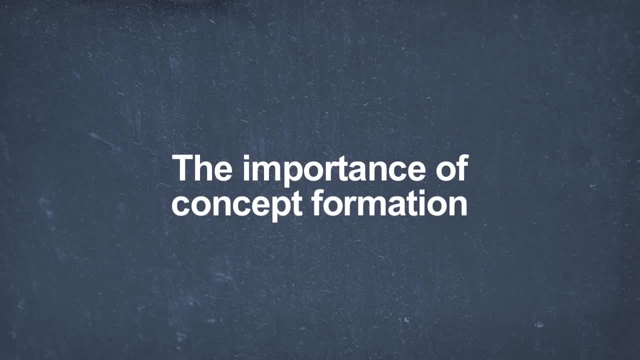 I get to Any key topic, to take it back to concept formation, I do that with reason and emotion, I do that with theory and practice, I do that through ethics, I do it through politics and throughout art, so that if you get this chapter, you really get the essence of it. So let's. 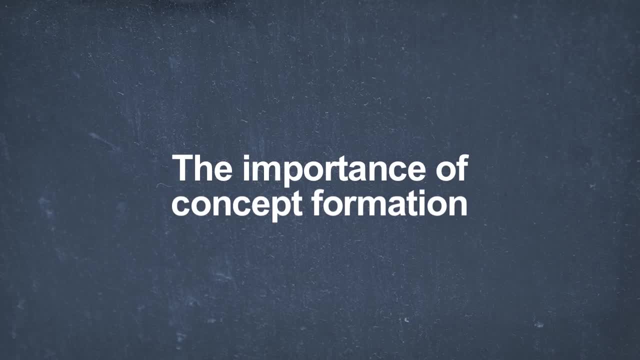 try to compromise and say: get the essence of the essence, even if you don't get every detail of this. Now, Ayn Rand herself regarded this topic. Chapter 2.. Chapter 3.. Chapter 4.. Chapter 5.. Chapter 6.. 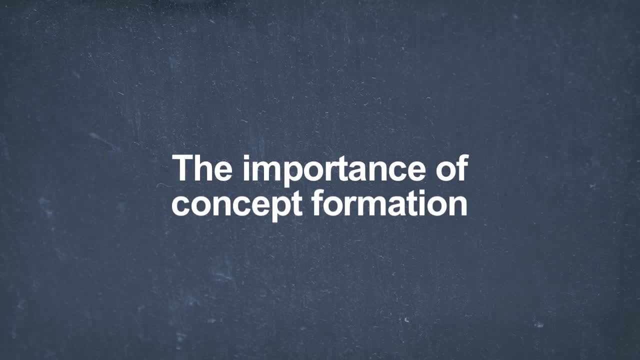 Chapter 7.. Chapter 8.. Chapter 11.. Chapter 12.. Chapter 12. as essential to underpin her novels and that's why, of all the possible books that she could have written in nonfiction terms, she did essays. but the only sustained monograph that she did was on this topic, her own mission as you. 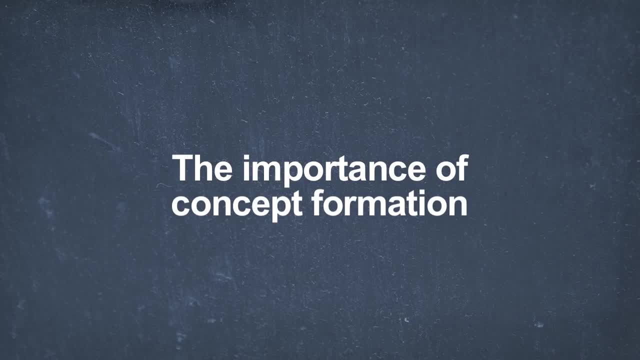 know in life was to present the ideal man. but after she presented it, she knew that one crucial thing was necessary to make it stand, and that was to validate the ideal man's means of grasping or dealing with reality. the essence of the ideal man was the man who relied on his mind. well, if she was to validate that, 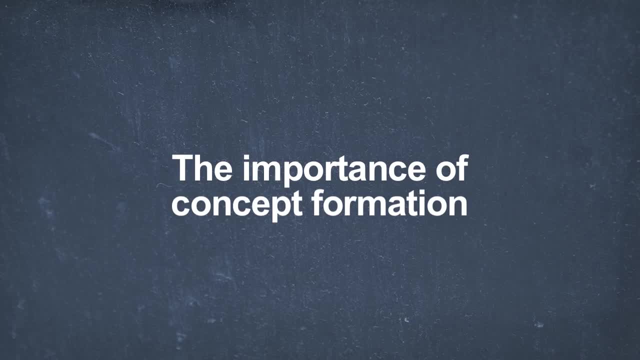 view of man all the way down. she had to show that it really was true that the mind had the power that she presented the mind as having. in other words, the mind really was an instrument for knowing reality. and that means she had to show how does the mind actually work and how does it relate to reality and 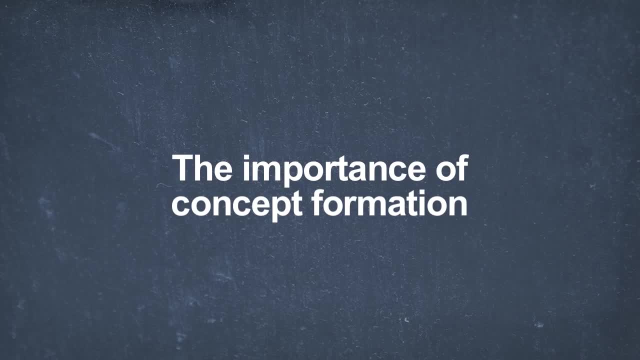 that really became her mission and that's what she did and that's what she comes. the problem of concept formation, because on the perceptual level there is no problem. you open your eyes and you see, even though philosophers have made a problem. but on the conceptual level it's a different proposition. now I asked her: 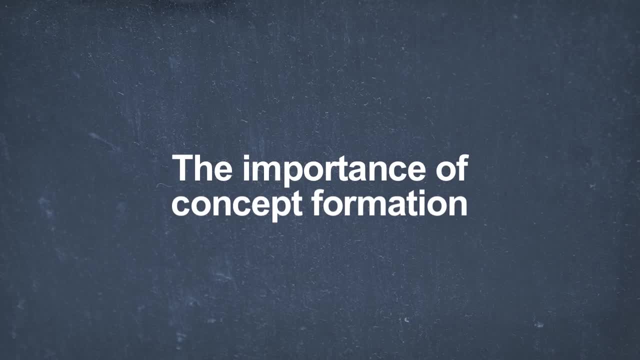 once. do you think an intelligent layman, honest, independent and so on, but not a professional philosopher, would have to know, or should know, the theory of concept formation, should know the stuff in this chapter? basically, you know, in measurement, omission and all that. and she said to me he has to know that there. 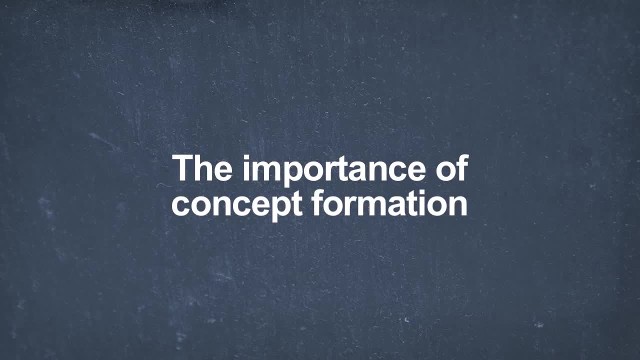 is an answer, even if not necessarily what the answer is. that is, he has to be able to know that there is some kind of definition and explanation of what concepts are, even if he himself doesn't go into this level of technicality. now I would perhaps myself elaborate that a bit like this: if you're a layman, you have 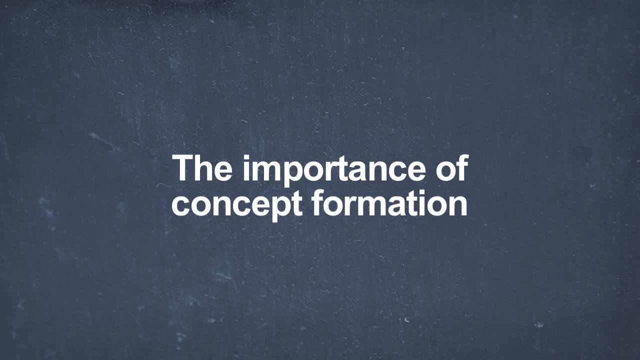 to know this much about concepts. I'm saying this in advance because you may miss a lot of technical points, but this much you should keep throughout. Concepts are man's form of organizing sense, experience, sensory data, Even if you only know it in those common sense terms. that, of course, will not be a 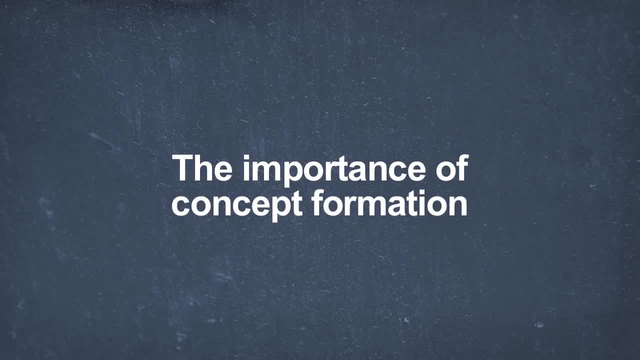 complete validation, but for practical purposes. you have to know that much as against two incredible errors: One that ties concepts to any form of the supernatural, that makes them revelations, communications from the beyond, etc. And the other that ties concepts to any form of the arbitrary, the subjective, the 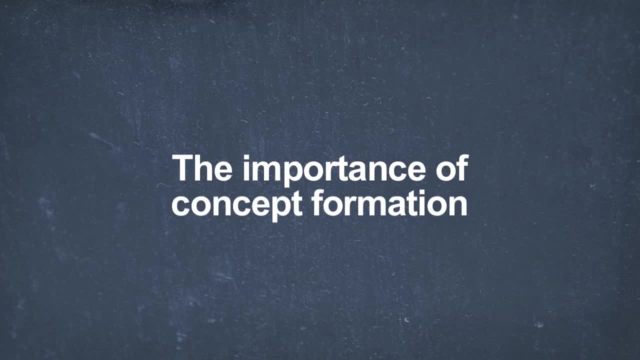 social, any idea that human beings can do whatever they want with concept. If a person simply has, in the simplest terms, the common sense terms, a word like table as my way of holding a whole bunch of concrete, that has nothing to do with God, but I have to do it by certain. 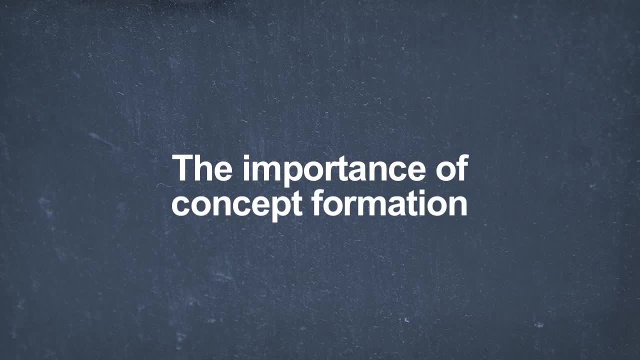 objective rules and not by whim, arbitrarily or the caprice of society. I would say that's the minimum that an intelligent layman has to know And of course he has to know, in some terms, the method of definition, because without knowing that he won't know how to clarify and define his concepts. 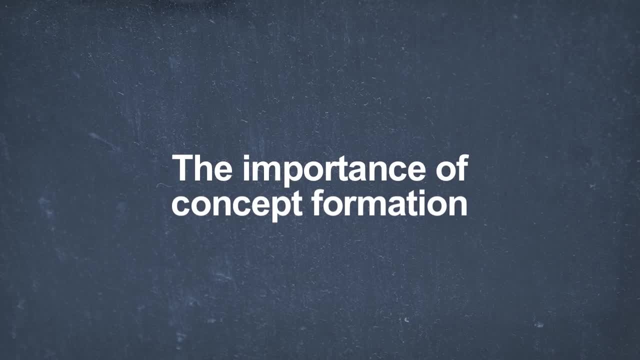 Now, all of you here, of course, are far beyond the status of layman simply by virtue of coming to this course and reading this book, if for no other reason. So I'm saying this to allay any guilt or anxiety you may feel if part of it. 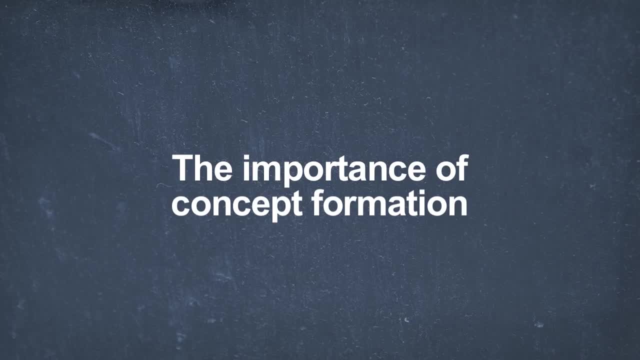 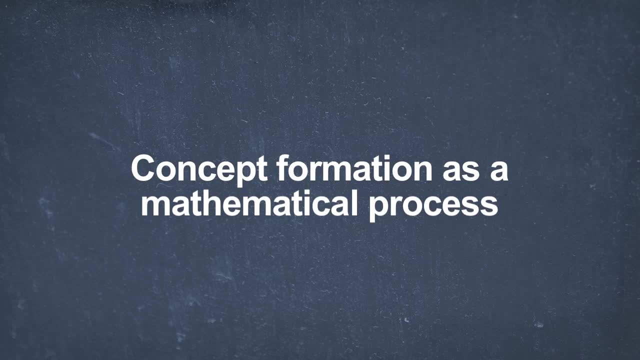 either doesn't interest you or washes over you. This is a unique chapter in that regard. All right, now let's take an overview of the content of it. First sequence: differentiation and integration as the means to a unit perspective is concerned, to describe the process of concept formation as we 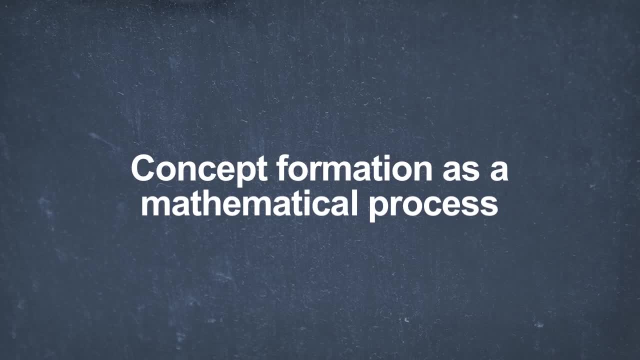 experience it consciously. Now take the various aspects of concept formation. observe similarities that differentiate a group of percepts from other things. isolate that group. You abstract away from the differences. you integrate the segregated percepts, make a single new mental entity out of them. 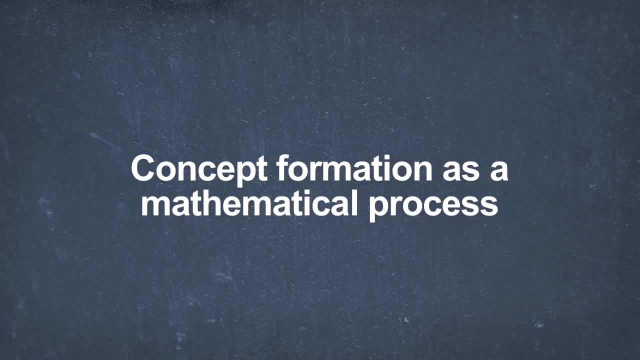 a process which is completed by choosing a symbol, a perceptual symbol, a word, and that word then holds the integration and stands for all of the percepts that you integrated, plus anything else which comes under this concept, past, present or future. 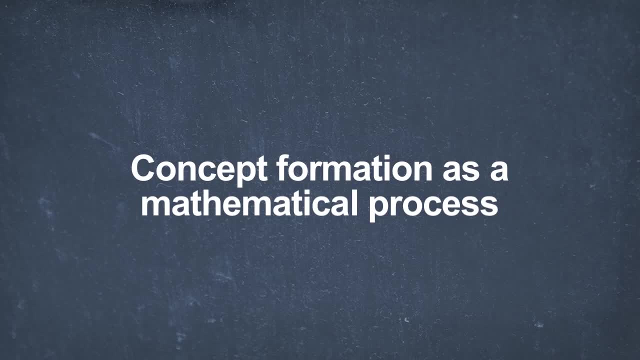 It has an unlimited number of instances all held together in that one unit as a result of your segregating a group of percepts, stripping away by abstraction their differences, and then they're all identical at that point, giving a name, which is that open-ended application to all instances. 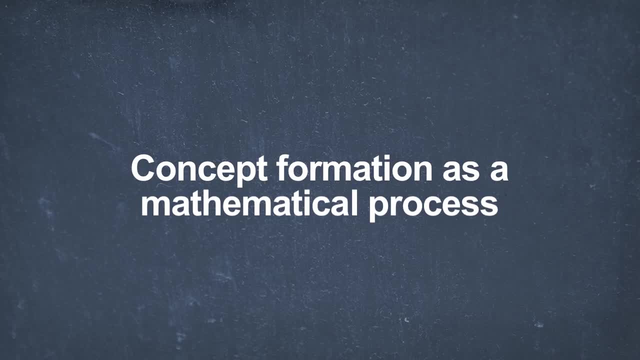 That, basically, is the concept. It's not completed. It's not completed until a word is chosen And I elaborate, and when we go over it in detail I'll discuss some of those more specifically. but that's the overall process as we experience it. 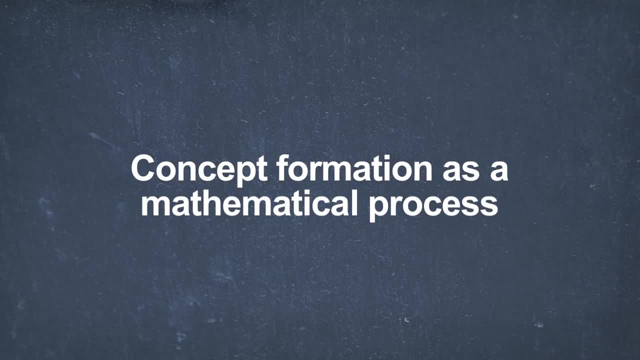 Now, of course, the problem, the philosophic problem, is not on this descriptive level, but what's called the problem of universals, which is, when you abstract away from the differences, what's left. And you know that philosophers delight in saying that. 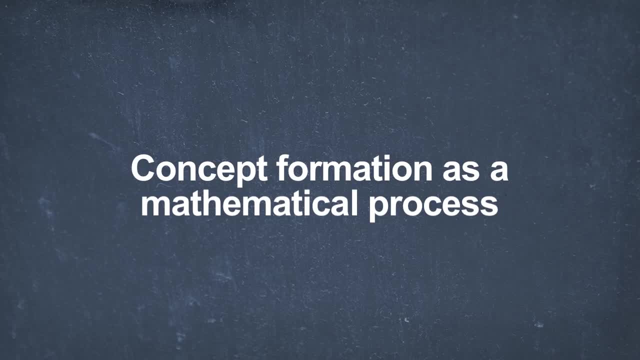 they can't find anything. the same among all the instances of a group, When they abstract away from all the differences, they can't find anything. They don't find any madness in man or roseness in rose, And so what is it that the concept actually refers to in reality? 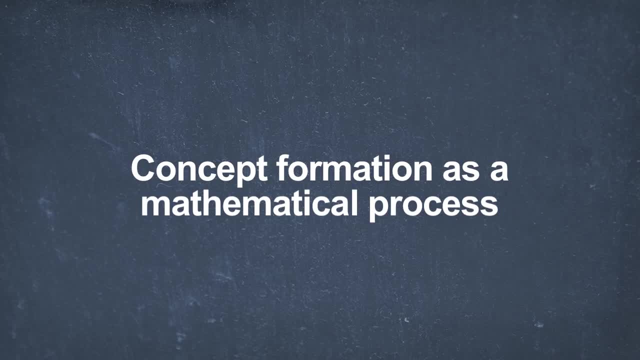 Since everything vaguely resembles something else, we just arbitrarily draw the lines or what, And it's to this problem which I assume you're familiar with. I'm not. I'm not going to labor to make the question real, but I think I discussed it in the text. 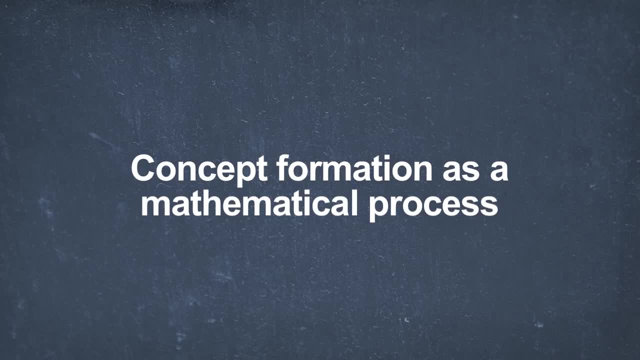 It is to this question that Ayn Rand came up with her unique, unprecedented answer, and that's in the section on concept formation as mathematical. That is the core of her discovery. Now a good, I think, general layout of the parallels, the similarities between concept formation. 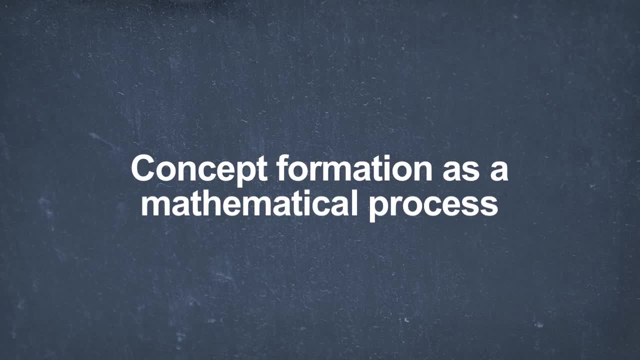 and mathematics is offered to you on page 123, which I find helpful because it simply point for point, parallels the two processes, The connection between measurement and conceptualization, and I say on the bottom of 122, the two processes, measurement and conceptualization, have the same essential purpose. 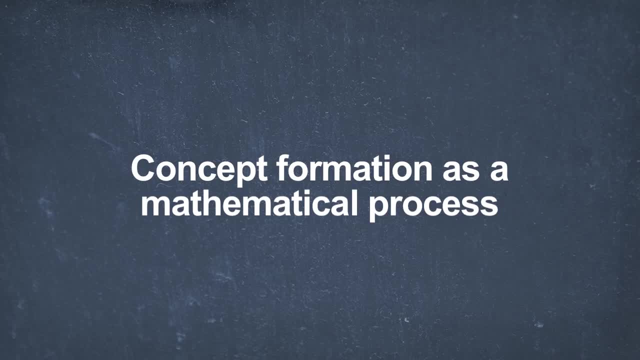 and follow the same essential method. They're after the same thing and they do it the same way. basically, And that is the essential connection. And then I elaborate on those two paragraphs in 123.. Now for concept formation. think as an example taking individual men. 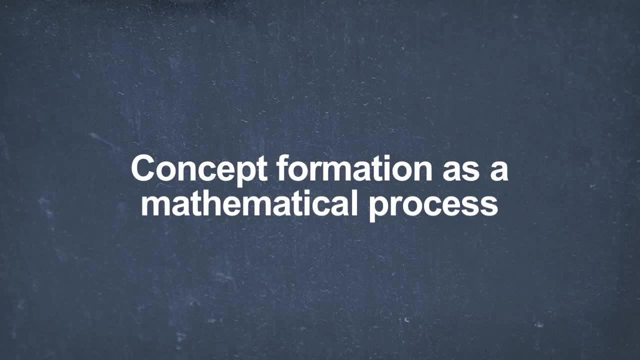 and relating them to the concept man and thereby to all men, past, present and future. For measurement, take an inch or a foot, say. Take an inch because a foot, you'll think of your toes. Take a foot as a unit of measurement and then you measure all distances. 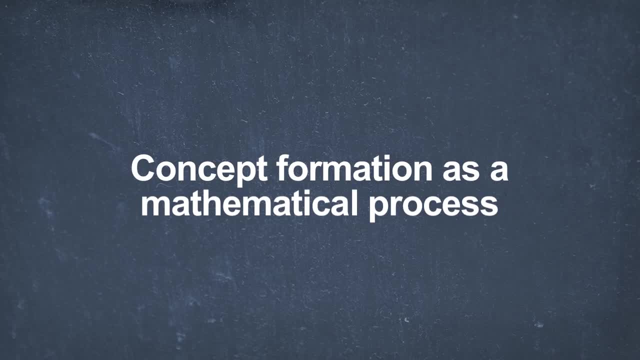 including the distance to the moon in terms of its relationship back to this perceptual unit Now. so in one case, man, we have concept, and in the other case- foot or inch, you're going to say- we have measurement. 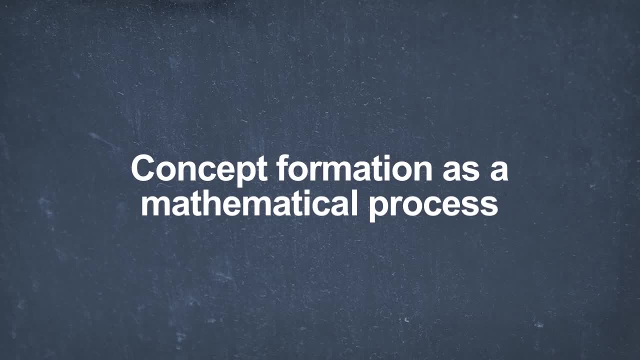 Now, in both cases we identify relationships among concretes. We relate inch to other lengths or one table to another. We have to be sensitive by its similarities. In both cases we have to take as our foundation, as our start, directly perceived concretes. 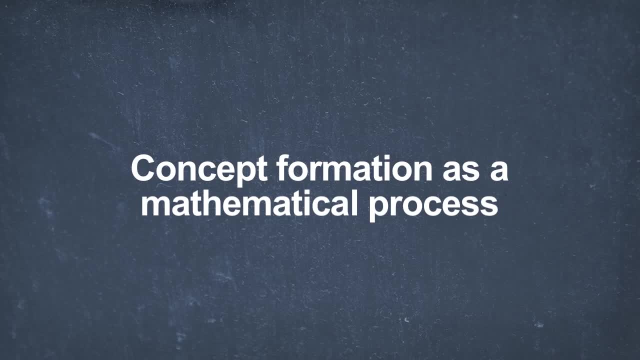 They have to be within our frame of perception. Your unit of measurement, for instance, couldn't be a light year, the unit of length, because that's beyond your frame of perception. You take some perceived concrete as the base and then you relate everything else in the universe. 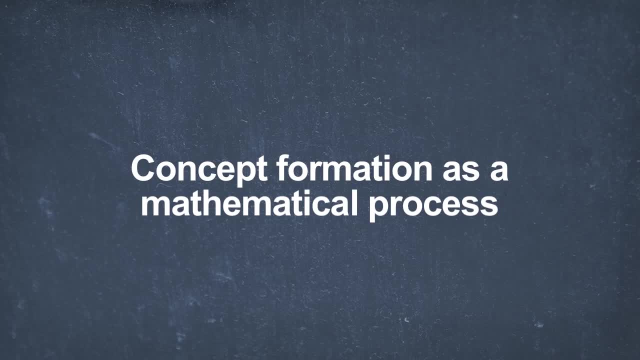 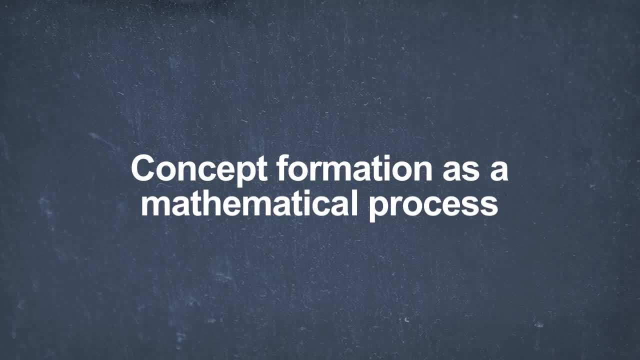 So, in the case of the example of man, you can now have information about all men past around the earth and in the future that you will never perceive, simply by reducing them all to the little handful of men that you do perceive. It's in that sense, you take the few you do perceive and relate an endless number. 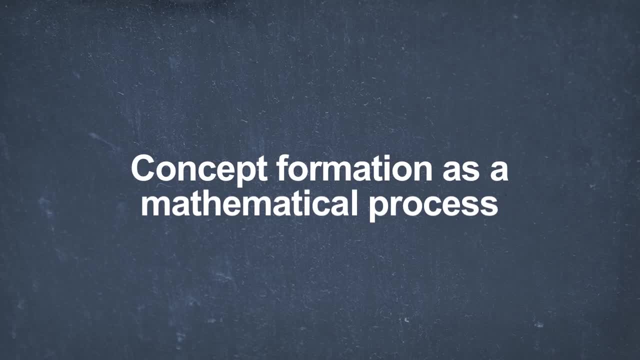 For all we know, there are equivalents. There are equivalents throughout the universe, but we bring the whole thing throughout to the range of our knowledge by somehow taking what we perceive as the base and bringing everything else into relation to it, And the same, of course, is true in measurement. 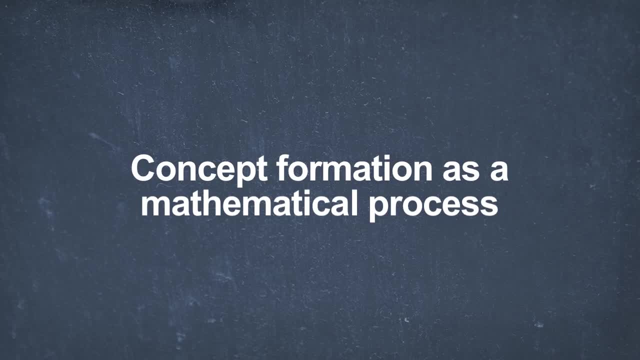 You can measure, if you have the techniques, any distance anywhere throughout the universe, as long as you have something like an inch or 12 inches of foot, that's directly before your eyes that you can relate every other distance to. So that game, you see, it's starting with. 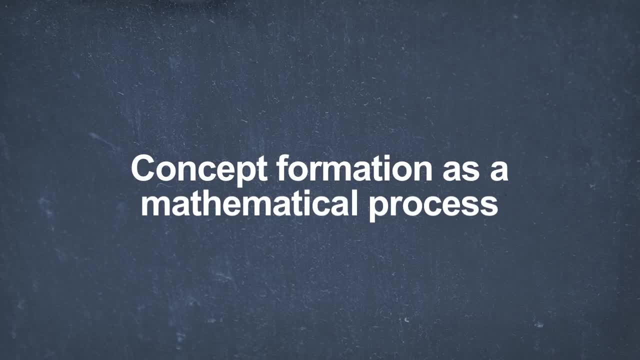 It's starting with the perceived and bringing everything else into relationship to it, And the result is the entire cosmos becomes accessible to us by this unique method of reduction to what we do perceive, through a type of relationship. And now the cherry on the cake is Ayn Rand's discovery. 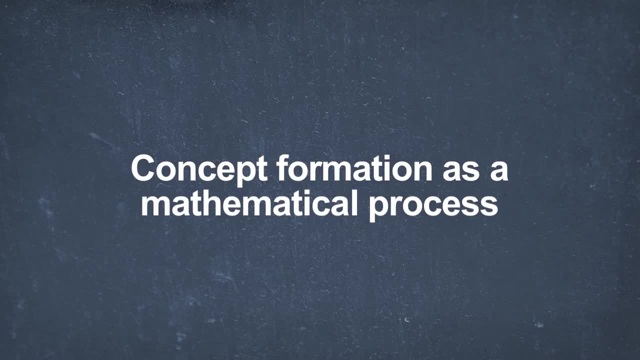 I shouldn't introduce it in that flippable way. I mean the climax here, the real thing that solidifies the parallels between the two, Between mathematics and concept formation. In both cases you bring concretes into relation by quantitative means. 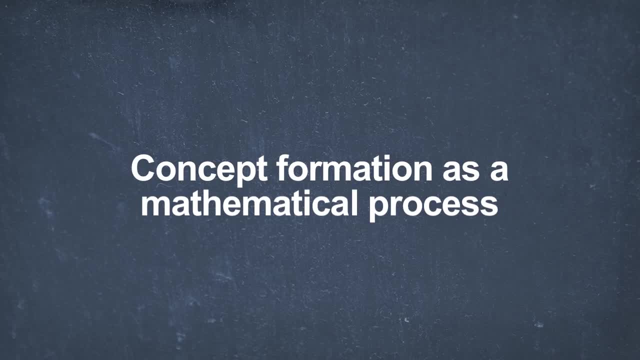 In both cases you discover a mathematical relationship between the concretes you started with and the rest that you bring into relationship to it. So it's not simply you generalize what you bring into it, You bring the Rest of the universe into relation to what you perceive. 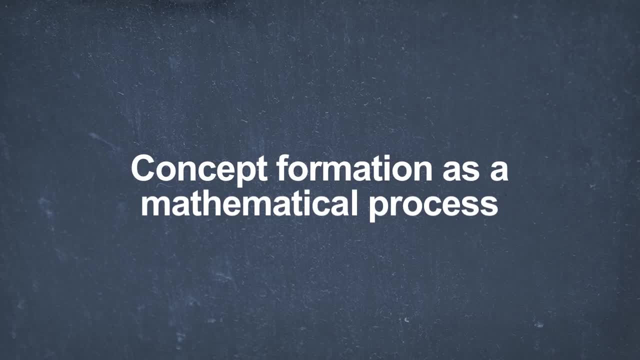 You specifically bring it into mathematical quantitative relationship. And, of course, on measurement, Unit of measurement example is simple. You ask an inches related to the distance to the moon. How, How many inches? Every length differs from another according to how many of these units of measurement. 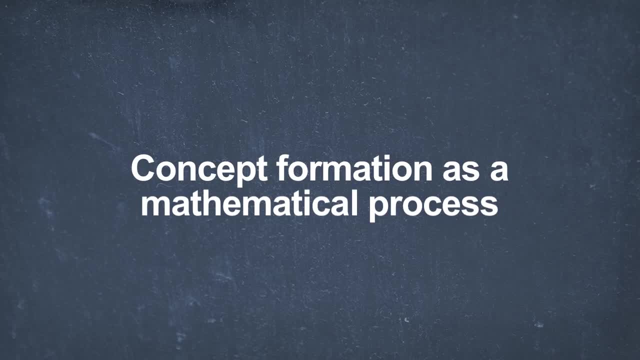 And we can measure any given one quantitatively by saying how many units Quantitative. And we can measure any given one quantitatively by saying how many units unit. Now, in a very similar fashion, how do other men differ from the men that you? 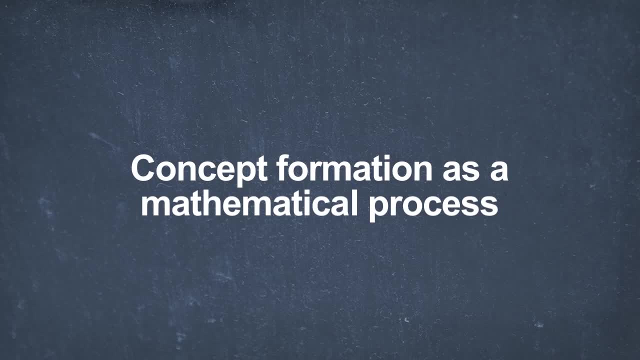 directly perceive. How does any one man differ from any other? And Ayn Rand's point is: one man differs from another in principle, the same way the distance of the moon differs from the distance of an inch in measurement Concrete, within a concept differ from one. 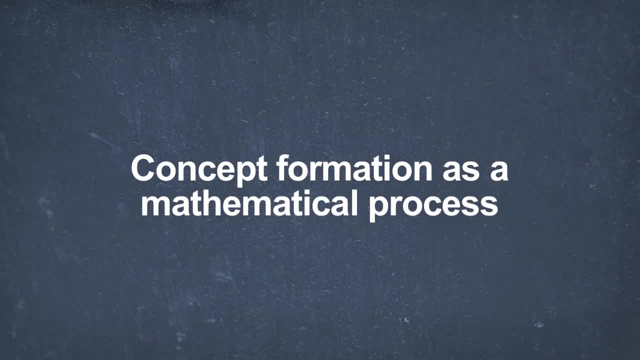 another, in the same way that the unit of measurement differs from any other distance or any other element being measured Quantitatively. So it's actually that you're doing the same thing: You're starting with a perceived element and then you are quantitatively relating everything else in. 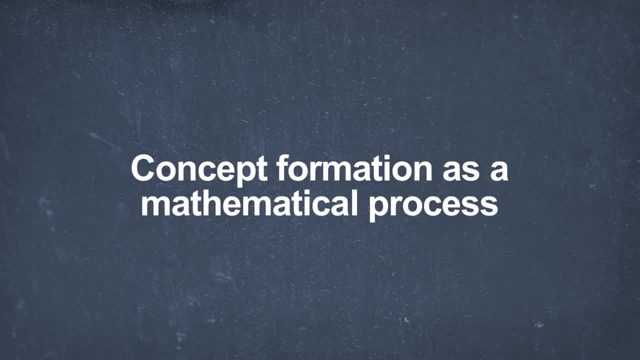 the universe in that category, to the perceived element, And thus her statement that what is common to the entities that come under a certain concept is their characteristics, their attributes, And what varies is only the measurements When we form a concept. therefore, this is the underscored. 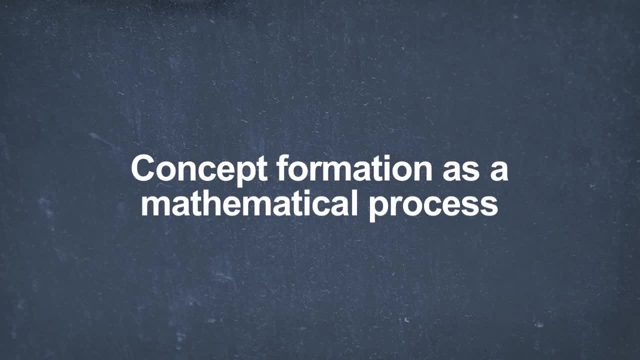 statement in the middle of 123.. Our mental process consists in retaining the characteristics but omitting their measurements. That is the decisive formula. When we form a concept, we retain the characteristics but omit the measurements. And when we do that, our mind grasps the identity of all these instances. They vary. 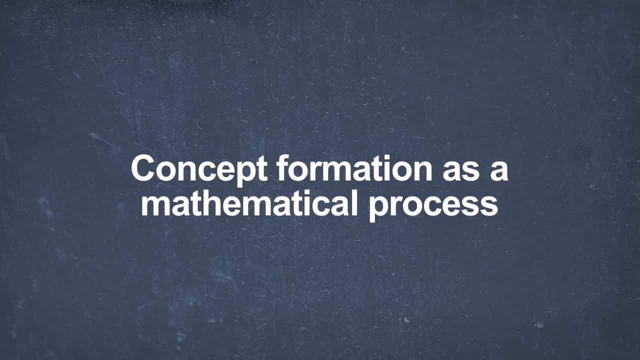 only in measurement, When we strip away or drop off the measurements, what we have left as concretes that we could easily integrate into a unity, because we stripped off what actually distinguishes one from another And then put a word and we have a concept. Now the key to grasping: 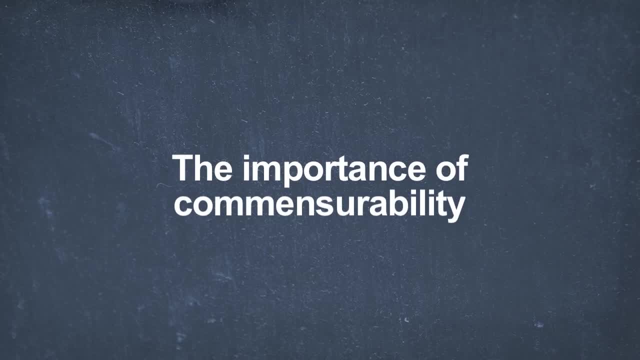 this theory is over on the next page in a single term- and that is the first, or I guess the second first of my underscored words on 124, line 5 of the text commensurable. That is really the key to. 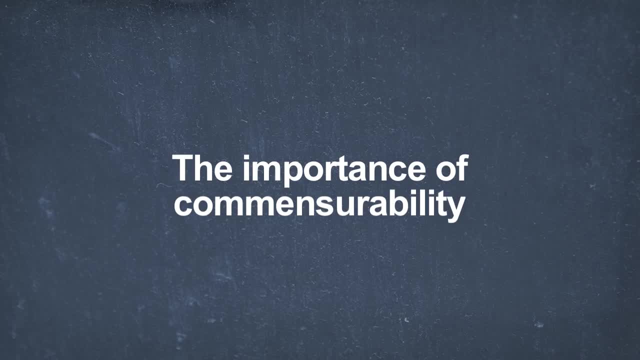 Ayn Rand's theory. here All the instances taking length as the example under a certain concept are commensurable, That is, they can be related to each other. They can be related to each other. They can be related quantitatively to the same unit: All lengths: the length of a ribbon, the length of the 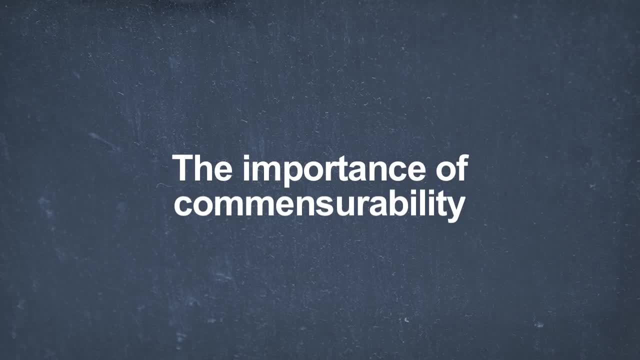 moon, the length of this room, the length of a pin- all can be related- can be measured in terms of the same unit, for instance an inch. On the other hand, color can't be measured in terms of an inch. A red. 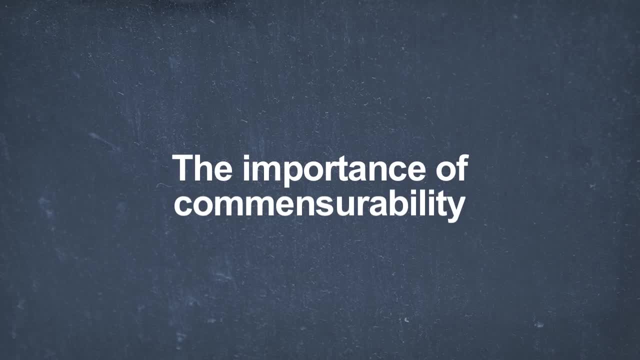 patch can't be measured in terms of an inch. You need a different unit to measure colors and weights, velocities, etc. But whenever the instances are commensurable- that is the key- They're all reducible to the same unit. 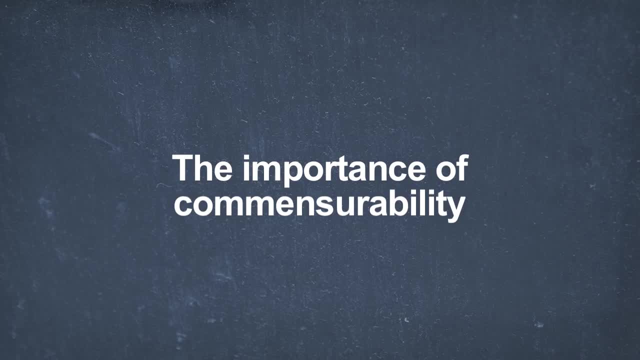 So what we really do when we bring together concretes that belong under a certain concept, we're able to relate them to each other by virtue of our mind's ability to bring them back to the same unit. That's the relevance of commensurability. 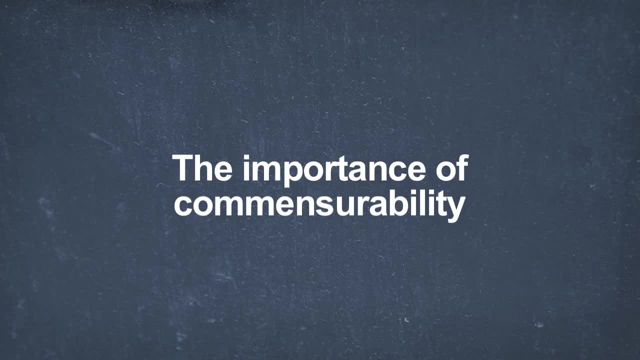 We can take together five or ten concretes which vary in many ways, but we can hold them all into connection with each other because our mind grabs that each of them can be brought back to the same one unit. On the other hand, if I give you an incredible disparate, motley collection of things, for instance, 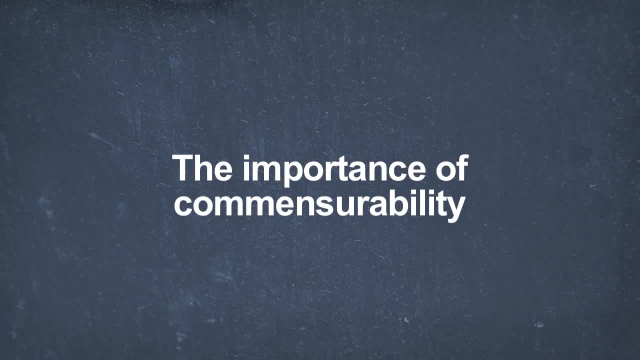 the Rachmaninoff Second Piano Concerto, The Square Root of Two Rotten Banana and my after image of the American flag and say now integrate. you simply can't do it. your mind absolutely box to put them together into anything, because there is. 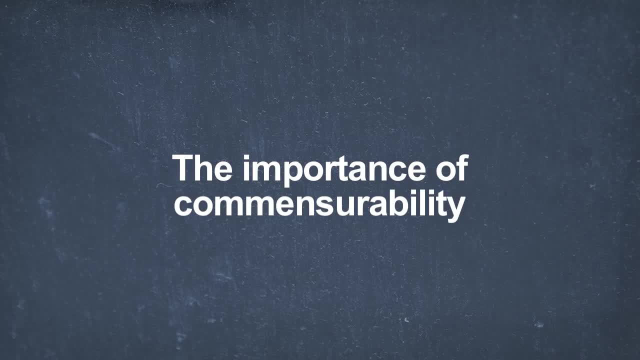 no way you can relate them all to the same unit. there's no way you can even do with man. of course we have to do it through his attributes. but we can say he has arms, but which vary in length. he has a head which varies in shape, which is 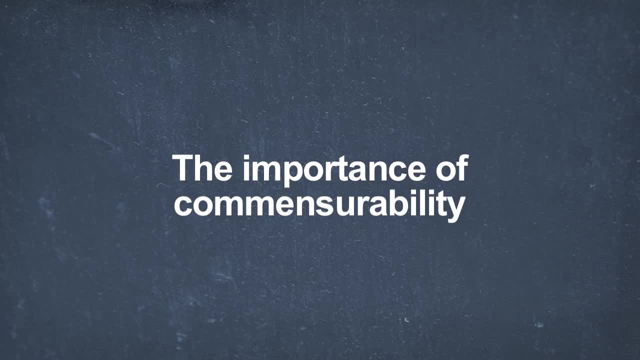 measurable. he has a body which has a weight which is measurable in all cases. we can take and put men together, because the variations are only in measurement and with. therefore we can relate every man, in terms of the various attributes, to the same set of units and thereby all of them to each other. but when that? 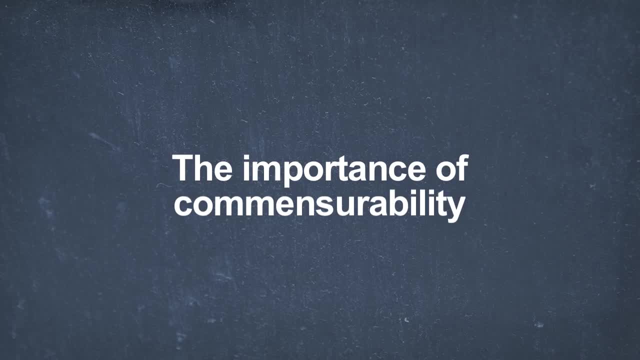 incredible collection which I can't even remember, but I just gave you. you couldn't do it because your mind just stops dead. there is no. none of those things are commensurable, nor nor are they attributes commensurable. it's not as though they're like all of you with the 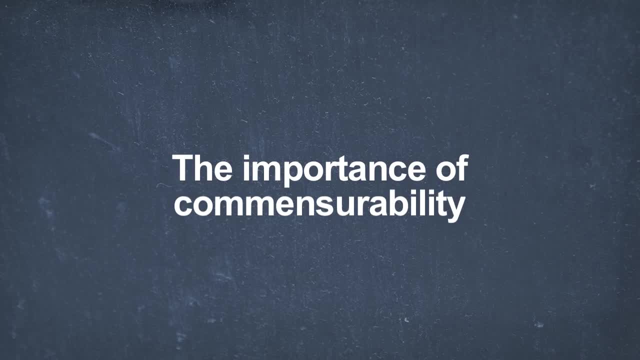 same characteristics, differing only in measurement. there they just simply. your mind can't do anything with it, and that is the issue of the importance of commensurability: commensurability. so when you grasp, you turn to 127: similarity. that's your perceptual experience on the conscious level. you look out and you 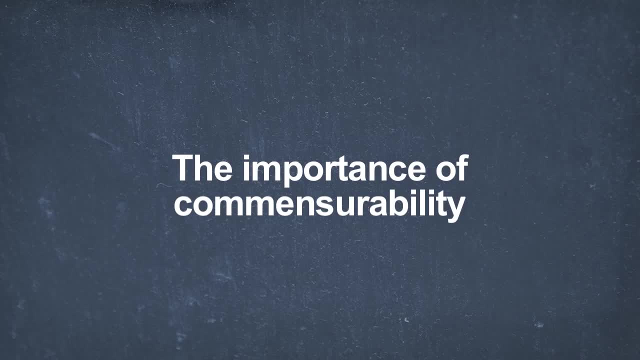 grasp that to men are similar. but the deeper point is that I said as a top paragraph 127, the grasp of similarity is actually the mind's grasp of a certain mathematical fact, namely that all these similar concretes are commensurable, but they are reducible to the same unit of measurement. now, if it's in the case of an entity, it's. 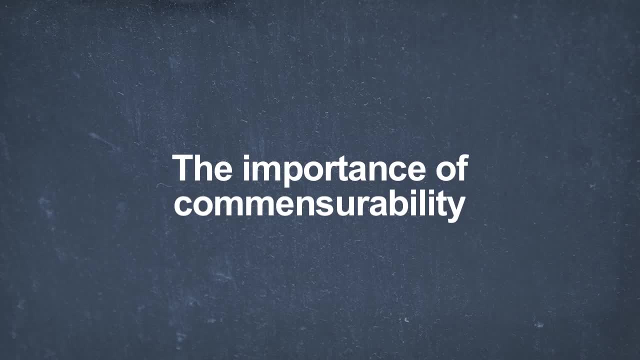 It's not just one unit. you measure entities through measuring their attributes, So it's many units. but then all of those attributes would be possessed by the entity and all of those units for each attribute would be commensurable. And then here's my- I think, most clarifying sentence. if you're with me, a man can relate. 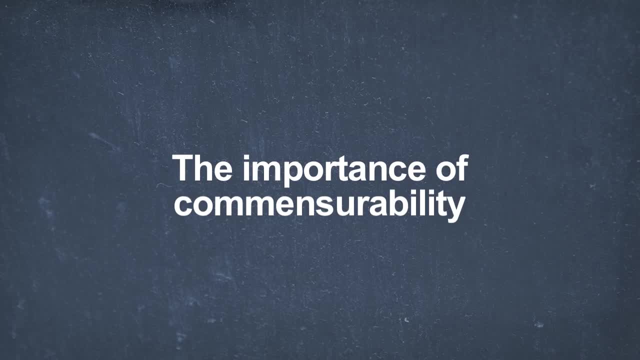 these concretes to one another, bracketing them mentally into the same group. that is all the men you perceive. You can put them all into the same group Because you can relate each quantitatively to the same standard. The only difference is the particular measurements of this relationship in the several instances. 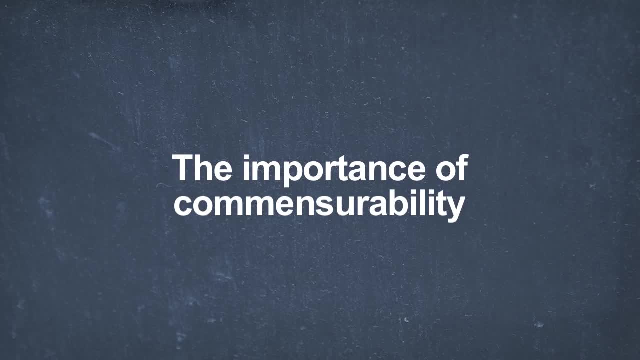 And therefore, once you have this perspective, all you have to do to form a new unit is: just don't specify the measurements, just omit them, don't focus on them- which your mind does for you by the nature of the conceptual faculty- and the result is you will have a 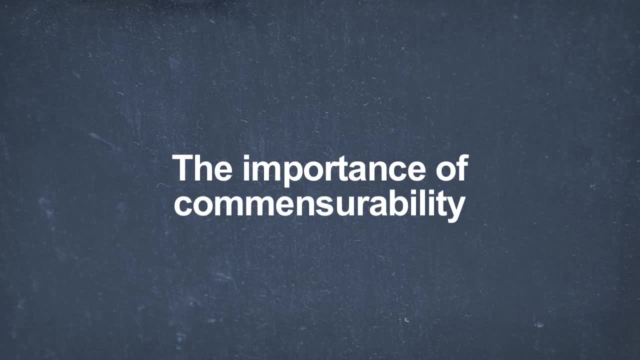 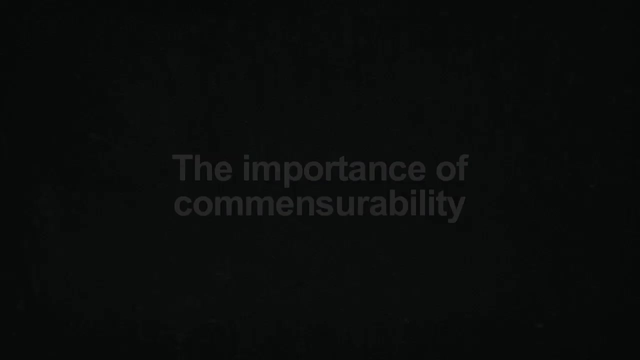 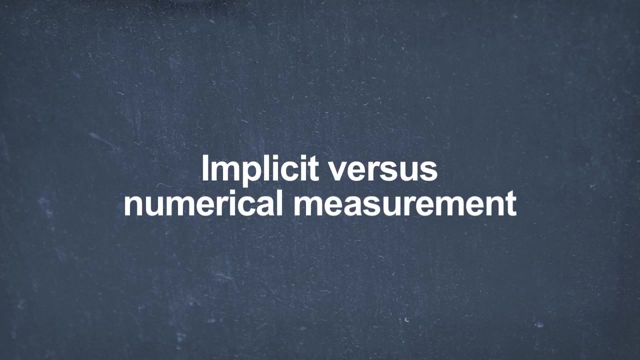 unit standing for all of them. So if you ask Objectivism, what is the same among the units of a concept? The answer is obvious: the characteristics, apart from the measurements. They are identical once you abstract away from measurements. Now I want to point out here one problem that you may have, that I deliberately put a new 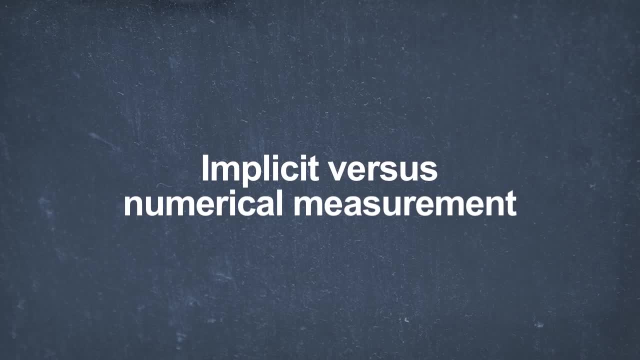 passage. This is about the only new passage. I got it, of course, from Ayn Rand, but it answered a question for me that always bothered me. Let me tell you the question. I went around this several times with her before I got it straight. 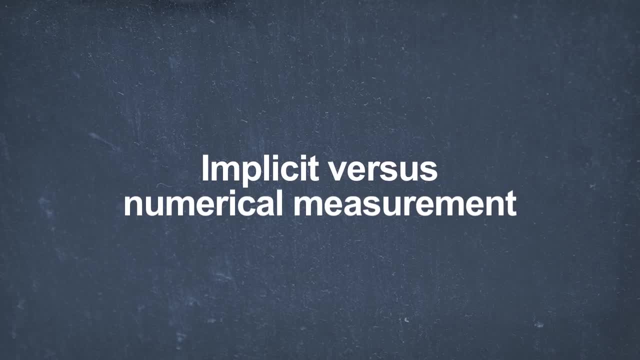 This is the problem, as I put it to her: Our early concepts, our first concepts, are formed far before we know anything about measurement, Far before we are capable of measurement or even capable of counting. So how can we omit measurements? How can we omit measurements before we ever measure or even have any idea how to measure? 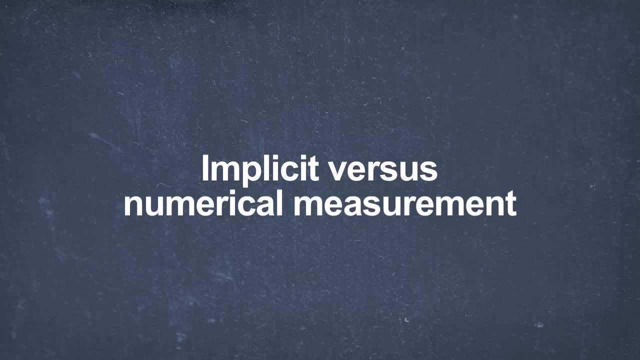 And I think, as I put it to her, how can we omit measurements yet never take any? And that bothered me. Now, that showed that I had a very inexact and unclear idea of what measurement omission consisted of. It was as though my idea of measurement omission was: first you measure the distance of this. 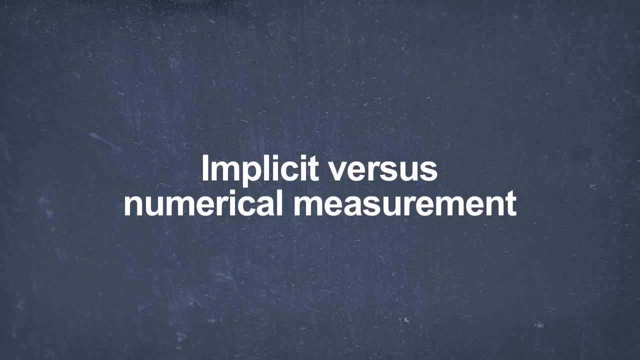 stage And you get that it's 12 feet. And then you measure the length of the chair and it's one foot. And then you measure this and it's one inch. And then you say, okay, I'm going to forget 12, one foot, one inch. what I got left is: 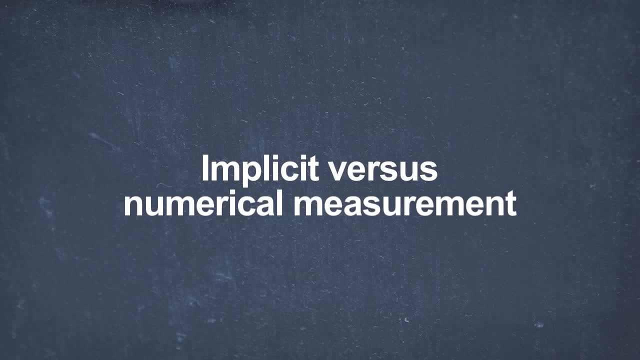 length. But obviously you can't go through any of that. You get the concept length far before you get numbers and units of measurement and the ability to count and all the rest of it. So how can you do it? Now, the answer that I give to that is from 1.24.. 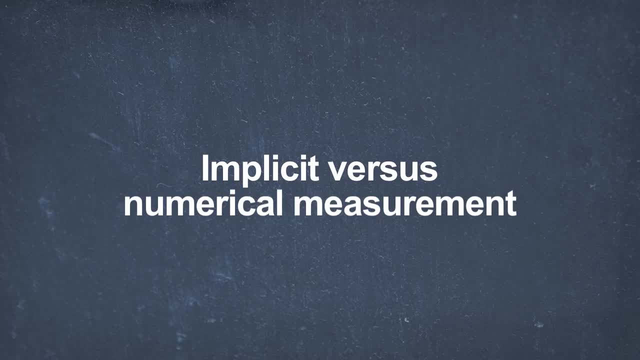 That's from 1.27 at the bottom to the top of 1.29.. And I make a distinction between implicit and numerical measurement. They're both measurement, They're both establishing a quantitative relationship to a unit of measurement, But one is explicit and using numbers. that's the numerical measurement. 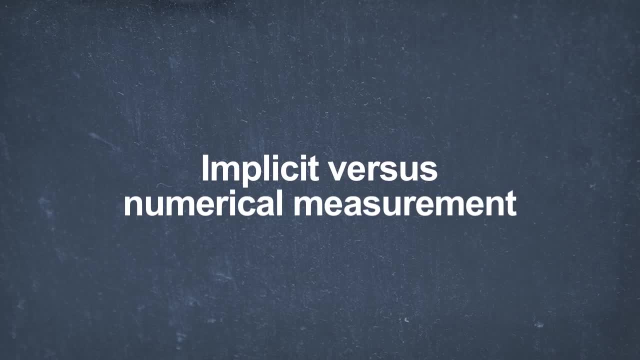 The other is implicit And it's not done by the use of numbers, It's done by direct perception And the description of it. it starts on the bottom: 1.27.. That paragraph at the bottom merely explains that numerical measurement, measurement as 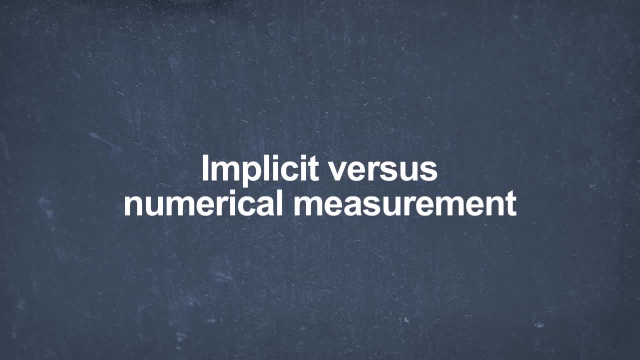 a conscious process requires a substantial conceptual development, but that that does not apply to concept formation. And then 1.28. That big paragraph. If there is the substance of the answer, We do not. I'm not going to read it all, because presumably you've read it, but just the part. 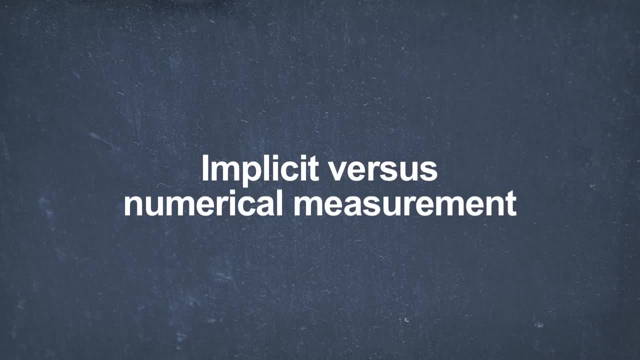 that's central here. We do not need a knowledge of numbers, because for concept formation we need to discover commensurability, not specific quantitative data. We don't have to know this is 12 and this is four and this is six units. 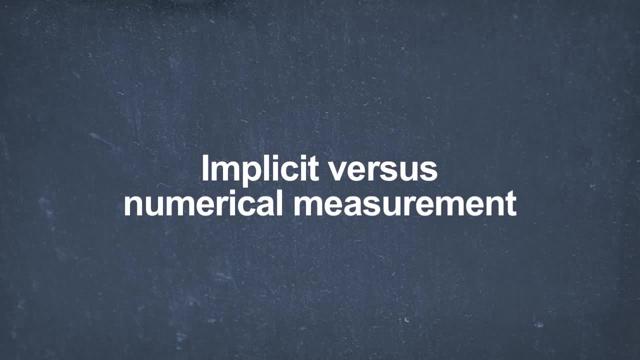 That's precisely what we're ignoring in concept formation. Therefore, what we really need, where the measurement we're talking about, is the ability to relate to the same unit, And that does not require precision, That does not require numerical formulation. All you have to be able to do is grasp that all the instances of a certain concept, that 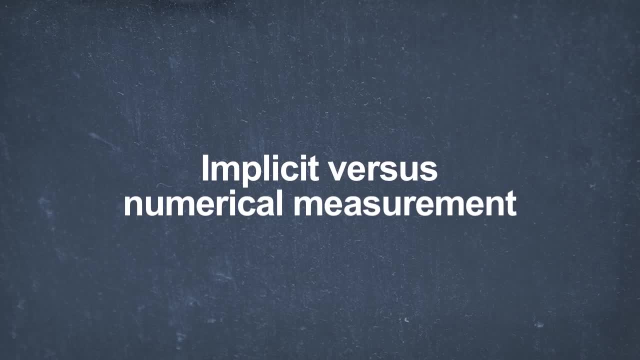 you're going to form come back to the same unit, That they merely are more or less of the same unit. The point is that you can do, without any numbers whatever, How- This was Ayn Rand's answer- Only by observing. 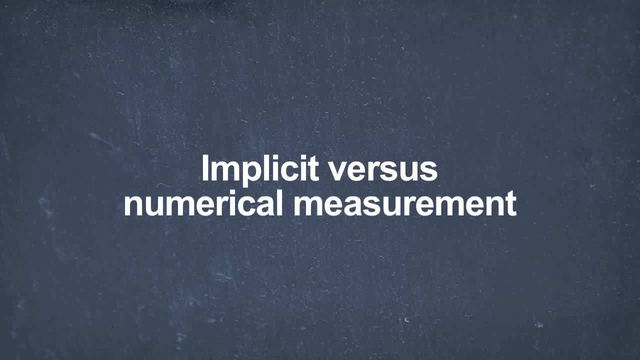 I mean, you can do it simply by observing the spectrum or continuum of more or less within any given attribute: Longer, much longer, shorter, much shorter, or hotter, much hotter, much, much hotter, etc. Now, distinctions of that kind of more or less within a given attribute. 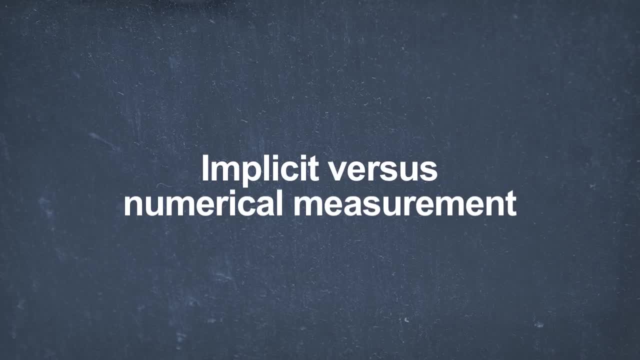 Are directly perceived, ahead of knowing how to measure them. A child can tell that this arm comes out much more than this by direct observation, without having the concept of length and without having to measure them. He can simply see one extends further than the other. 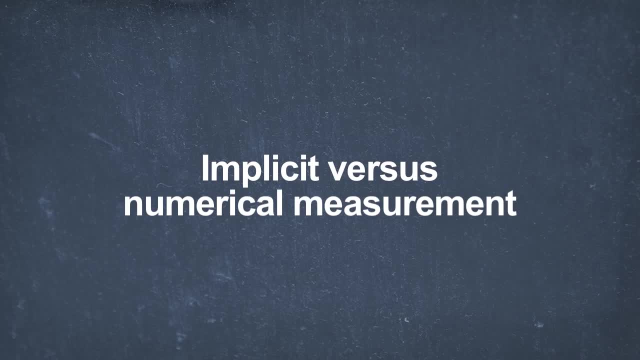 If he couldn't. we couldn't get to the conceptual level at all if we weren't given elementary data of that kind. All you have to have to engage in the type of measurement we're talking about is the ability to measure. That's the point. 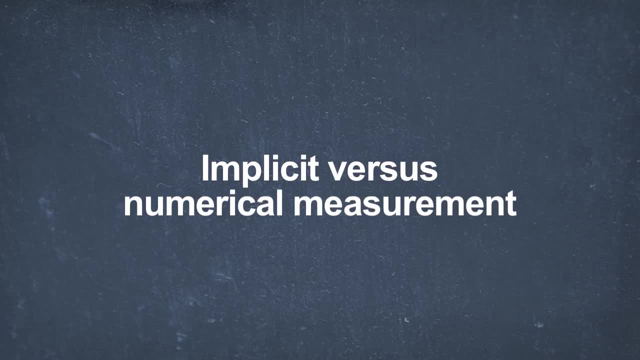 What we're talking about is the idea of a continuum of more or less that you can directly apprehend, directly perceive within a given attribute. In the process of grasping such a continuum, you're grasping the place within it of any given unit. 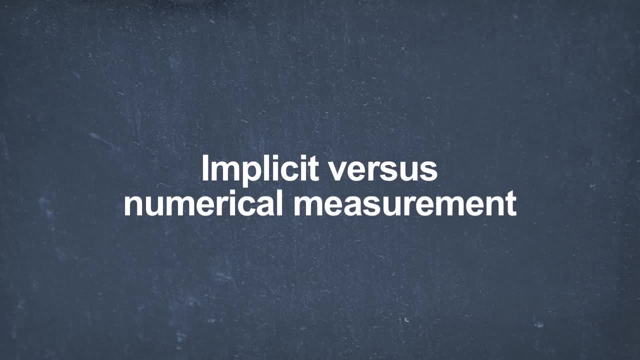 For instance, if it's length you see bigger, smaller, very small. You can pick any one and you see, in the act of grasping, where it is on the continuum: This is more and this is less. In that way, without words and without numbers, you can relate all of the instances of length. 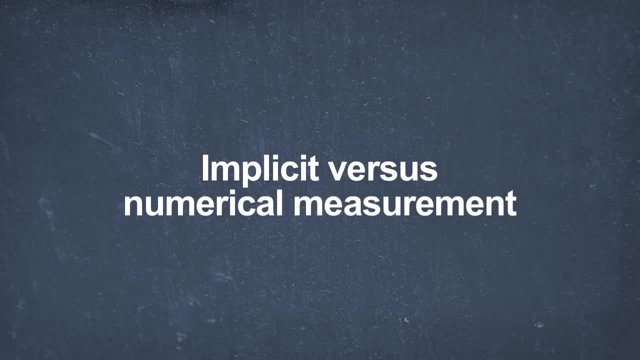 to any one of them, because you see all of them on a continuum. For the purpose of concept formation, it doesn't make any difference which one is your unit that you relate them to. You can form length out of ten lengths that you perceive by taking any one as the unit. 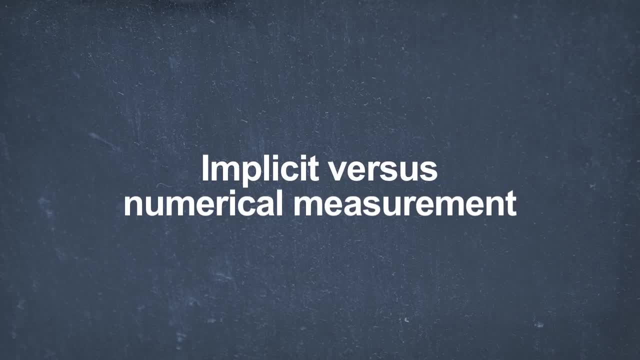 That's the point. The whole point is simply to grasp that they are commensurable, that all of them go back to some one unit, So it doesn't make any difference at all which unit it is, as long as you can perceive it. 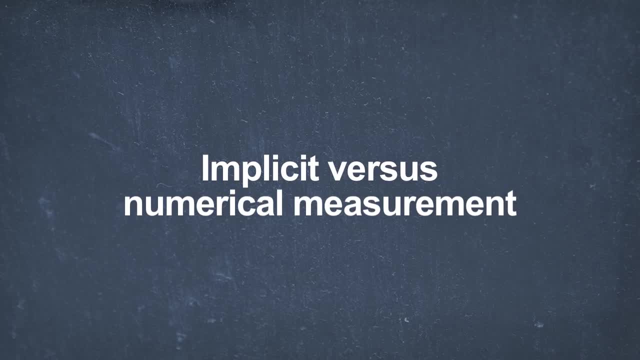 So if you see a spectrum, all you have to do is choose any one. Whatever happens to strike your attention, and your mind grasps that all the others are relatable to it. As I summarized that, any perceived instance can serve as the standard in the process of 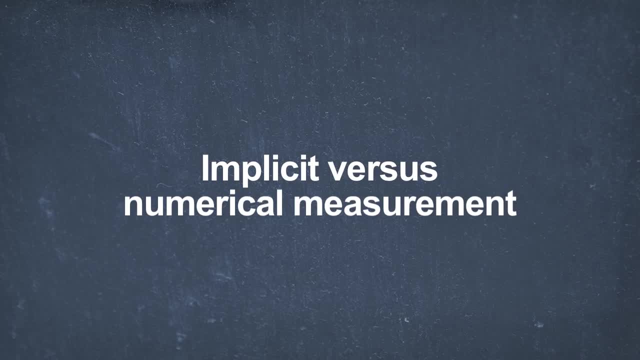 concept formation. Any perceived unit of the future concept can serve as the unit of measurement, So that in numerical measurement you have to choose a unit consciously, you have to define it and then you have to relate it to the rest quantitatively. 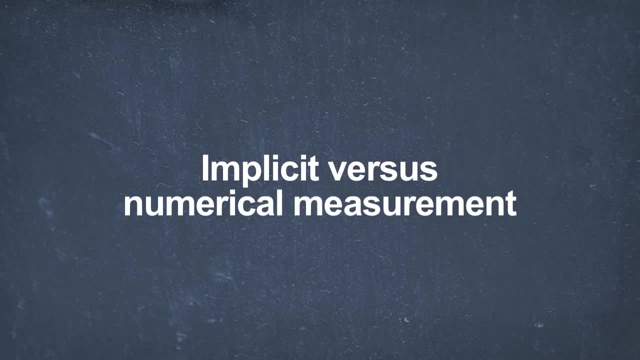 You have to discover techniques by which you can establish the precise quantitative relationship In concept formation. to put it crudely, you don't have to know what you're doing. You don't have to know that you're taking a unit. You don't have to know that you're taking a unit. 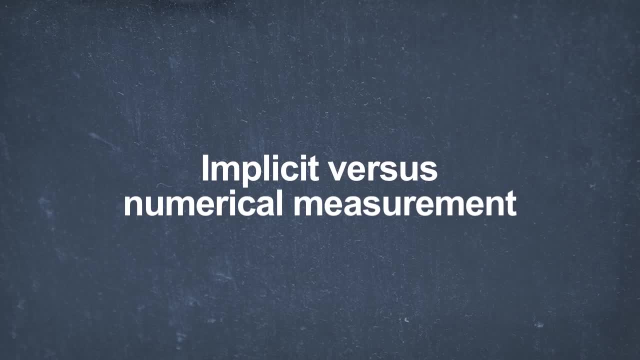 You don't have to make a point of relating that unit to all the other instances because in the mind's very grasp of more or less that continuum within a given attribute, it grasps that all of them are relatable to any one of them quantitatively, that the variation 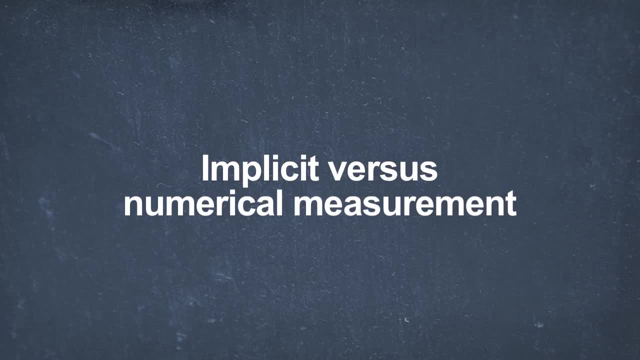 is simply how much, And that is all it has to know for concept formation. It doesn't have to know specific measurements, because the whole point is to ignore specific measurements And integrate into a concept, Into a new unit. Now that either answers the question decisively or leaves you in a hopeless quandary of what? 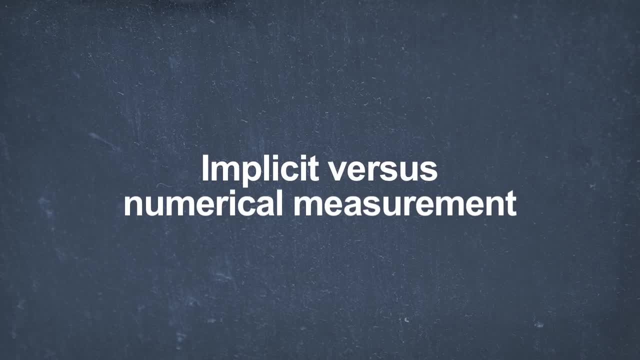 am I talking about. But if you're in that, let me make it worse for a minute. Oh no, I want to first just point out to you on 129 here. I think it's a good summary, if you get my distinction. 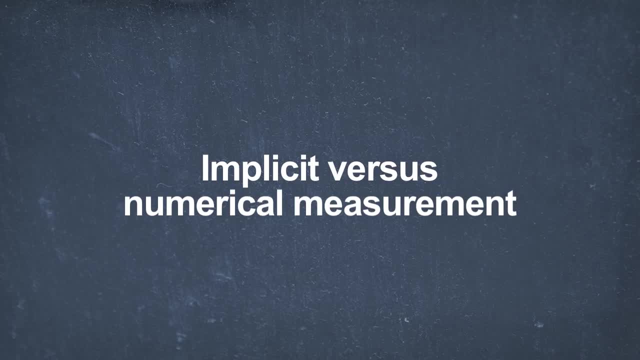 A form of measurement makes concept formation possible. That is what form of measurement Implicit measurement, The grasping of a quantitative continuum and thus of commensurability to a unit. So a form of measurement makes concept formation possible, And concepts in term- I'm on 129, make numerical measurement possible. 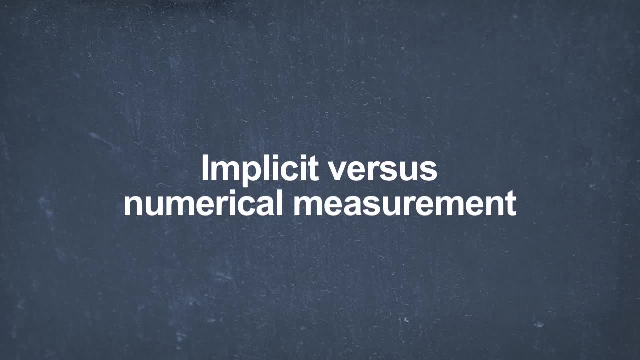 Once we have concepts, then we can form concepts of numbers. we can acquire the knowledge of how to perform measurements consciously, and then we can gauge in numerical measurement, in mathematics. So each in a different form makes the other possible. They're interdependent in that way, and that reflects the fundamental fact about human. 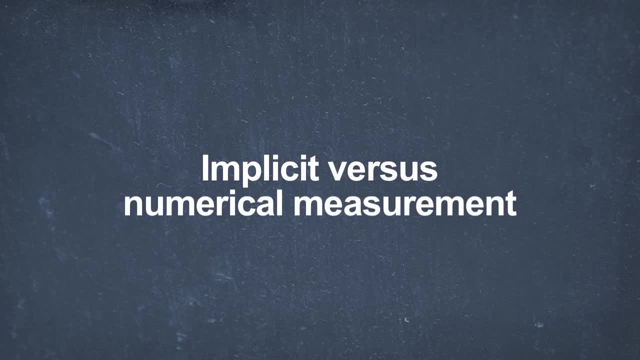 cognition, that the essence of those two processes- measurement and concept formation- the perspective that makes each of them possible is the same, and that is the quantitative reduction to a unit. Now you'll have to really get at home with this no-one presentation. well, do you have? 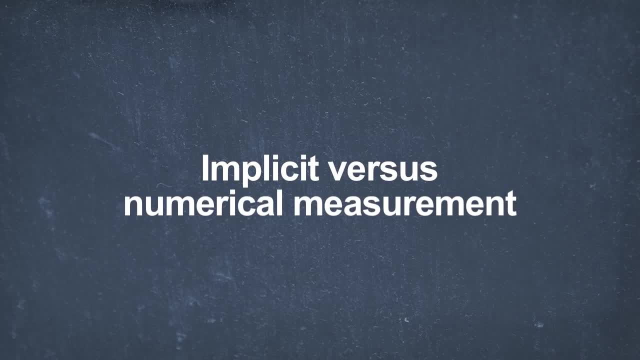 a question right here. I'm not quite finished. Yeah, Aren't you really describing the process of discovering similarity? Well, yes, I'm describing, he says. am I describing the process of discovering similarity? I am Ayn Rand, rather, because this is entirely her theory- is describing what is the well. 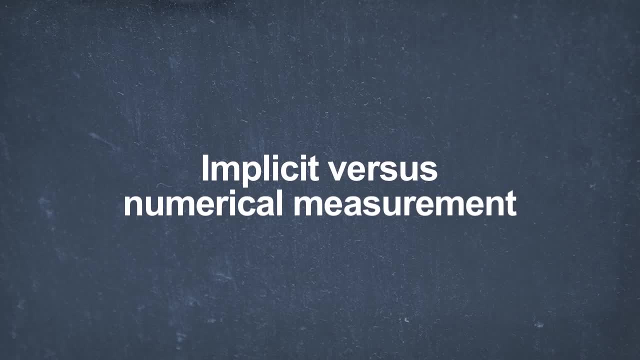 I'm not quite finished. I'm not quite finished. Well, here we are. What do you think of similarity? Well, the reason is the way I see it, similarity is the actual underlying mechanics of grasping similarity. When you grasp similarity as grown-ups, as philosophers, we simply look out and we say: 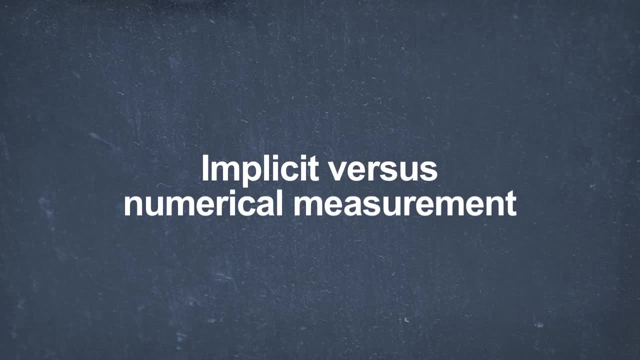 this is similar to this, That's it. But similarity itself is simply a description, That's just an identification of things. Similarity means identical in certain respects and different in others, The same in some and different in others, and what was never answered before in philosophy. 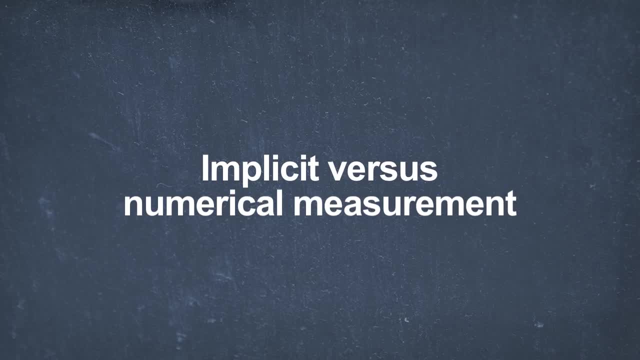 is: what is the same. What is your mind actually doing when it grasps similarities? The crucial importance of this is: if you don't have an answer to that, you say: well, I don't know. They're like each other. That's an irreducible primer. 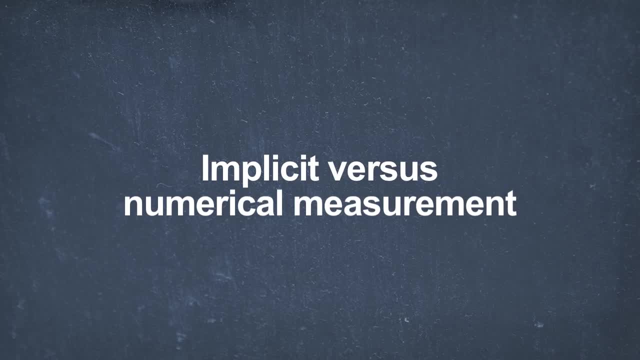 Well then, of course, they will lead you down this slippery slope that apes are like people and the next type of animal is like the other. If it's just irreducible and it strikes you, it's like it or it isn't. 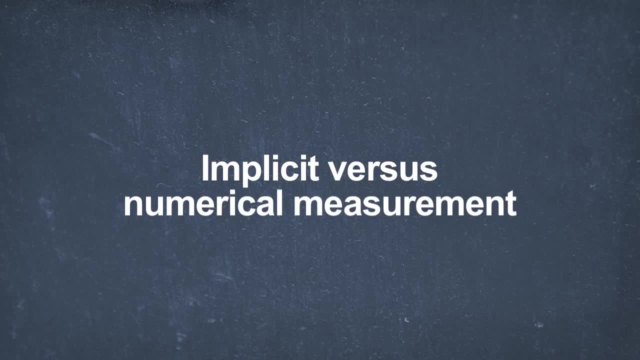 With no further definition, you have no basis of what is your justification in reality? what is the relationship to actual reality? So it's true that on the conscious level, you don't know anything about grasping a unit, having all the concretes be commensurable. 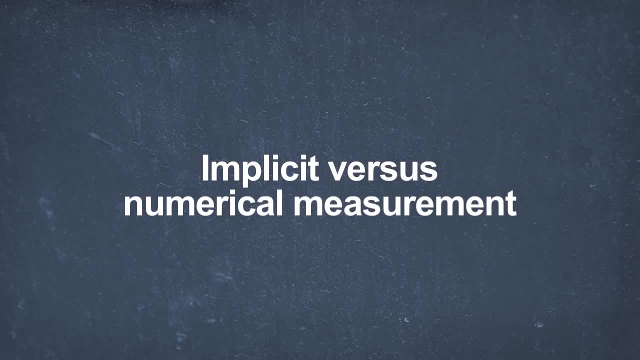 having them differ only in measurement. but it's that identification that permits the objective validation of the faculty. and of course, as we'll see later, without that you wouldn't know how to use concepts properly, Because it's only knowing how they really are formed. 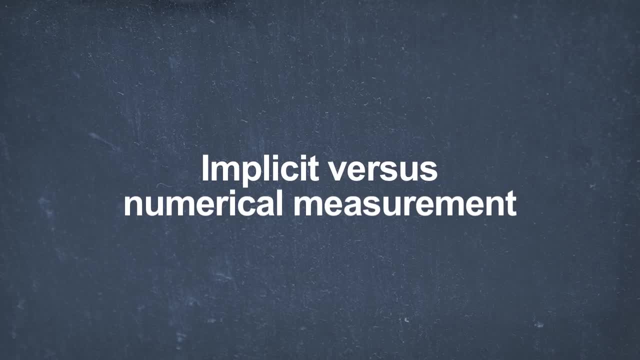 that leads us to such ideas as objectivity versus intrinsicism and subjectivism, and therefore logic and all the things that are within your conscious control. So if you rested only on, I perceive similarity, but I can't do any more, it's just a primary. 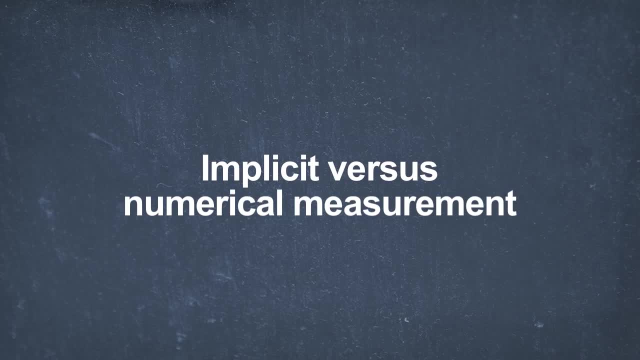 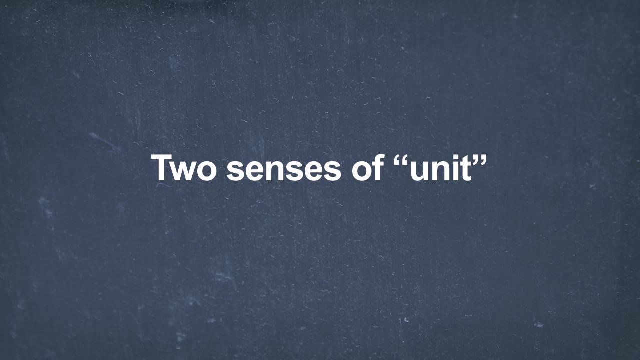 you would be stopped dead both polemically and epistemologically. So it really is crucial to get underneath the perceptual experience, and that's what she's trying to do Now. I wanted to make one clarification here. There are certain people who are bothered. 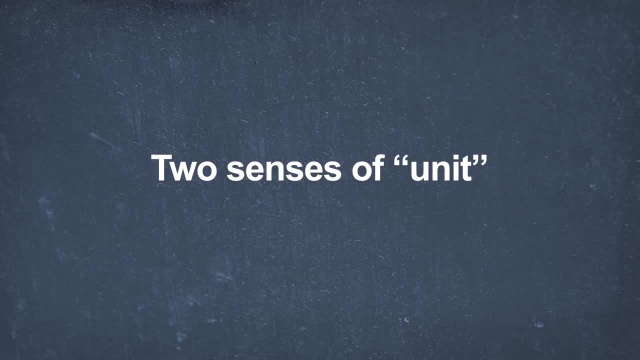 by the word unit, which is and is not used in two senses, And that is a perennial plague to people who are learning this theory. So let me point out that there is two senses and then quickly show you that it's the same sense. 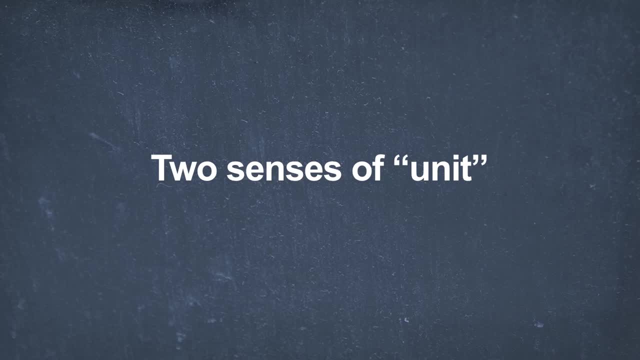 But there is two senses. first, because if you don't get this, you'll swim forever. When we say every man is a unit in relation to the concept man, or every banana is a unit in relation to the concept banana, we're using unit there. 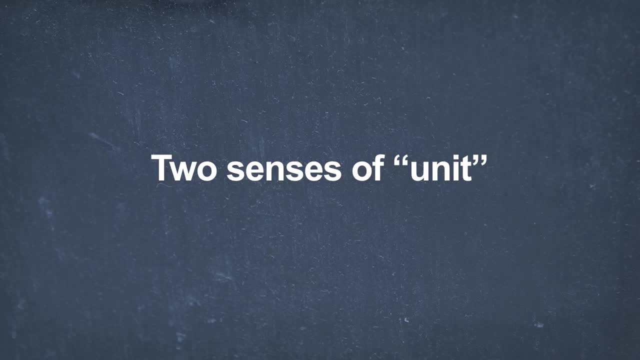 in the sense of Ayn Rand's primary definition, An existence considered as a member of a group of two or more similar members. The existence considered as a member of two or more members. it as a member of a group of two or more similars And, in that sense, every instance of a concept. 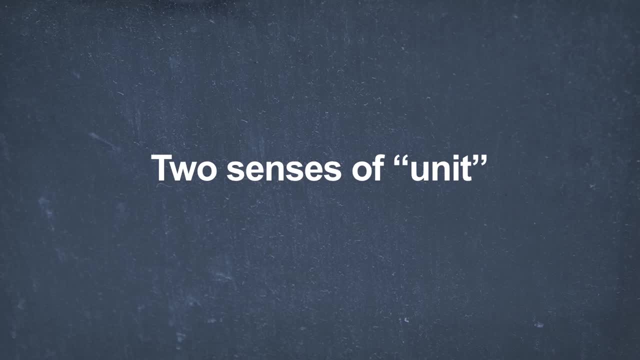 she describes as a unit, because you look at it as one of a unit of this total related to them by their similarity. Now we also use the word unit in the sense of unit of measurement. A unit of measurement is a unit used to measure something. It's still a unit, but it's a unit. 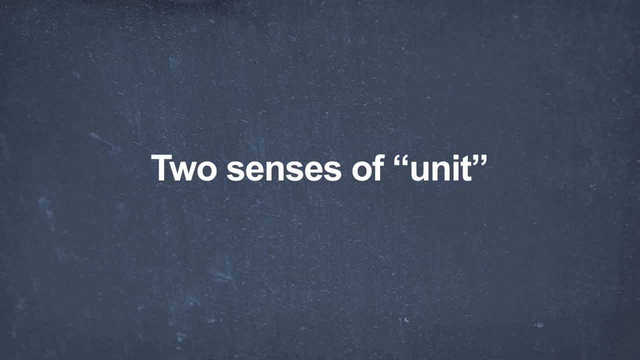 which has a specific function. For instance, an inch is a unit. It's one length out of all the endless number of lengths there are, Just as one man is one out of all the possible men there are. And in that sense, an inch is a unit of the concept length, Just as man. is a unit. In other word, at least ten of Us triples our entire different universe. Just as Man equals Man equals the whole thing. Furthermore, Unit of Me equals the itself. Just in the blink of an eye There. why'd you think of this? The line when we could rely upon this is We talk about. 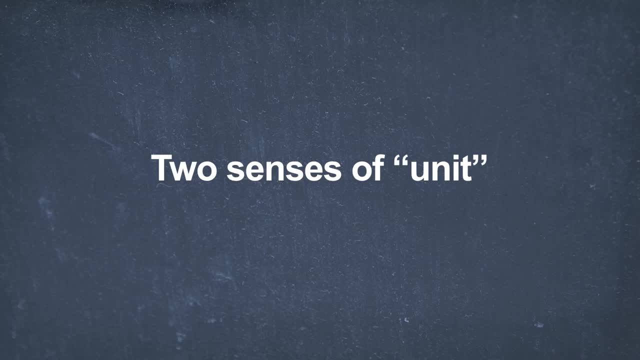 is a unit of the concept man, But the difference is because length is an attribute, we can take one of its units to measure it. So the same thing which is a unit of the concept is also a unit of measuring the concept, or measuring the instances. On the other hand, when you deal with things which 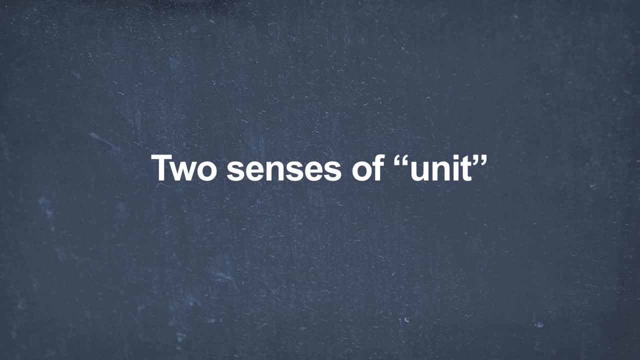 are not concepts of attributes like man. you cannot measure them by individual men. You can't take a little man and carry him around and measure all men. So a man is not a unit of measurement. To measure man you have to strip man into attributes and then you take a unit. 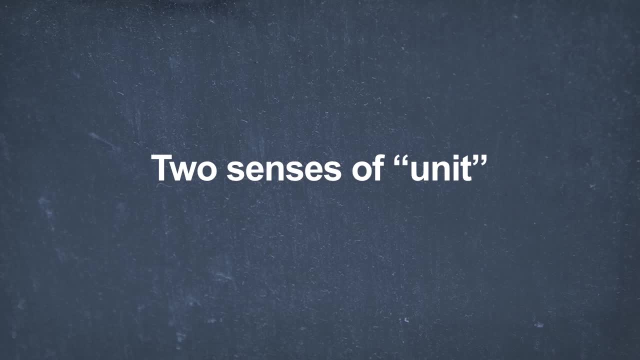 within each attribute, which serves as the unit of measurement for that attribute. So I get this question all the time. If you need units to measure, and every concrete is a unit, doesn't it mean that you measure by each concrete. It just simply wipes the mind out just to hold. 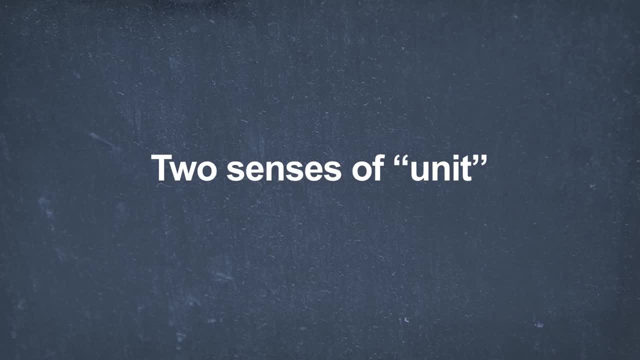 that, So I don't know what to do further. Perhaps I'll just on that point. Ayn Rand herself discusses this on the second edition in the workshop This. I was referring to pages 184 and 188, but just to read the key points here, I think I've 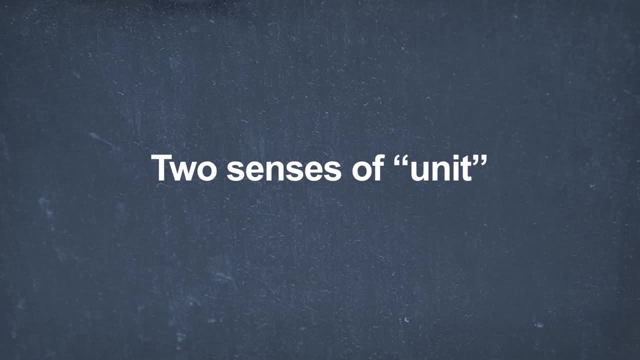 made it clear. You see, it's two different senses. Not every unit is a unit of measurement, but it's not an equivocation, It's not an accident, because the unit of measurement is simply a unit. It's the same perspective, but it's a unit put in the service of measurement. 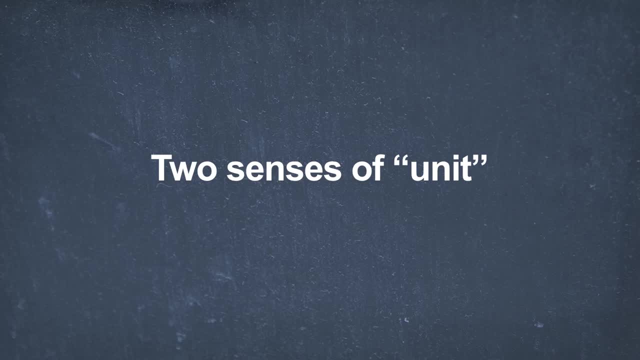 Is that unclear? It's unclear. It's clear To you. it's clear because I saw you nodding- Yes, Can't hear you. I was going to ask if something that I've done on this was the same thing. quite the same, as I thought that concepts of entities can be treated numerically. 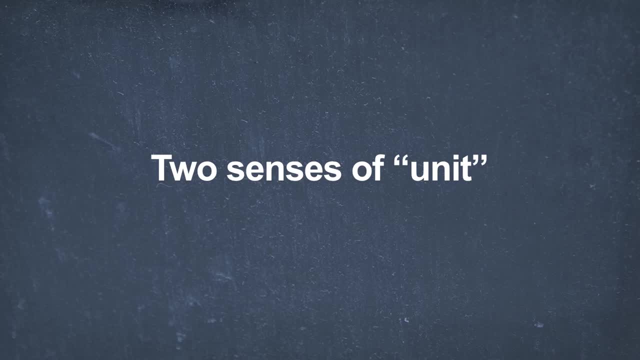 only as integers, In other words counting distances of the entities, as opposed to concepts of, say, things that do represent attributes. measures can be represented by fractions. You know not in Well, I want to. I appreciate your attempt at originality, but I want to stay away. 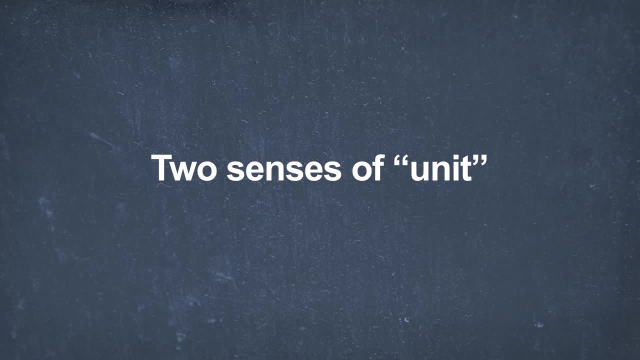 from it, because parallels here would require a tremendous detailed discussion to try to relate attributes to fractions and entities to integers. I wouldn't dream of such a possibility because they're not the same and you would have to specify in what sense exactly you mean the analogy. 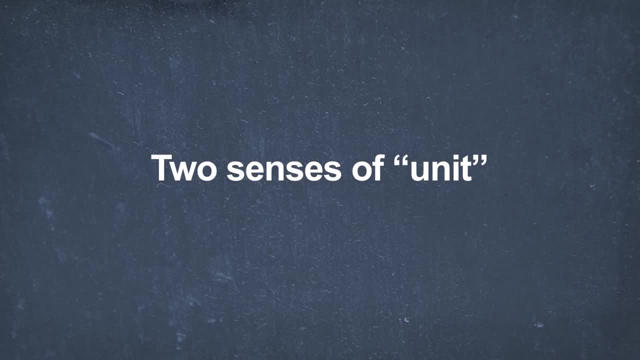 and how would you then apply it to actions, for instance, and so on? And then, when we did it all, the question whether it would be illuminating is another question. so I'd rather not. let's just stay with understanding what Ayn Rand said. Someday somebody will elaborate a whole. 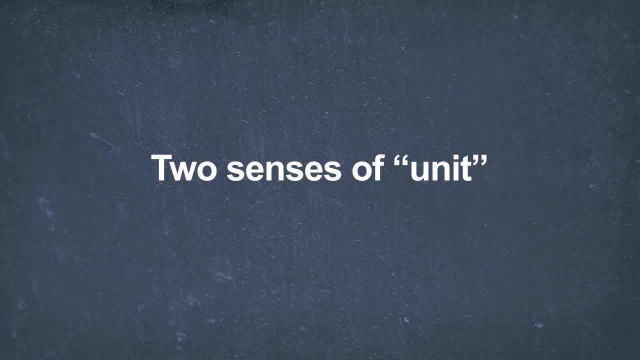 theory and maybe something on the order of what you're suggesting would be conceivable, but I wouldn't try it now. I want to just read her passage on unit: Every concrete is a unit when regarded as a separate member of a group of two or 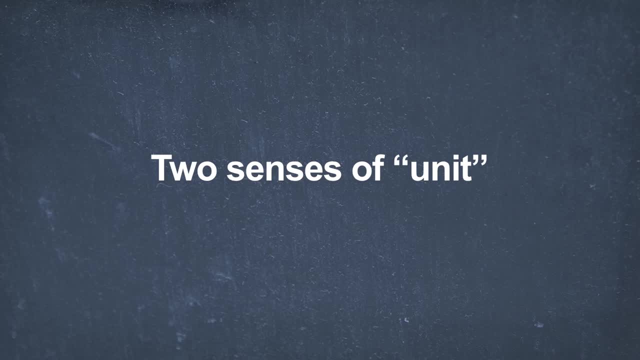 more similar concretes. A unit means a group of two or more similar concreteness. Every unit is a semiton. The unit is a concrete, an existence, regarded in a certain manner, regarded in a certain relationship. Every concrete is a unit when it is so regarded. 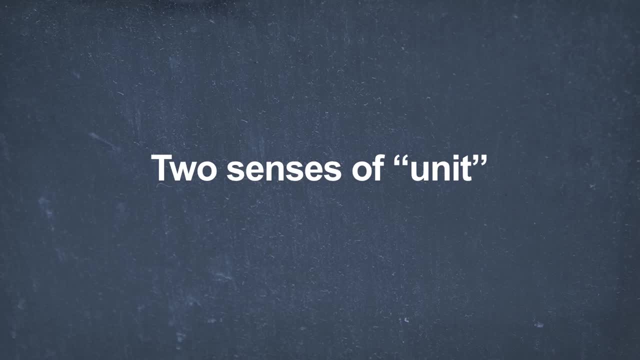 But that doesn't mean that every concrete can serve as a standard of measurement, because unit here has two different meanings. A unit selected as a standard of measurement, for example the inch, has to be a given quantity of a given attribute, not of an entity. 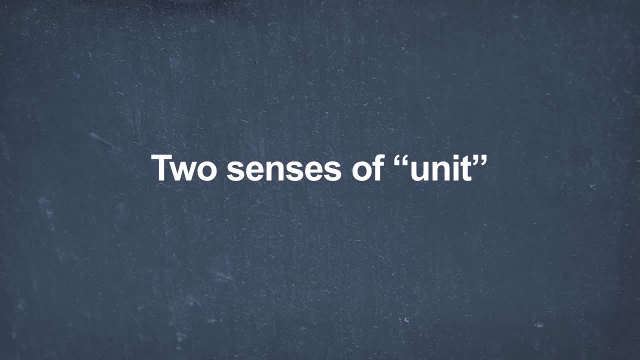 So you see, in a sense there's two different meanings, but in a sense it still comes back to. she goes on in page 188,. it isn't arbitrary or purely linguistic in discussing measurement that I use such a term as unit. The mental relationship involved is the same as in regarding concretes as units. when we 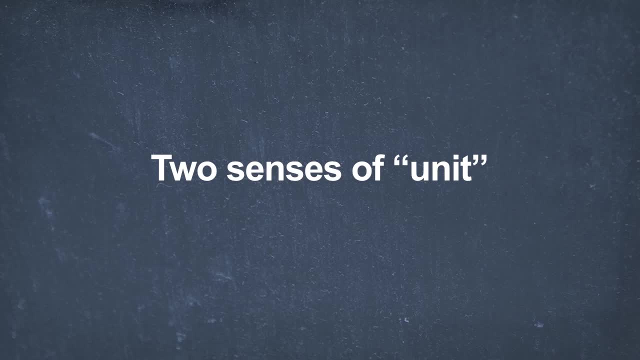 form, a concept, The relationship, the aspect from which we regard it is the same. So You get that. I thought that might clarify something. Now I'll just say a word in conclusion of this preliminary survey about the profound importance of this theory. 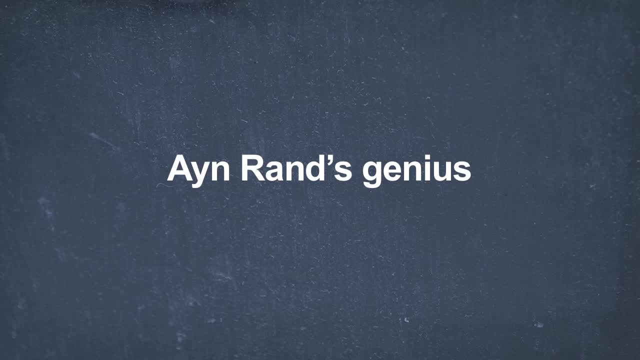 To me Ayn Rand's genius is captured. I discussed it on page 134 and 5.. It's a parallel or not parallel, because it's literal application to algebra that concepts are to their instances, as algebraic symbols are to. numbers is the single most. 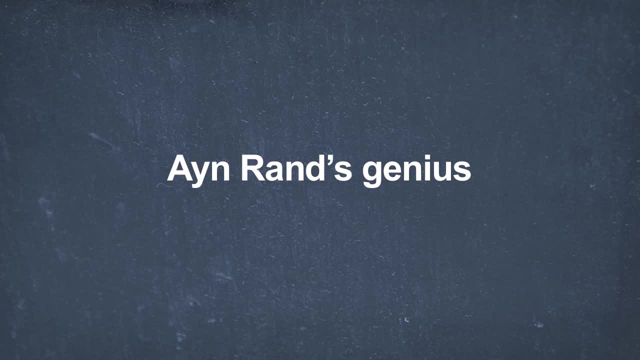 brilliant paragraph, I would say, of her life output, I mean as a way of taking a problem at the root of all philosophy, And And She's making a presentation of a whole complex theory in terms of a known, obvious, simple 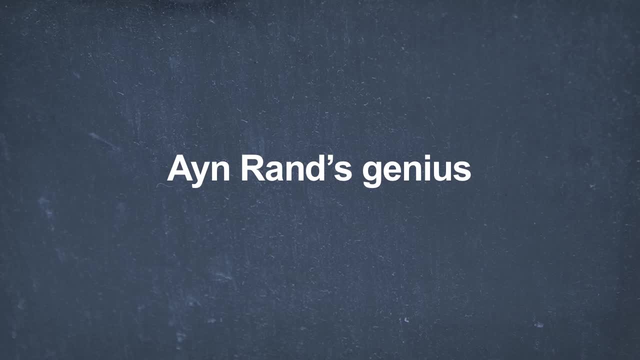 relationship like A to all the content and the numbers that go into the variable, And to put it together in one paragraph that is so luminous that after you read it you can't imagine that it wasn't known. That is the mark of genius. 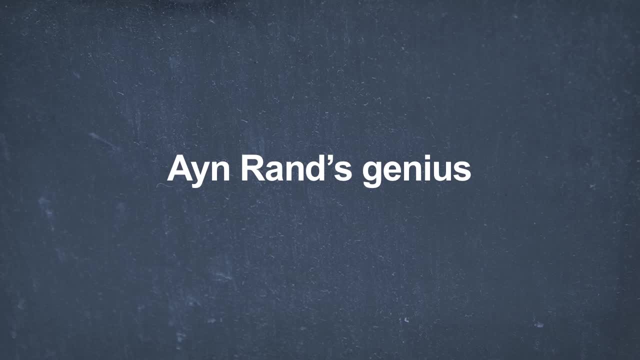 And then she has the polemical paragraph there. I'm sorry. Let those who attempt to invalidate concepts by declaring that they cannot find madness in men try to invalidate algebra by declaring that they cannot find anus in 5 or in 5 million. 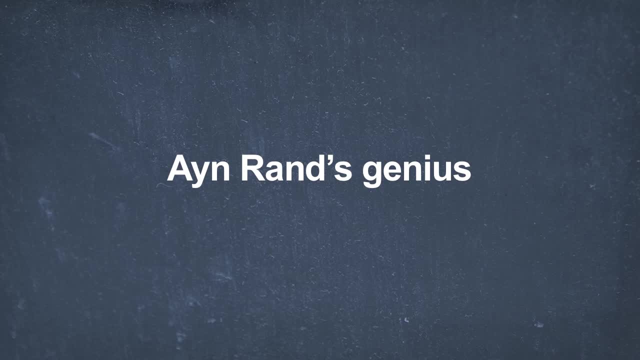 And it's the same thing. A, there is any number, but the measurement is omitted, not how much. Therefore, it stands for any number And nobody would say. I've gazed at 5,, 5 million, 13 million and I just can't find anus in. 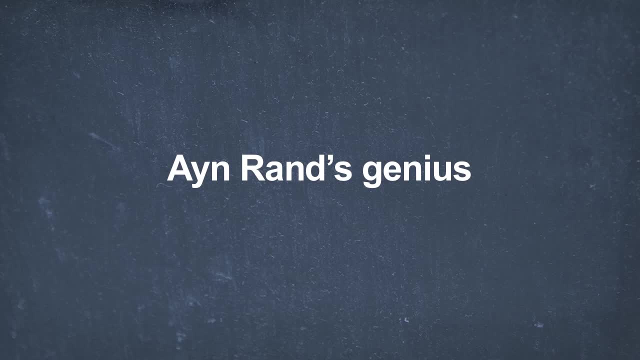 You would know, it's a device to be able to focus on all numbers. It doesn't come from God and it's not arbitrary, And it's a device of integrating them and being able to work on a higher level without having to focus on any particular number. 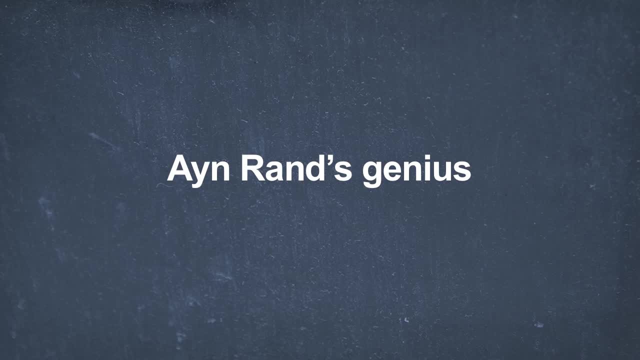 nevertheless applying to all numbers. And there is no problem of algebra, And yet there's a problem of concepts, and it's exactly the same phenomenon. Table is to table like A is to 5 and 10.. And that, to me, is her single greatest act of genius in her entire life. 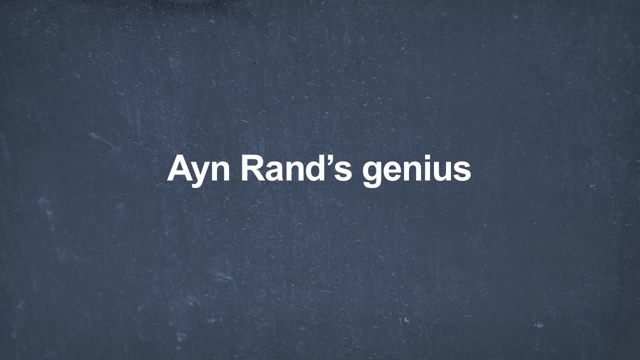 even more than her morality or her politics or any other thought of hers, because this really goes to the very, very foundations of human life, of human thought, And it is such a fabulous integration that I think someone should go down in history simply for that idea, even if she didn't write a book on it. 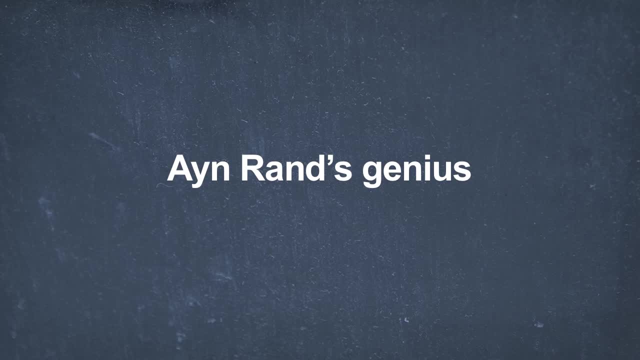 let alone an entire philosophy, And then the artistic implementation and projection of that philosophy. So, as you gather, I'm very enthusiastic about that paragraph. Now I myself, if I say so, made a good observation about her achievement here in these follow-up paragraphs. 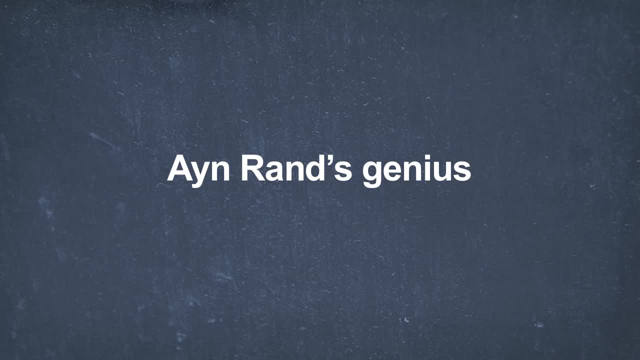 That is the difference between objectivism's attitude toward mathematicians or mathematics and the standard attitude. Now, philosophers, As I say here, from Pythagoras in the ancient world on up, have always venerated mathematicians. Mathematics, somehow is the key to everything. 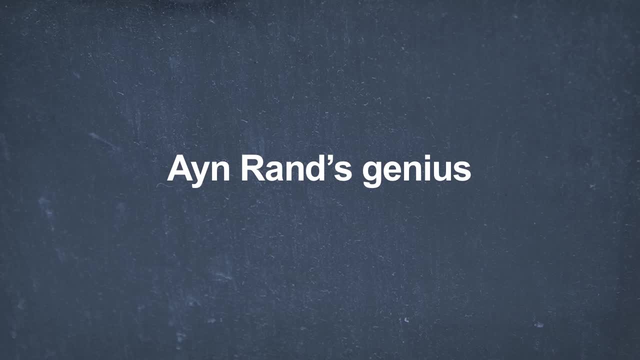 From the very first that Pythagoras said: all things are numbered, which was, you know, a crude, metaphysical, primitive way of trying to get at the idea, which was valid, that somehow numbers are everywhere, that mathematics is everywhere. 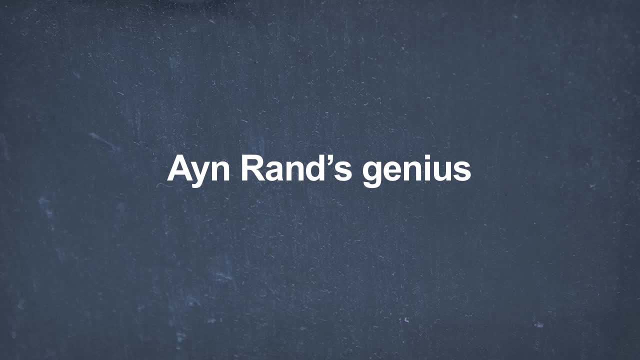 that that is the key to the universe And of course, that thought has been held, in different forms, more or less valid. But there's something unique about mathematics. But what rationalists have done is take the formal deductive structure of mathematics. 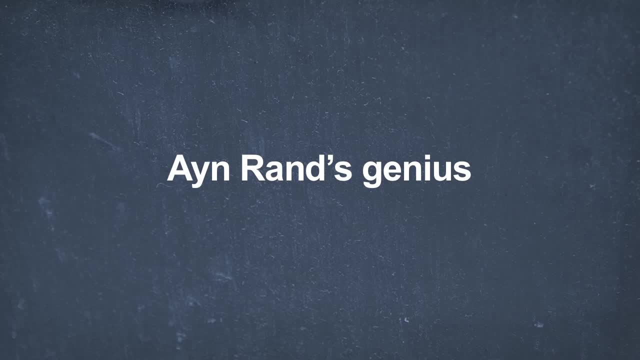 as the key to its importance, Starting with an axiom and saying if this then this, if this then this, if this then this, And therefore they have turned what should be a profound illumination into grist grist for the rationalist mill of constructing floating systems. 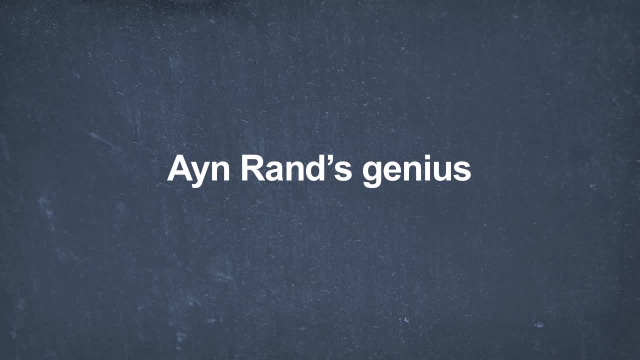 But what is Ayn Rand's uniqueness is to say: you're right to focus on mathematics. but what mathematics gives you, if you approach it properly, is not how to churn out deductive consequences from premises. What is really crucial is how to go from observed and bring the whole rest of the universe. 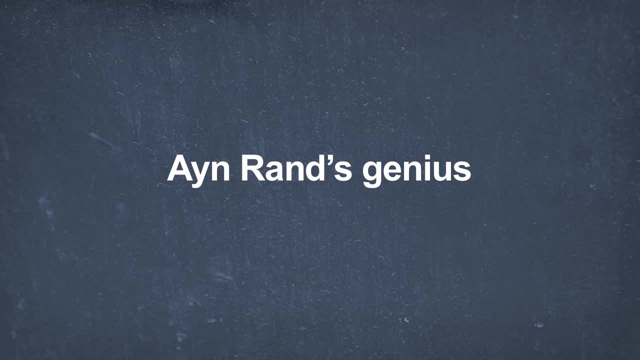 into relation to what you observed through measurement. Now the matter has been the science of measurement and, from that point of view, mathematics. for her, this is my formulation, but it's a good one, I think. But mathematics reveals, it's not the mechanics of deduction. 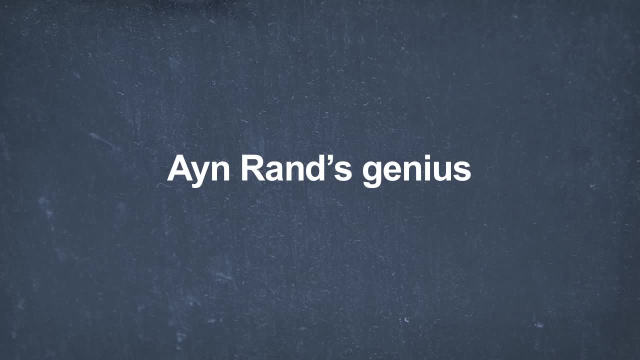 but of induction, And that is, you know, Ayn Rand's genius. that would simply have occurred to anyone who wasn't aware of her approach. Now we just flip over quickly to to the end, which I believe is 163.. 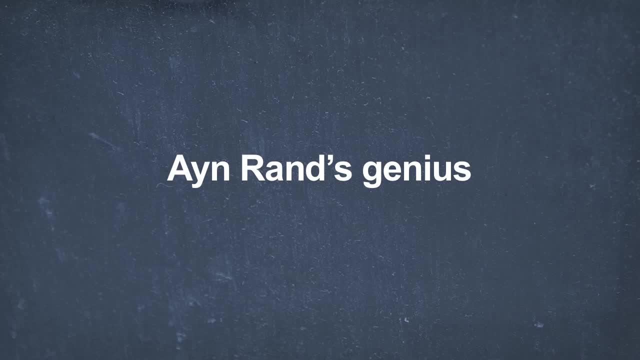 I believe that I mentioned there Ayn Rand's unfinished work. I think that what she would have done if she hadn't lived long enough is use mathematics, higher mathematics, to solve the problem of induction. That is, I think, the direction that her thought was going in. 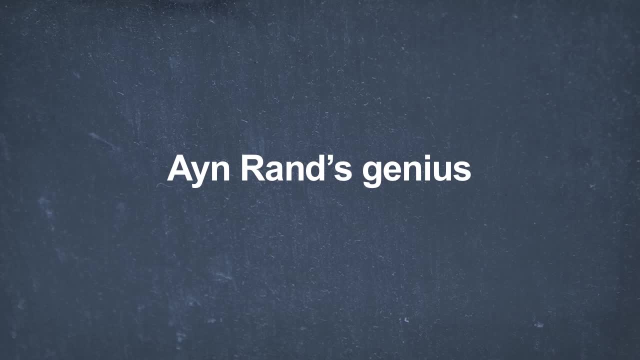 Because she knew that there were many more similarities between concepts and mathematics than the one she had mentioned, And in fact, she was undergoing the systematic study of higher mathematics at the time that she died, because she felt that she had to learn as much as she could about higher mathematics. 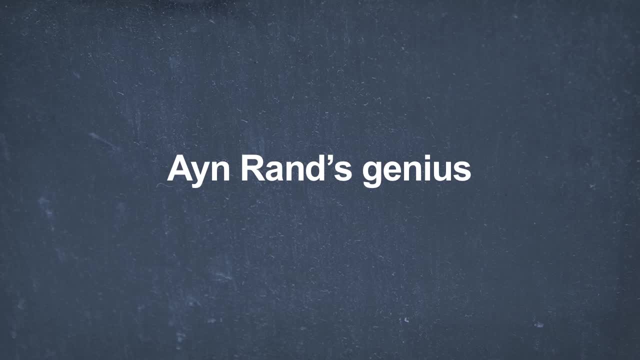 specifically from an epistemological point of view, of what similarities did she see at each step- positive and negative, numbers and equations and so on- and where did she see similarities to what ordinary conceptual development? And she was convinced that there was a great deal more to connect. 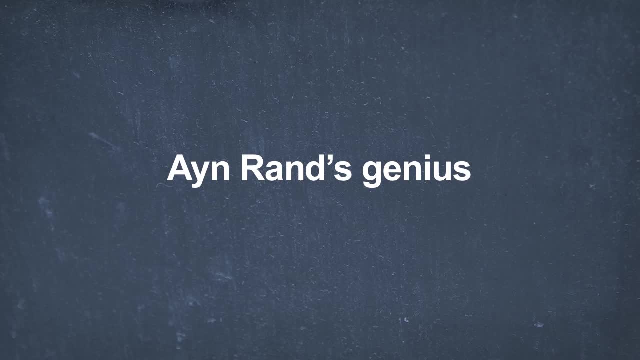 than what she had done in this book, And she also, by the way, was extremely interested, as they say here, in neurology, Not that she knew much about it, but just in the idea that there are things to be learned about the brain and the nervous system. 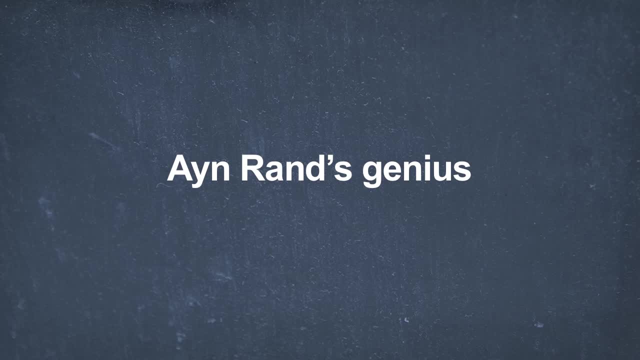 which is, after all, the organ of our mind. that would also tie into how the mind works, And of course this reflects her commitment to the mind-body integration. She was not content with the theory of epistemology that simply said: I have nothing to do with the brain. 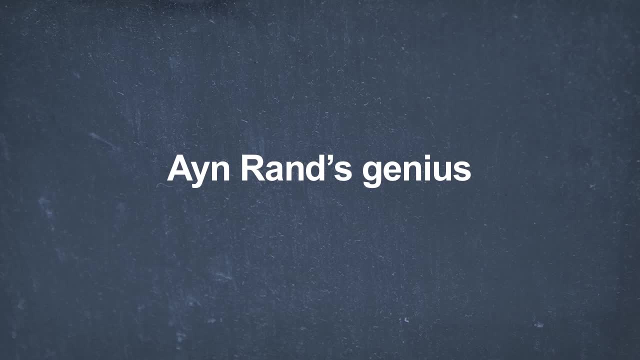 that's physical. I'm only concerned with the mind. She wanted the ultimate integration And I believe that this is as far as I can make out. the direction of the next genius, whenever he's born, has to follow, to build on her leads. 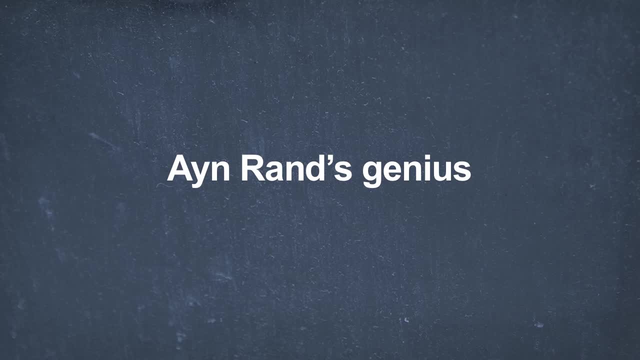 I do not believe that this is necessary in order to know what she has done, And I think we can validate what she did on the basis of what we ourselves know. But I do strongly believe that the human race continues and if another genius on her level or Aristotle's- 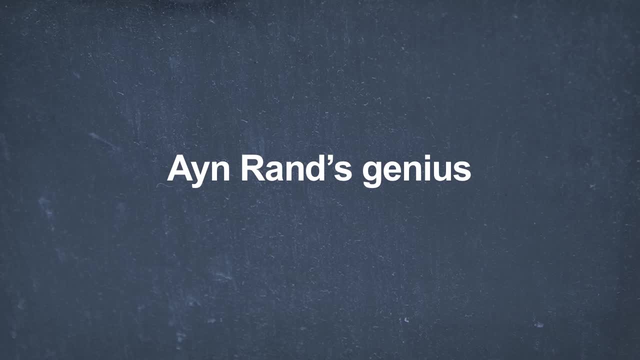 is someday born. at that point he will look back on what we're saying now on concept formation and mathematics as just the beginning of a much, much more complex integration between mathematics and concept formation, which will go all the way through the higher branches. 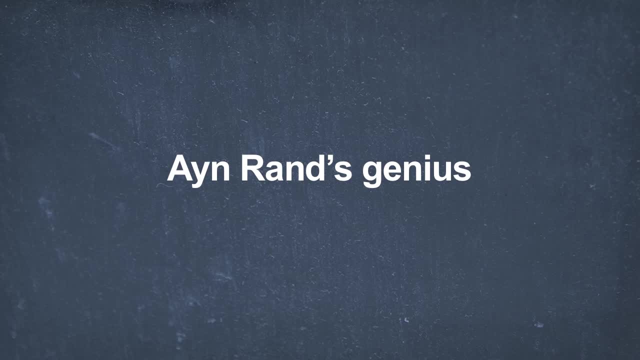 of mathematics and connect to all the different aspects of concept formation and, in the process, solve the problem of induction and of theory formation and of how you know when you're entitled to hypothesize a certain theory and when you have enough evidence to say. 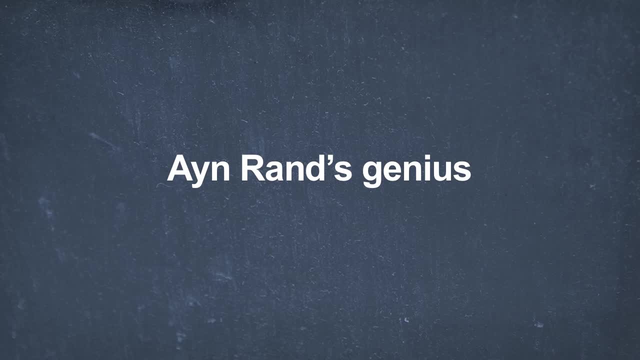 it's the only possibility. I think all of that, and I think that's the only way that we can do that. I think that's the only way that we can do that. I think that's the only way that we can do that. I think that's the only way. 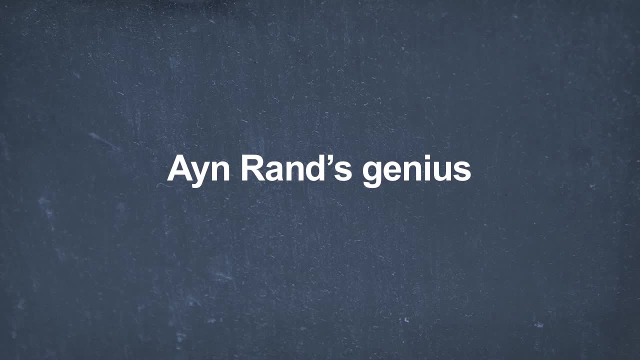 that is not now done will be done by following this path, And so I think it's a tremendously important lead, And unfortunately I can't do it. If you can do it, more power to you, But what we have to concentrate on here is that. 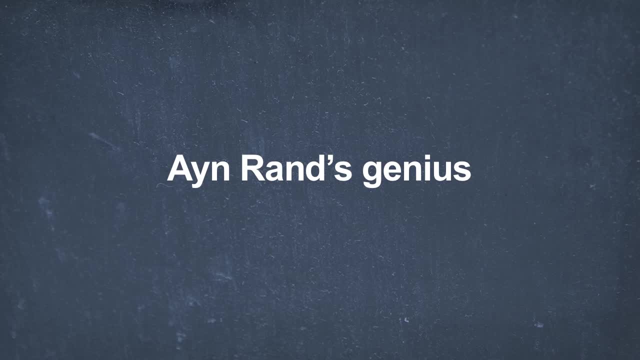 what we have got and understand that, and someday someone will give you the rest of this class will give not you, but your 50th and your 50th generation grandchildren. However, since knowledge is contextual, he'll do it only on the basis of what we establish now. 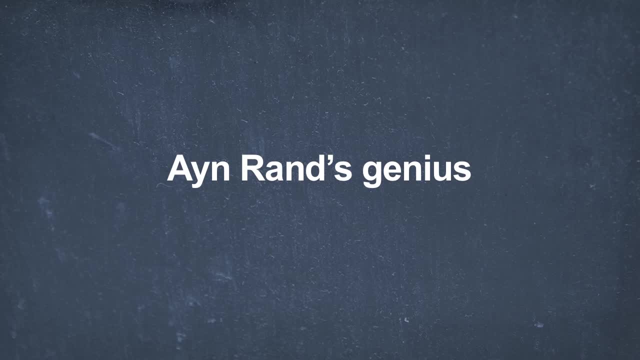 which you then have to pass on generation by generation until someone can take it further. So what we're doing is not to be sneezed at Now. does that bother or elate you that there's so much still left to do? Both, Why does it bother you? 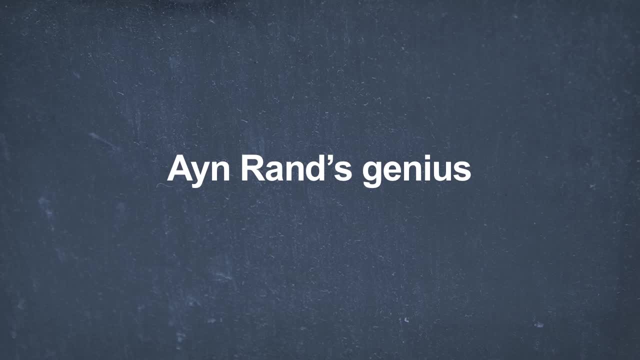 It doesn't jeopardize what we know. It simply means that what we know is a window on a huge field yet to be defined. So don't let it bother you. Or maybe it bothers you out of sheer curiosity. Several people have said to me: 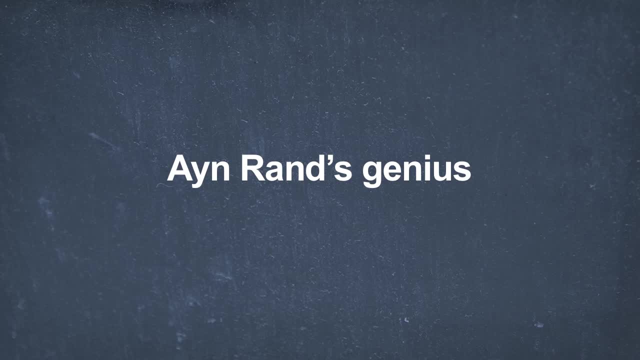 couldn't I make Orrin's scrawled notes on this development available? Well, someday I'll publish everything that she wrote, but believe me, it's likely that I won't deliver that book. the notes exactly for Galt's motor. 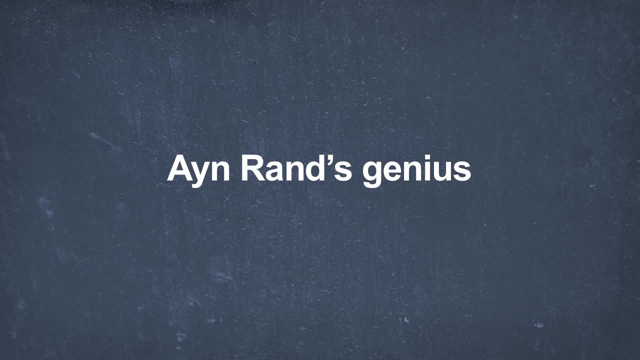 You have to be able to invent the motor on your own, to reconstruct it from the notes. If you don't already know where she's going, it won't get you there. I can certainly testify to that. a scrawled fragment And it just won't help you. 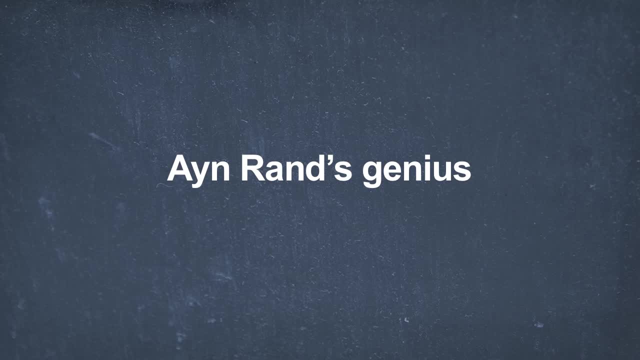 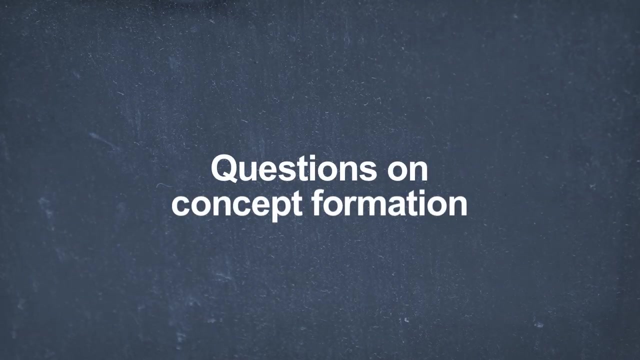 So let us, I guess, take our break here and then we'll have questions after the break. All right, just let me reiterate the preface to questions. I want them to be in terms that are of general interest to a broad, overall philosophic view. 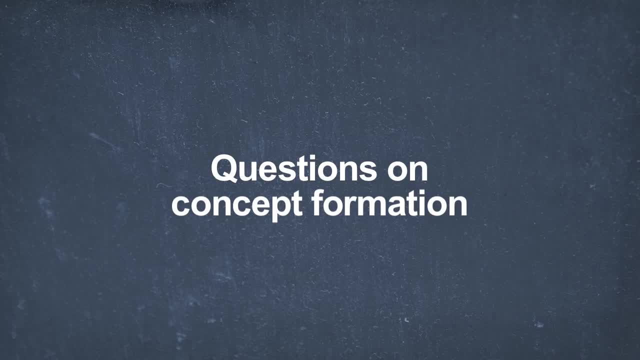 as I said at the beginning, Now various people in here are highly specialized and one gentleman very kindly put his question to me personally And said I don't think that this would come under a general interest, and it was highly specialized. 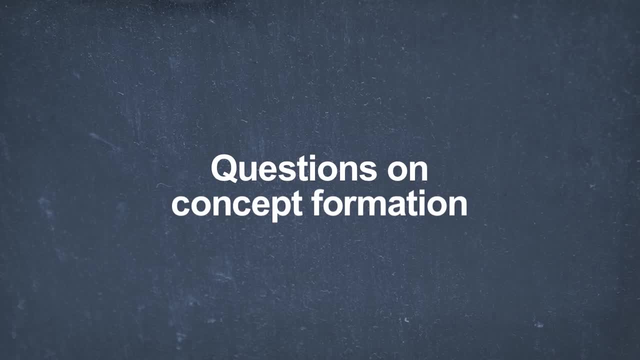 Now, whether I can answer it is a different question, But it's not appropriate in this forum because this topic is hard enough as it is, let alone a highly technical call. it could be back and forth. It would be of interest to a specialized scientist. 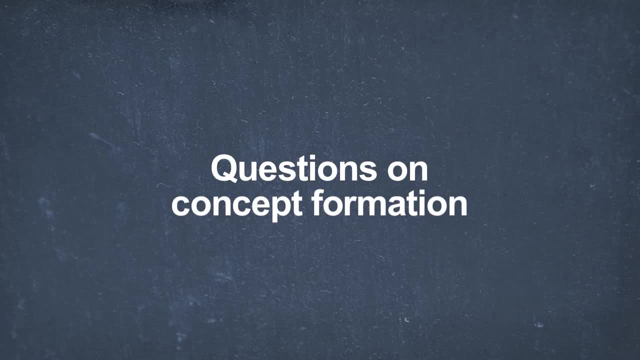 but not to just human beings living their lives. We're already beyond what you need for that, but I don't want to get off the deep end completely. Ray, I don't want to intimidate you, but I want to have this on call when I need it. 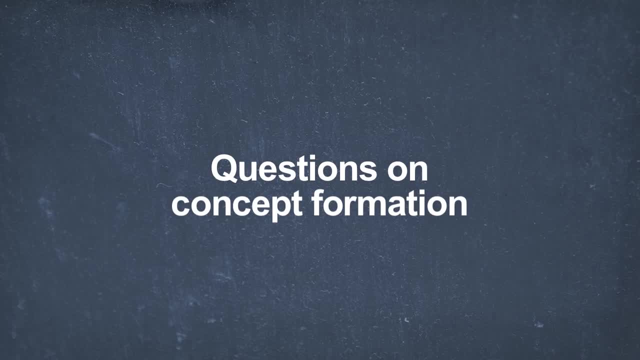 Yeah, Okay, 129.. Oh, we're in the first section. I thought You're going to the. I'll do it now, but then I want to start with the first section, 129,. yeah, Fourth paragraph, Yes. 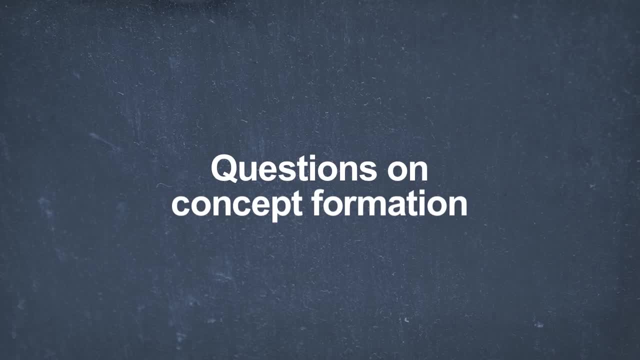 So far. so far we've been talking about integration. I didn't know how far back that went. I assumed that the section at the start of this section on 120.. And when you talk about there, Yes, by so far there. 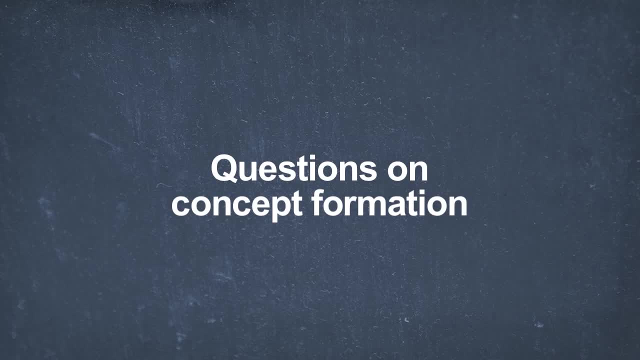 I mean up to this point in this section, Because- and the fact in the further editing I added the word primarily to that sentence- We have been primarily considering, we've measured it rather primarily in regard to integration, Because you cannot integrate without differentiating. 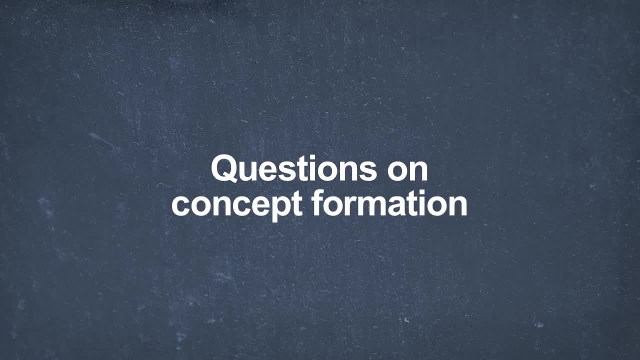 So you can't treat it as though integration- you know you differentiate- a group of people, a group of concretes, Then you go out to lunch and come back and now you're going to do the integration. It is one process. 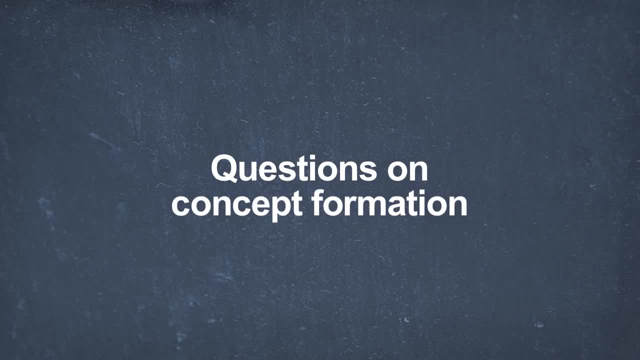 We can separate aspects of it, but if you just separated a group, went to lunch, the group would be gone. When you came back you'd have to start again. So it's just simply from the point of view of focus. What I focused on in the discussion was what's the same. 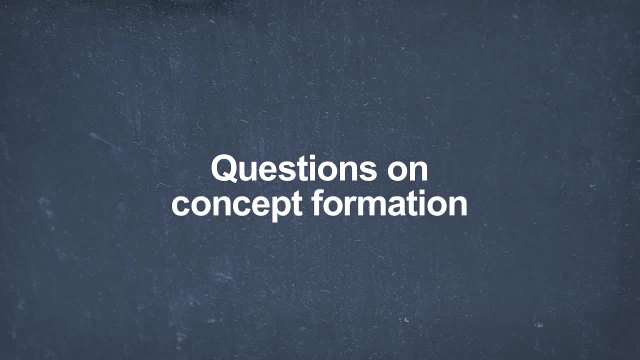 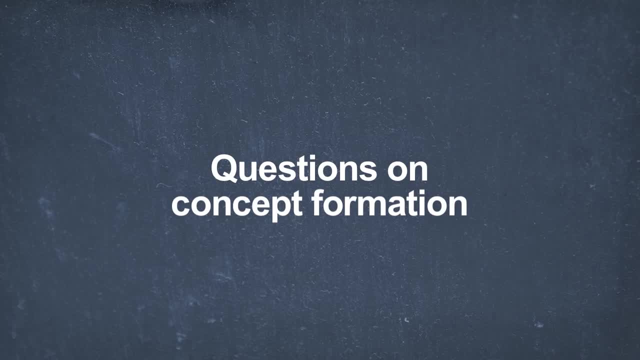 but that still leaves the question: how was I even able to separate this group out to begin with? And that's where the other side comes in. So why differentiate on page 124?? You just answered that with the prime arrow. Yes, that's why, when I reread that, 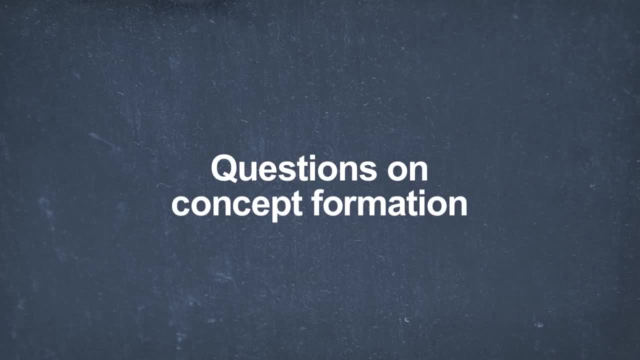 I thought to myself: it's too flat to it, tears, integration, too much away from differentiation. to say this is the omission of the word. primarily, there is a slight rationalistic touch. you see It's like: well, now I'm doing this. 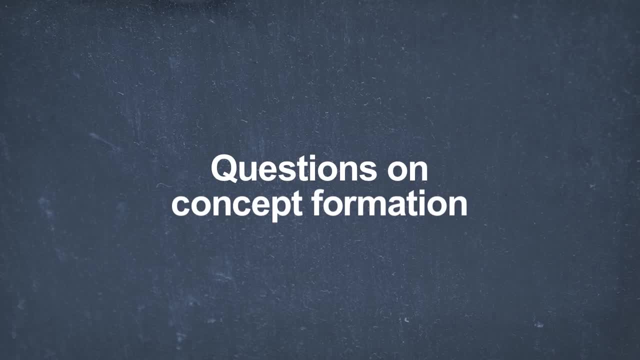 so that I'm wiping everything else out. And that's the kind of shading that you get only on the ninth editing. I hope you get them on the ninth, Who else? And now let's go back to the first sequence, which is where I'd like to start. 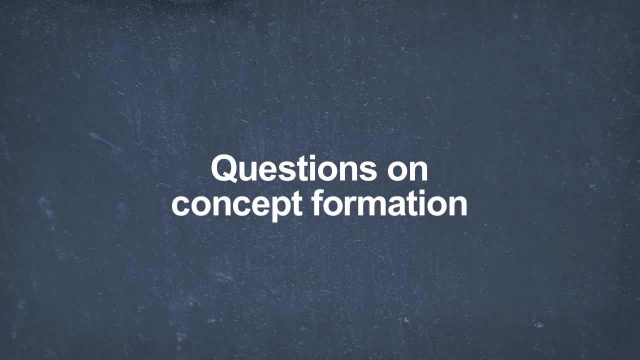 The description of the conscious processes: differentiation and integration. yes, Now my question is about what a concept consists of as a mental unit. I always thought that, as a mental unit, a concept consists of a group of similarities that are integrated. 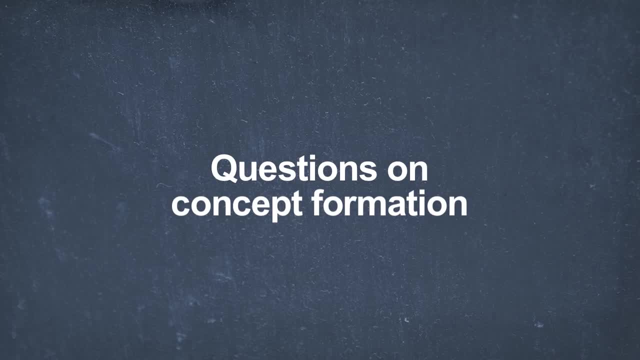 No, No, No. On page 116, you talk of them as being percepts that are integrated. Yes, And then on page 118, you talk of a concept that's consisting of a word and a conscious perspective. I take a conscious perspective to be. 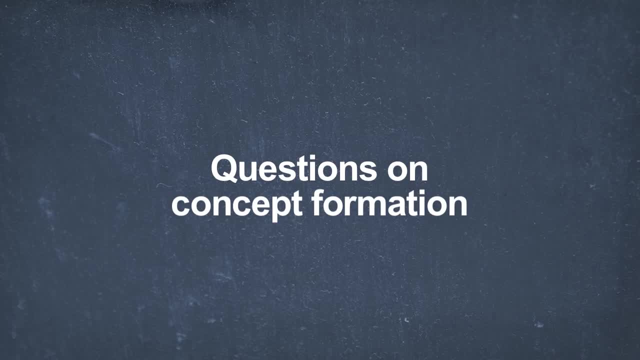 like a sort of a mental state, And so these look like- All those are correct, except what you said: It doesn't consist of a concept, does not consist of similarities. Now, let's all right, I get your idea. A concept is a complex state. 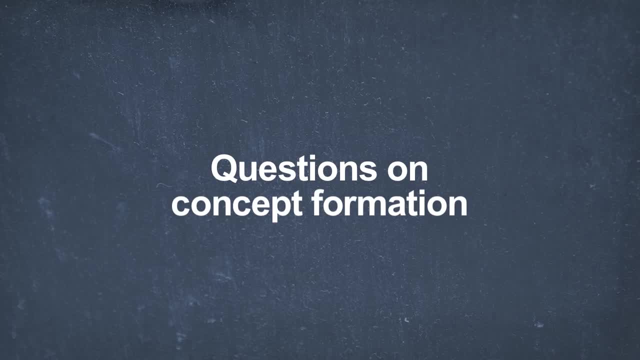 It's reached by a variety of processes. It has a relation to reality that we reached first by perception. So you can describe a concept in many different phrases, which are not contradictory, depending on your perspective. First and foremost, the essence of it is: a concept is: 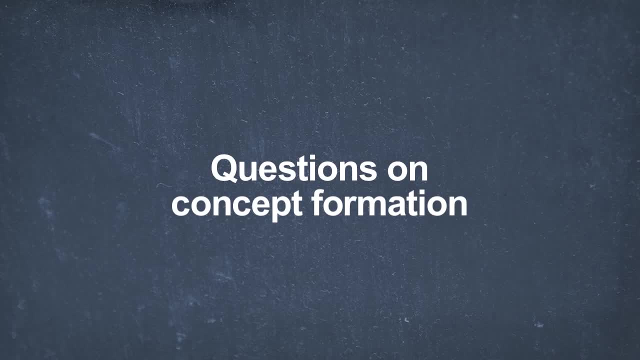 an integration of units. A unit is any existence viewed as a member of a group. A unit is any existence viewed as a member of a group. The unit, however, is not simply quote its similarities to other groups. The unit is itself, with all its attributes. 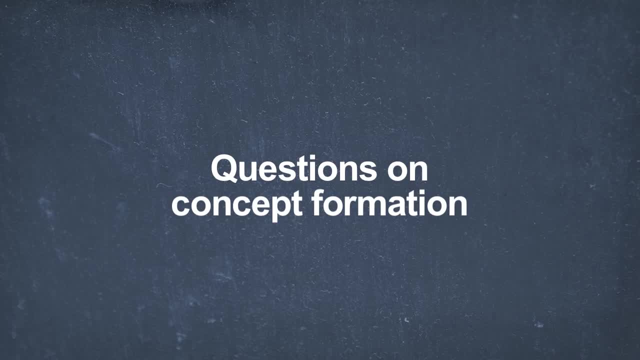 Similarity is a relationship you detect between it and another, But the concept doesn't stand for similarities. Similarity is simply the relation every concrete within a group has to each other. Similarity means partly the same and partly not. The concept stands for the entity. 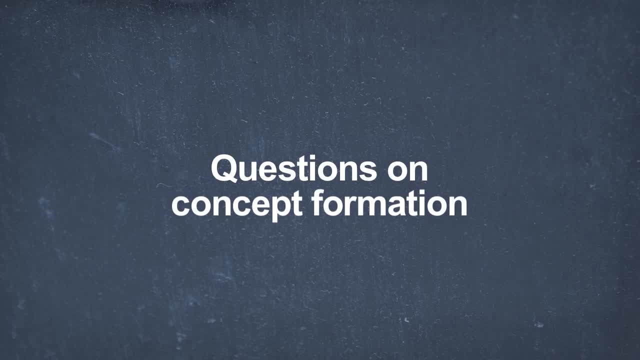 but, viewed from a certain perspective, The entity considered as belonging to this group. Now, you could only do that if you were able to grasp similarities, But it's not as though the concept grasps only the similarity and is oblivious to anything else. You can use concepts to grasp what's unique about a thing. 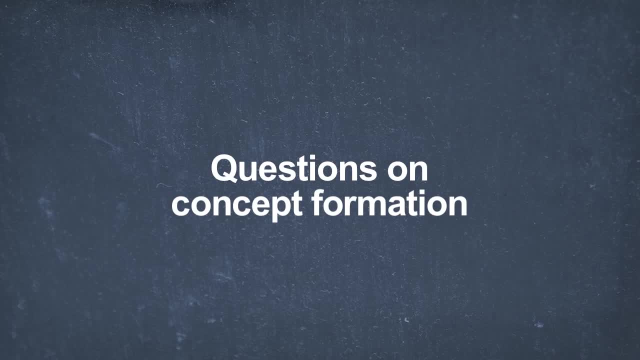 Using a certain amount of concepts, I can tell what's distinctive in you, so I wouldn't want to make it as though concepts can never grasp uniqueness. They can only grasp. you know what's common Concepts. grasp a thing with its attributes. 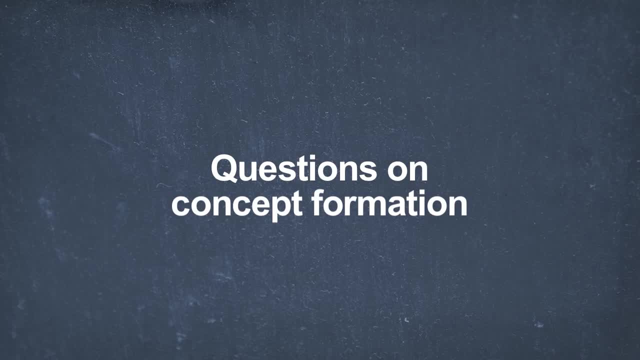 and, if necessary, with its distinctive measurements. You use concepts to grasp that. Now you say: are they an integration of percepts or are they an integration of existence concrete? Both depending upon what context you're talking about. How do we? 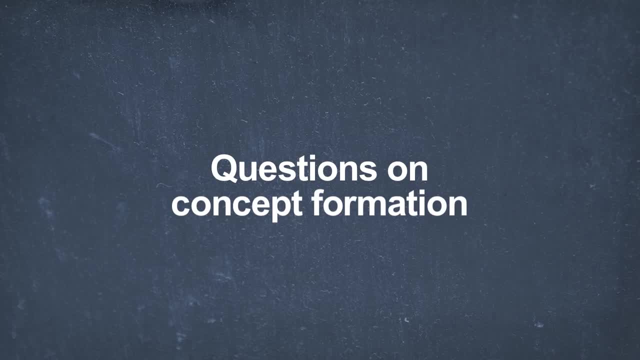 Certainly, they're an integration of concretes of existence. But now then, the question is: how do we get to know existence? We can only know them through our sensory faculties And cognition. remember, the perceptual level is the given. 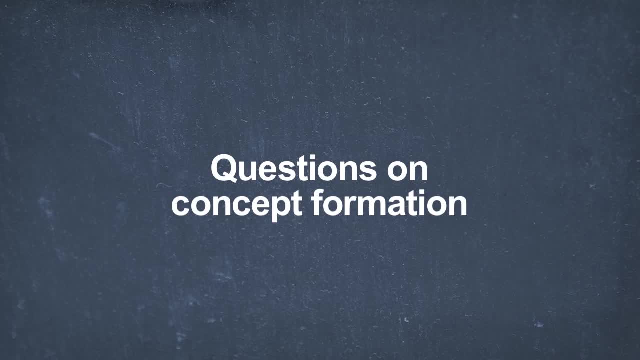 So when I say to you: integrate concretes, and you say to me: I'm sorry, I can't do it, all I have is percepts. That would not be. it's not a different thing. That means you're integrating concrete as you grasp them. 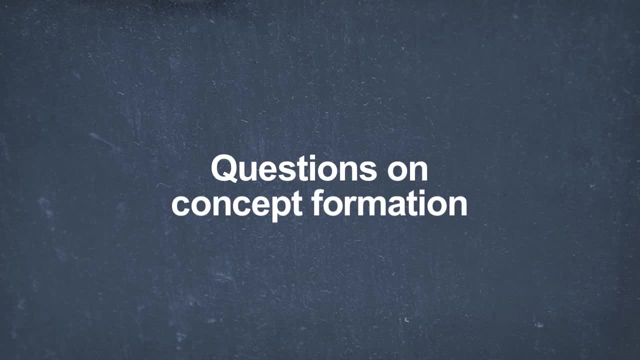 And that that the direct object grasping is the grasp of a concrete as a person And therefore there's no clash between the statement that concepts integrate are integrations of existence or concretes. that is the metaphysical formulation. 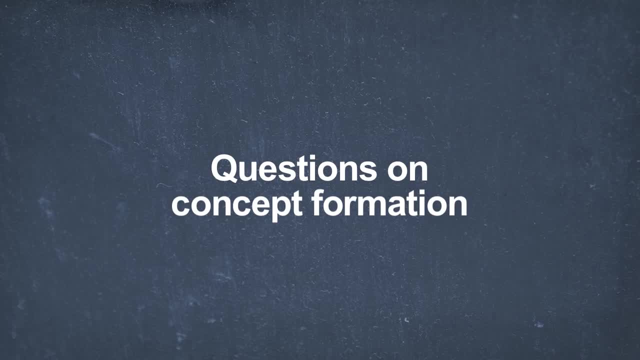 or concepts are integrations of percepts. Now you say, isn't a concept a mental state? Yes, it's a mental state, But that is not enough to tell you. It's a very special kind of mental state. Closest I come to describing the concept without the word. 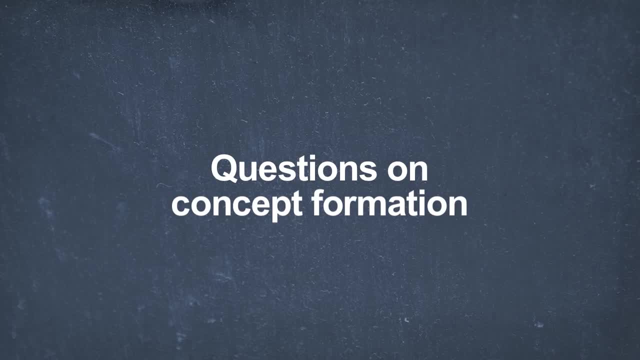 is on page 117.. If you didn't have words, but you focused on a group of persons, you observed their similarity as against some other group. you focused on them and you said: I'm going to keep them together and everything else like them. 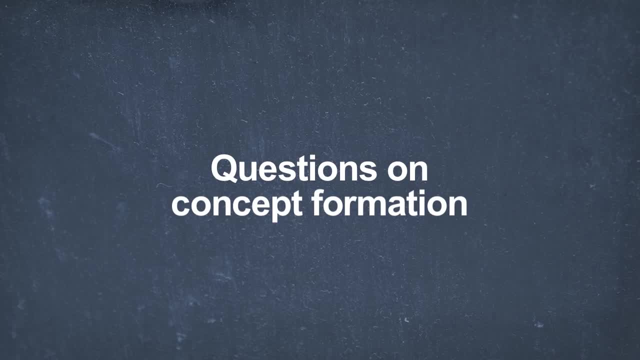 There's a moment where you could do that before you have a word. That is the mental state, the conceptual, that is the concept. The concept is the resolve to treat all these instances as one, The grasp that they're all like each other. as against that, 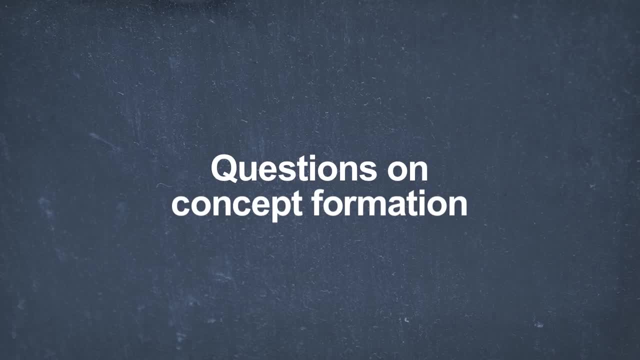 so you're going to treat them as one, But that is a very even. the words I used are an unwieldy state. It has to be pinned down and turned into something perceptual before it becomes an actual unit, And that's why we say that the word completes the concept. 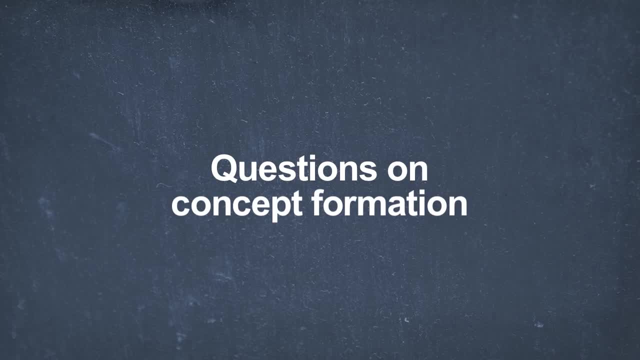 When you say I'm going to call a dog, then that sound or that shape becomes what actually occupies the mind, that person, And it then stands for everything within the group. So, strictly speaking, a concept is the word standing or the word completing the integration. 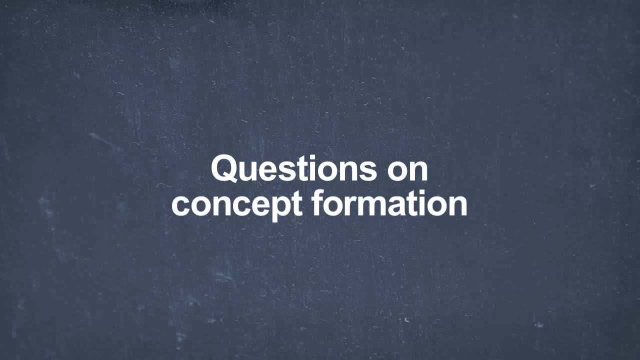 And that total mental state designates concretes as perceived. So you can, depending on how you look at it, it's a mental state, the concept is a word. it's an integration of percepts, it's an integration of existence. 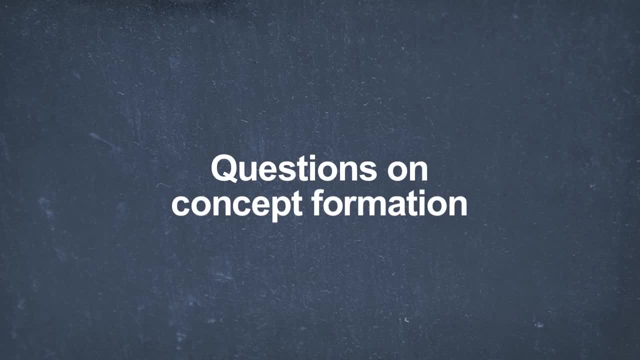 Those formulations do not clash with one another. Yes, The perspective I was asking about is the perspective of what's actually left over in your mind after you finish forming a concept. So I take it that the answer is: it's what's actually left over in your mind. 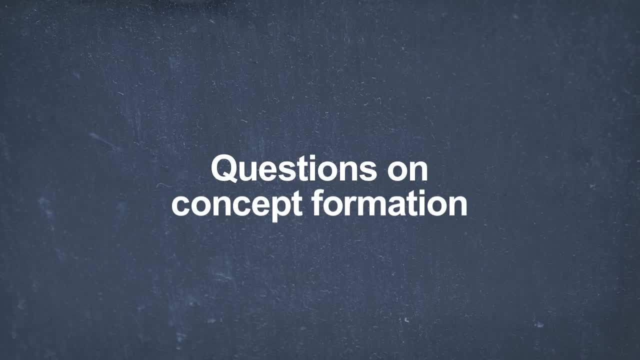 is a word, What is left in your mind. if someone could inventory your mind with a mental fluoroscope, they would see the word. I don't know how you would do that, but the word or your knowledge of the word, that would be the file in the subconscious. 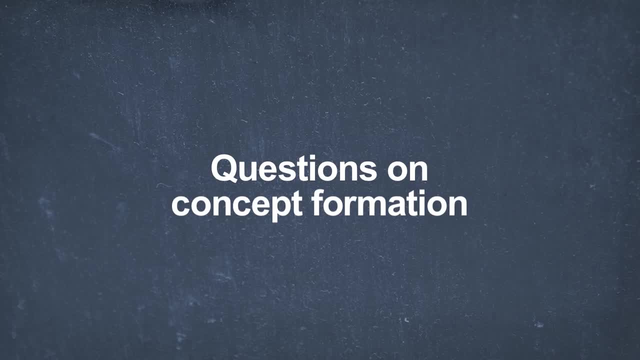 would be the unit That is the new unit. But that word is not just a noise. If I say that is not a concept, It doesn't stand for anything. It doesn't result from any segregation of one group of percepts from the others. 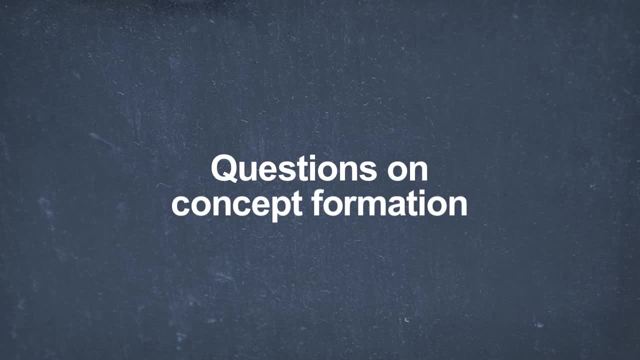 No abstraction, nothing. So a word is not the same as a noise. But if you understand a word in the sense that a perceptual symbol, completing the integration, turning that unwieldy resolve into an actual perceived unit, that is what a concept is. 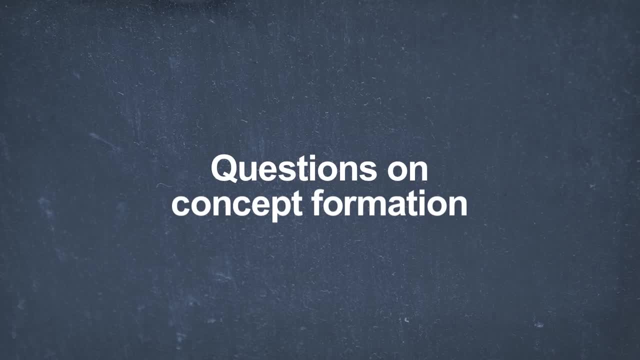 Yes, Could a word be just a mental picture? Could a word be a mental picture Rather than like letters? It can in primitive situations, but you could not get very far with images. Ayn Rand discusses that. There's a very interesting discussion of that. 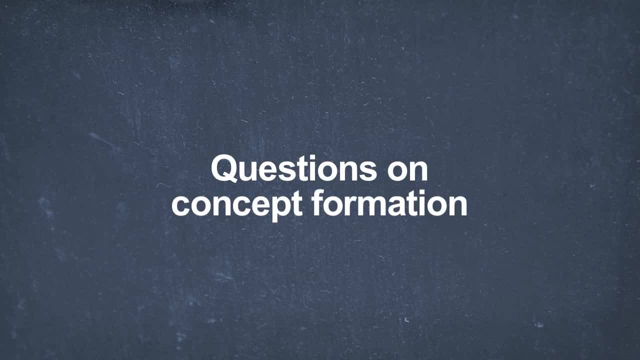 in this book, Introduction to Objectivist Epistemology, Why you need a fully symbolic code rather than just an image. Someone there asked her- I think it was with regard to a man or a notebook or something, but why do you need the word notebook? 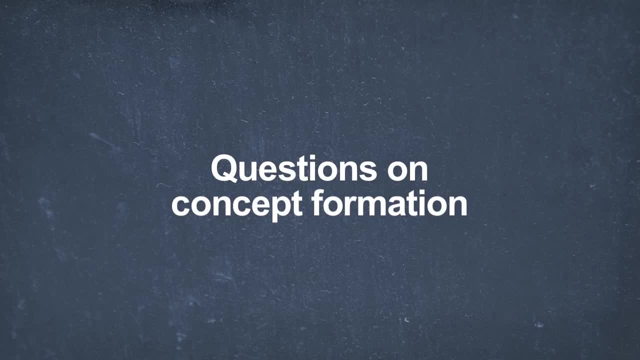 Why can't you just hold an actual image of notebook before your eye with the mental resolve- I don't mean just this notebook, I mean this notebook and anything else that's like it- And you carry around the concrete which pins down your integration becomes one of the concretes in the class. 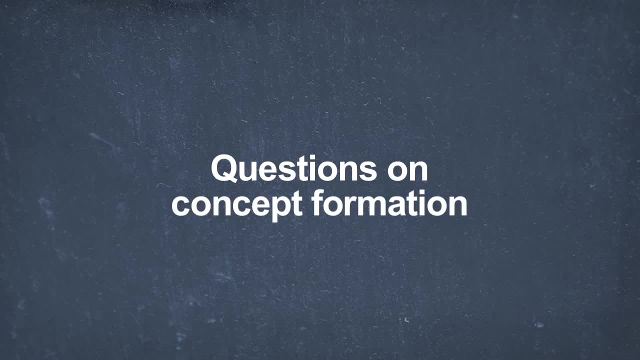 an image rather than the total, And her point was that you could not work with images on the level required and still keep your tie to reality. You know, on a very primitive level and probably on the early stages of the conceptual development, you can. 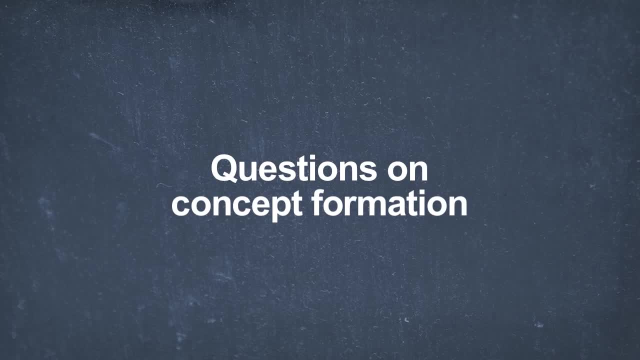 But at a certain point, when you're talking about things like justice, marriage and so on, to try to hold it by a little image of all the aspects, it would be the same as basically having to go back to the perceptual level and start all over again. 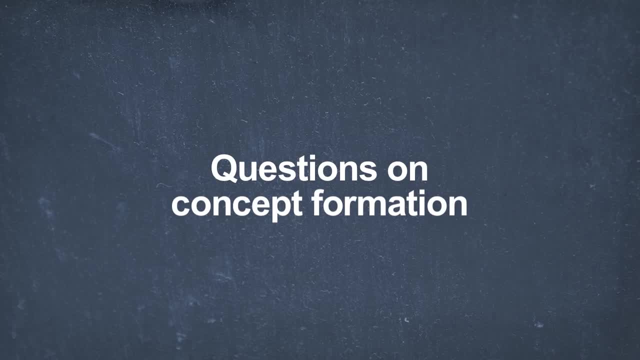 Even on notebook it wouldn't work very well, as she points out, because I mean even on that primitive, primary, ostensive level, because when you gazed at this little notebook, it, for instance, would have a spring binding. And you're saying: it's this: 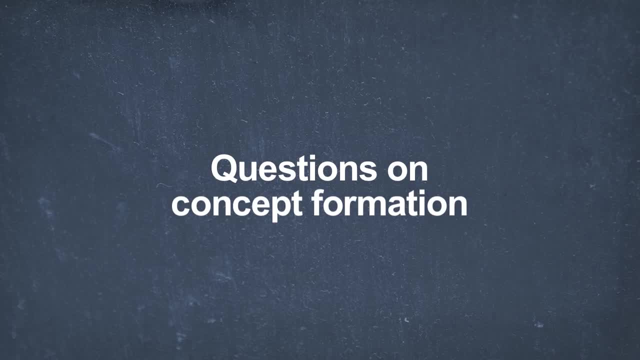 and everything similar to it. But you'd have to say: well, now, of course I don't mean the spring binding, because that doesn't count under notebook, This is a thick one. No, no, I don't mean the thickness. 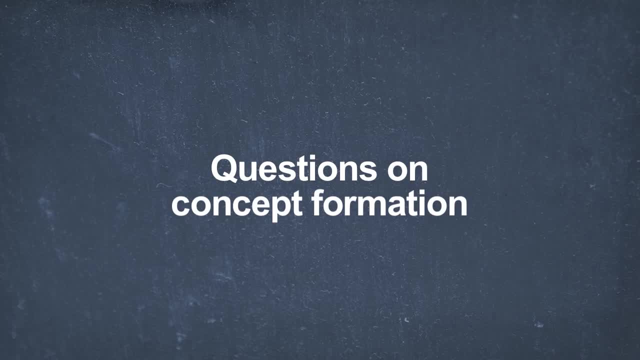 That you know it can be thin. In other words, by the sheer act of bringing an actual, perceptual, concrete, even if in imagistic form, before your eyes, your mind has the challenge to figure out. well, which aspect of this? 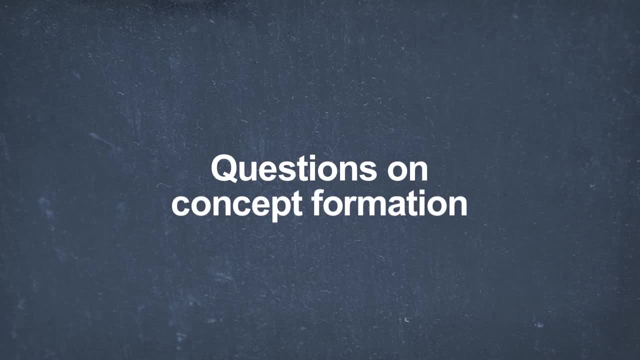 is it you're talking about? Since you're holding it by one of its concretes, you're back to square one. You have to do the perceptual abstracting over again, And so an image is at best a transitory state. 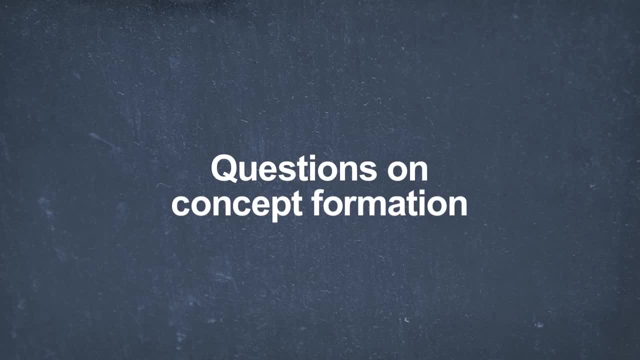 There's some evidence that children use images at the beginning in place of language. But in order to reach full efficacy on the conceptual level, and especially to get to the higher levels, you cannot do it by images. She also in there discusses which I refer you to. 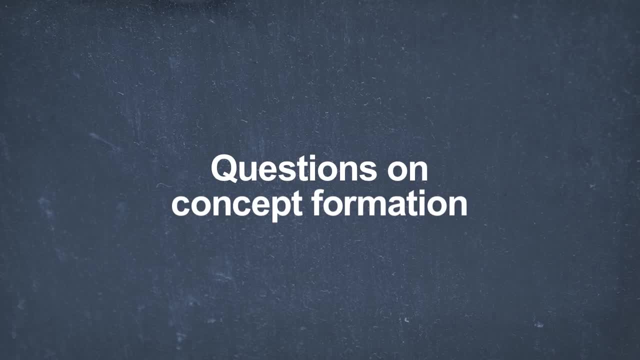 could you try to hold your concept by an emotion rather than a word? That is somebody. she gives the example. somebody is disgusted at tables and he tries to hold table by a feeling of disgust. instead of the word table, He perceives them in the abstract, and so on. 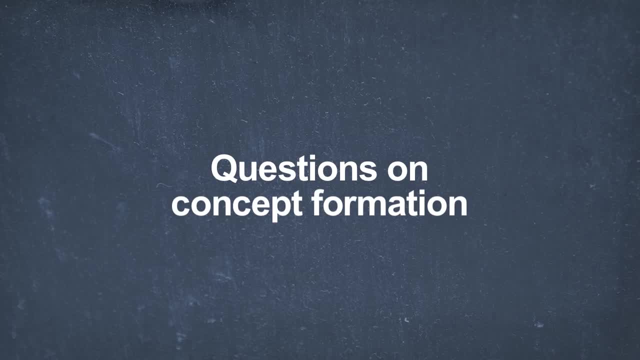 but instead of picking a sound, he just focuses on revulsion, And every time he wants to say where's the table, He says where's the? and he feels that in his state. Well, of course, you see that that is impractical. 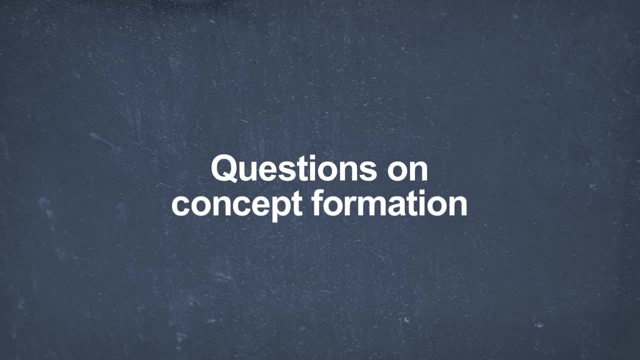 Even to sum it up, the revulsion would destroy his whole mental state, And it would be. it's an analogous to what would be the problem of the mind. It's the problem of anything other than a purely symbolic code, which doesn't require of you any experience. 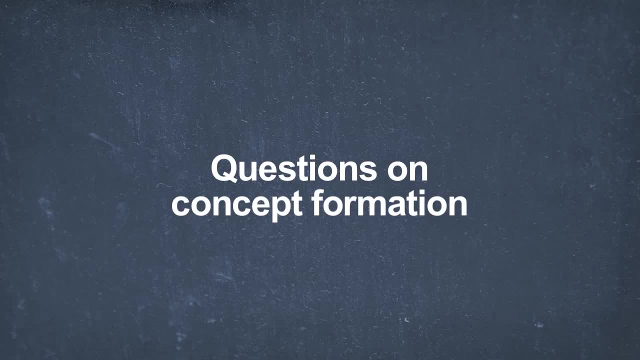 any perception, just a cipher, an empty perceptual datum. That's exactly what we want. It would be like trying to do algebra. Maybe I'll give you this analogy: Trying to do algebra by saying, instead of using A, let's call it five. 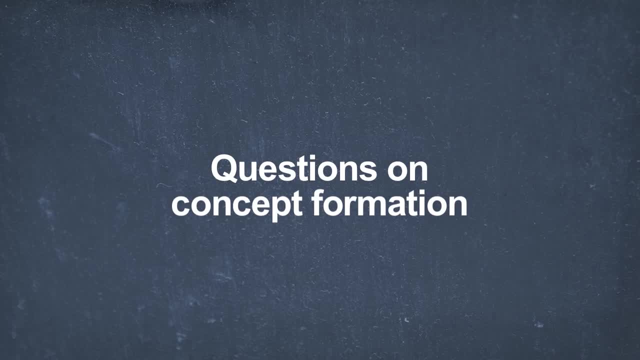 But remember that we don't mean five, We mean any number, but we're just gonna keep five because we feel happier with it. You couldn't do it. The sheer fiveness of five would obliterate your mental process until you got to A. 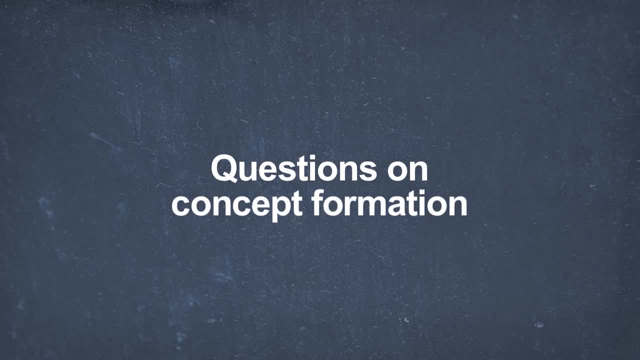 And that's the reason why you need a word, not an image. That's a good question. Yes, You discussed how concept formation is the beginning of, where there's volition involved, where the perceptual level is automatic. On page 115,. 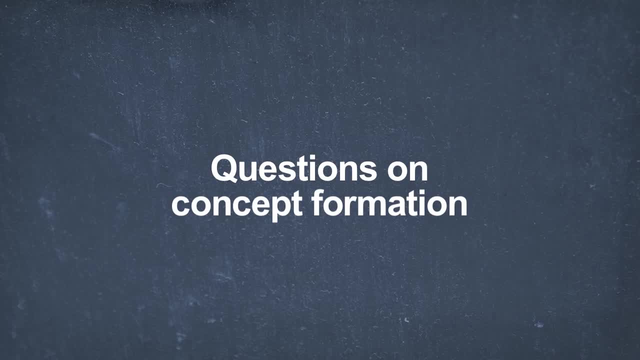 you remind us of the fact that concept formation is the beginning of a volitional process. But I'm troubled by the fact that you seem to be suggesting that similarities as opposed to differences these two processes of concept formation. similarities, you seem to suggest. 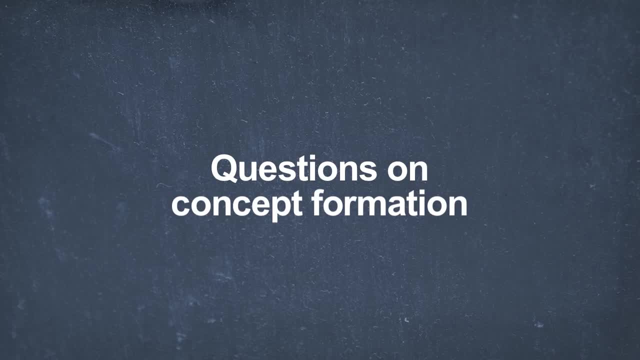 are given to us automatically. Well, the first similarities are certainly given to us automatically. The early similarities, yes. The similarity and difference is if those are the two parts of concept formation. it sounds as though you were allowing in sort of automatic aspect to concept. 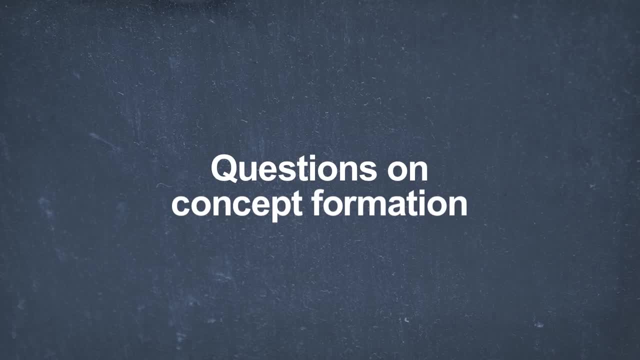 I think there is definitely an automatic aspect to the first stages of concept formation. I definitely think that I do not believe that there's a clean break between the automatic perceptual level and then the completely volitional conceptual level. I say as a general principle. 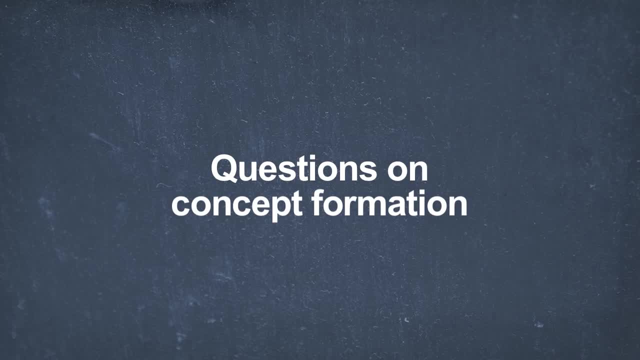 volition is coextensive with the conceptual level. But the early stages of the conceptual level, the stages of the conceptual level, are built on direct observation And there, I think, probably on a desert island, starting completely from scratch. now I'm just hypothesizing here. 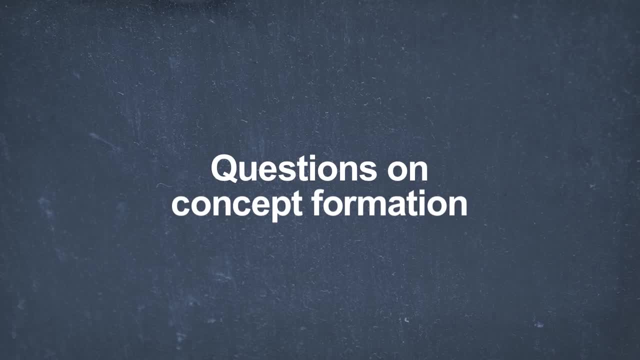 you would have to use volition even to get table or rock or whatever. your first one is because it would have to occur to you with a separate act of focus, not only to perceive that this is like this, but to focus on this as against this. 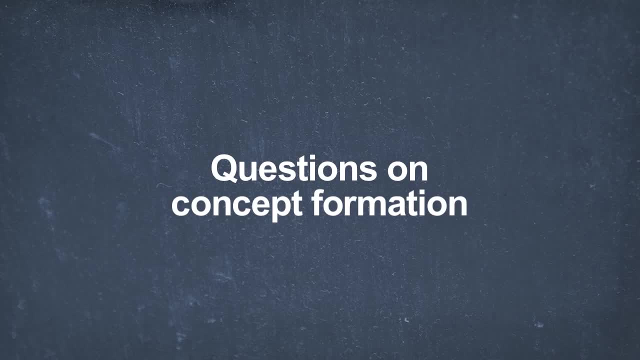 This is like this. this is like this. as against that, And now I'm going to, you know, you'd have to invent language, you see? So you'd have to be a tremendous volitional achievement and, as a result, 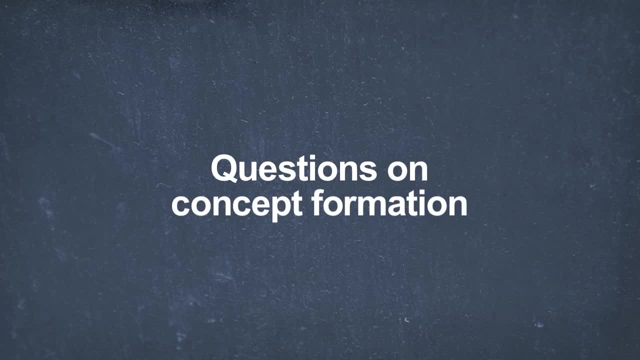 you'd get probably only a few words in your lifetime, But that is not analogous to the situation as we have been growing up and learning language from others. In the present situation, I do not believe volition is required on the early levels, That is, if you have a mother showing the child. 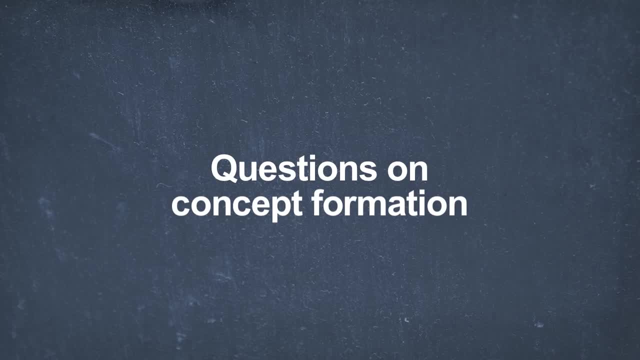 all the time: ball, ball, you know. and that's not a square, and it's not so, and it's a ball, it's not a block. She points the number of instances as against the others and gives it a name so repeatedly. 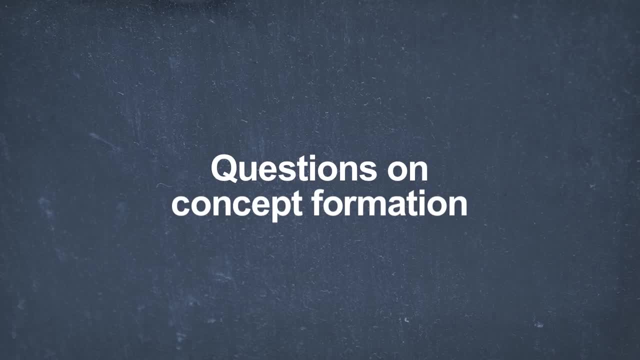 that it does not take anything in the sense of choice on the part of the child to be able to grasp right away this as against that, and he's given the unit. All he has to do is simply be minimally receptive and have an unimpaired mind. 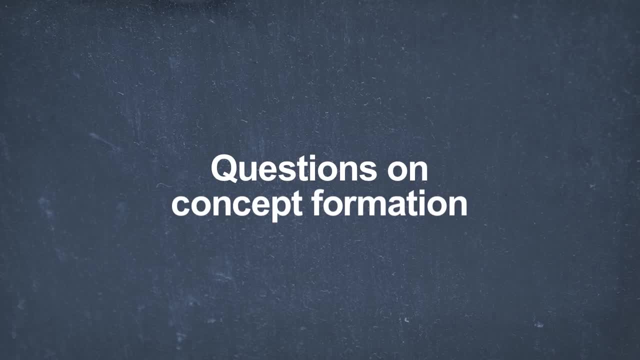 and that much is automatic. Where it stops being automatic is when other people can no more do it for you, When you get to the point where, no matter how often they point it out, it isn't a direct perceptual thing. You just open your eyes. 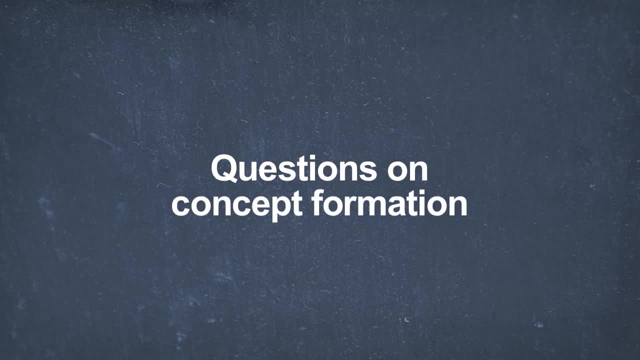 and you see certain similarities. Oh yeah, that's not this. When you get to higher level concepts, when you get to integrations of consciousness and existence, when you get to concepts of consciousness, when you get to that kind of complexity, 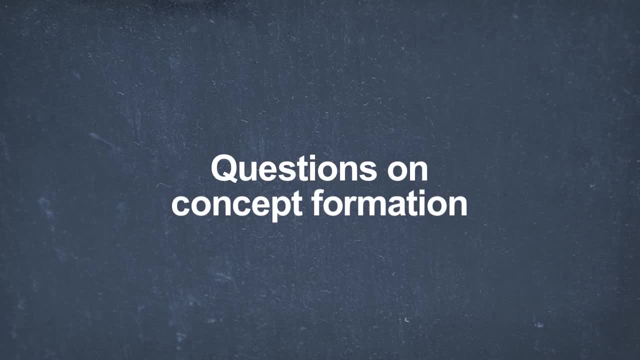 there is no way to make the process automatic the way it is on the very early first level perceptual level concept. But it is true, I think that there is an automatic boost that we're given at the beginning While we're on that page. 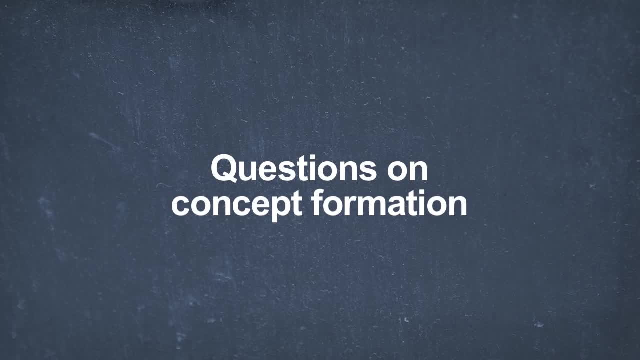 I would like to just stress this sentence that you mentioned: the similarities which make possible our first differentiations are observed. In other words, we don't need conceptual knowledge to reach to grasp that these things are similar, And this is very important. 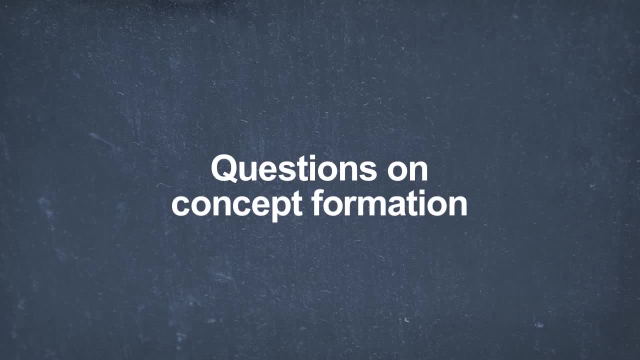 because rationalists historically tend to deny that percepts can give us any information. Anytime you'd say: I learned this by perception. they will try to construct an argument to show that you couldn't have learned it by perception. For instance, they'll say: 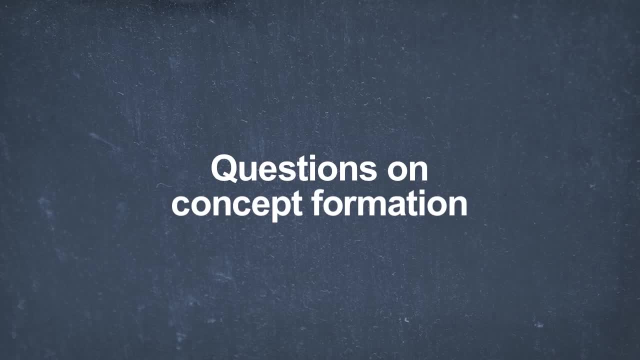 I gave the example. you can see that this thing projecting is longer than this thing projecting. And a Platonist will say: how could it be longer? You don't have the concept length. How can you know it's longer? Well, of course you don't know. in words: 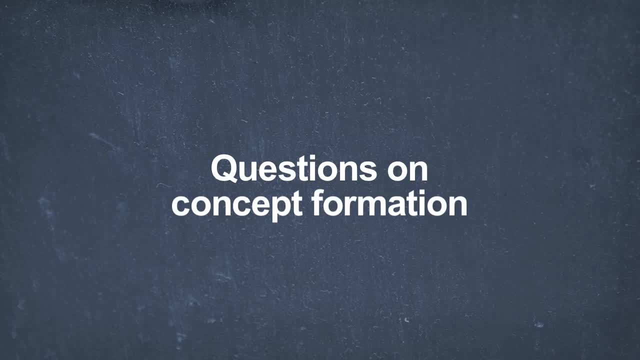 that it's longer, but you can perceive what we as adults describe as one thing being bigger than another, even without the concept. You can perceive the relationship And that simply is giving you by observation, even though you can't conceptualize it. 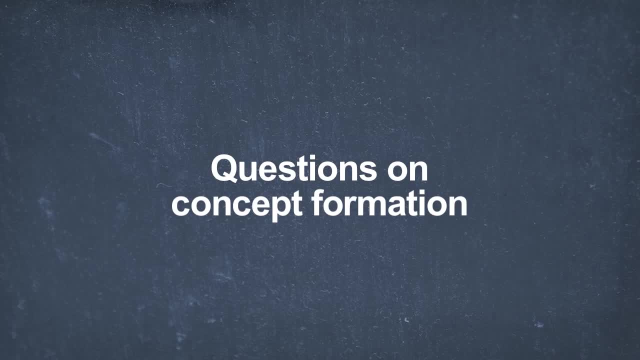 Now, I point this out because there are people like rationalists who think that you can't get anything from perception. All knowledge rests on conceptualization. Well, if that were true, you couldn't have concepts There. first has to be the perceptual data. 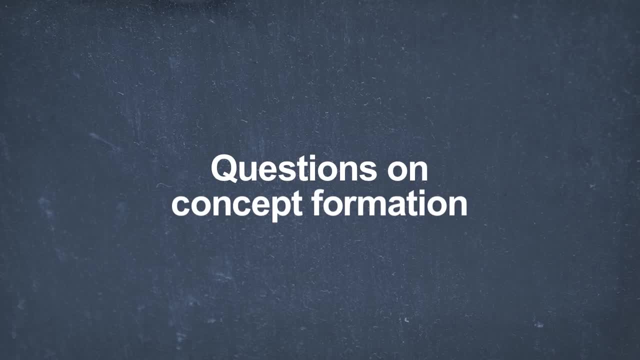 that concepts integrate. Another example of that is the gentleman in the workshops who I said to Ayn Rand: how could you possibly get the idea of function from observation? I can see a table, but I can't see the function of a table. 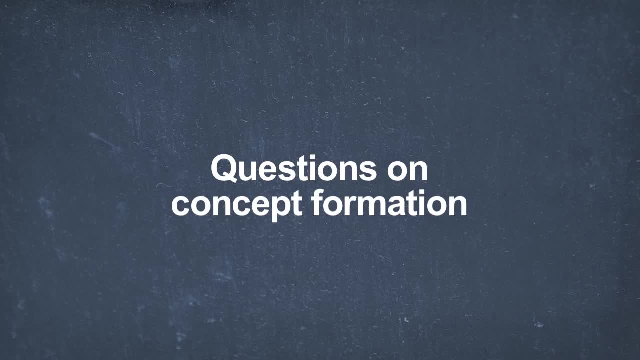 So how could you grasp function from perception? And her answer was: lie on the table and then lie on a bed. That's the difference. When you see, ah, this one doesn't feel good and the other one does. you now know what the function of a bed. 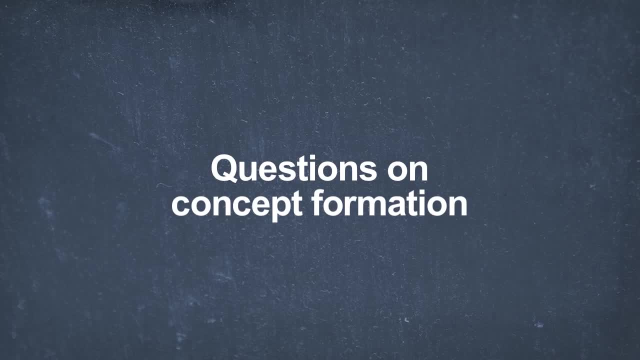 as against. the table is So it is a directly observable issue. There's two mistakes you can make: To say percepts give us nothing or percepts give us everything. Empiricists tend to say percepts give us everything. 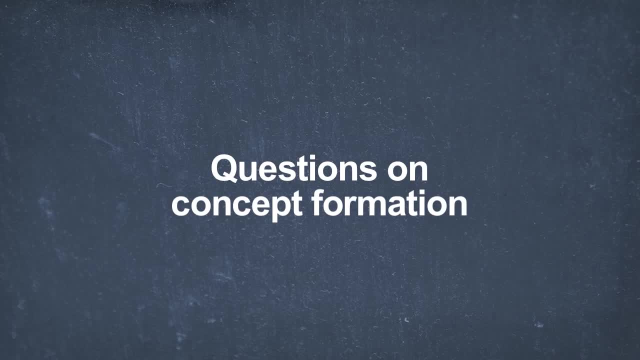 Rationalists say percepts give us nothing. The truth is, percepts give us real, vital, crucial information, And on that basis we are then able to reach the conceptual level and do something with the information. Now, while we're on this page, 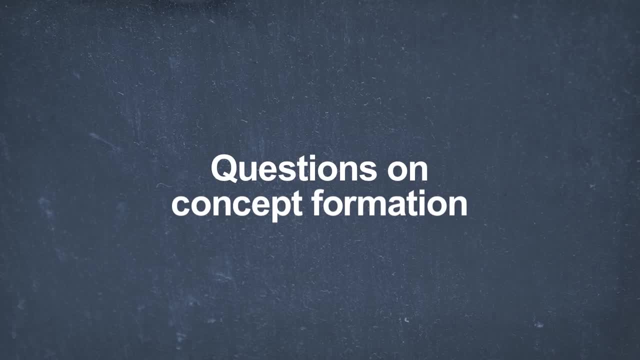 I wanted to go to the very top and just explain one word. That statement, table 115,. integration is the process of uniting elements into an inseparable whole. I don't know if my intention in putting inseparable in was clear. Is that clear to you? 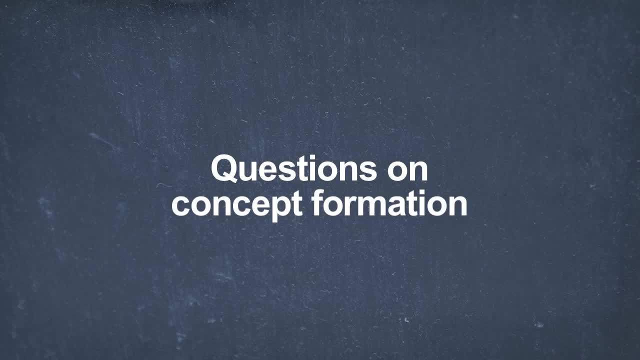 why I put the word inseparable there and not just said uniting elements into a whole, which I could have said. but I was trying to bring out a certain angle here. Does anybody have an idea what I'm trying to stress there? Yes, 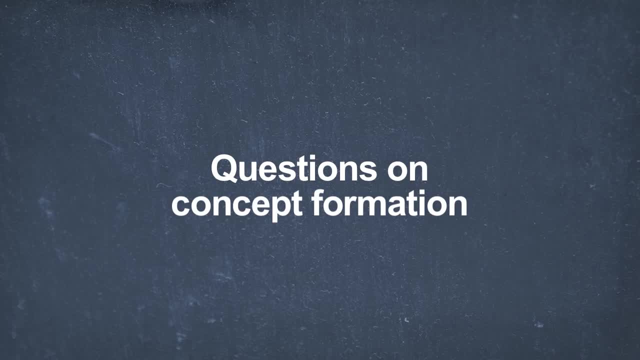 Once you form a concept and it is valid, that concept will be valid forever. Well, it's not just that the concept is valid. The units are actually blended into a new single unit. It's not what I'm trying to say. 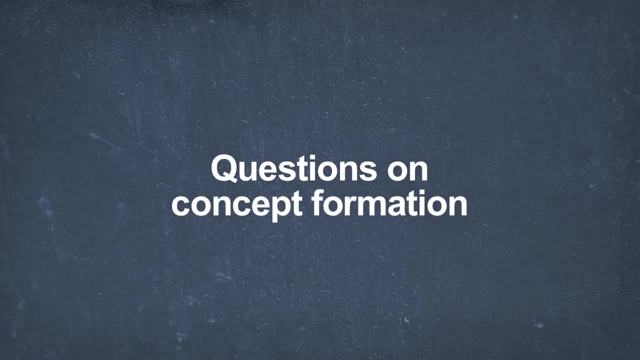 and this applies on the perceptual and the conceptual level. When you integrate sensations into a percept, that is a percept. it's a complex state of awareness, has many aspects, but it's reduced to one unit mentally, And in that sense, 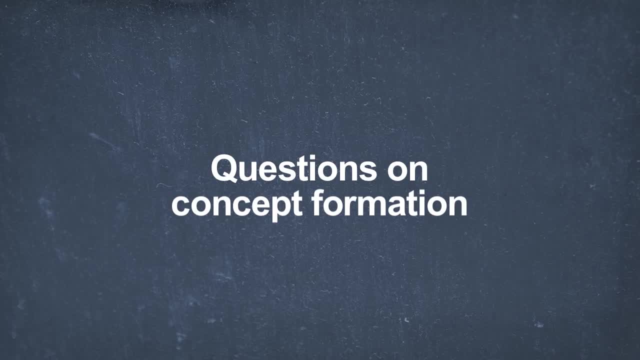 it's a whole which all the parts are tightly interconnected. to make one new phenomenon. I don't mean a whole in the sense of just an amassing of parts side by side like a pile of junk. you know, in the junkyard you could call a whole. 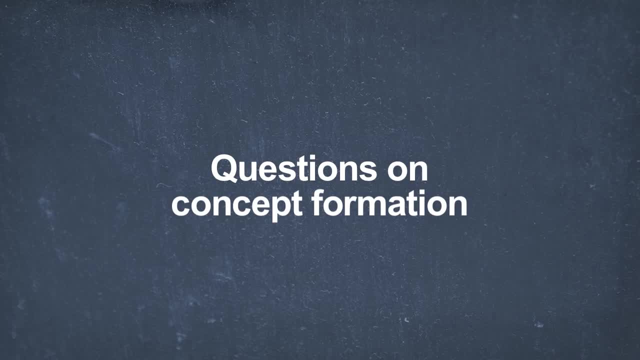 all the stuff in the junkyard, But that is not what we're talking about here. We're talking about parts actually blended or welded. You have to use an analogy because the actual experience is unique, but parts actually put together into a single unit. 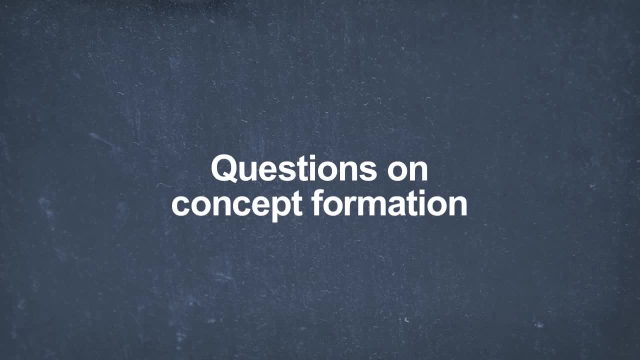 which is no longer torn apart. And the same is true when you go from percepts to concepts. Once you have table, all tables are blended together: past, present and future contained in that one, And you don't any longer, unless you go back to the perceptual imaging level. 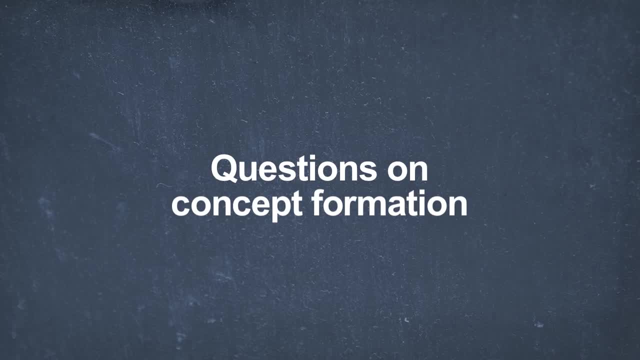 have this percept: this one, this one and this one, You have all of them in one unit, And that's what I'm trying to get at. It really is a whole, in other words, not just an accumulation. It's not just that you view tables side by side. 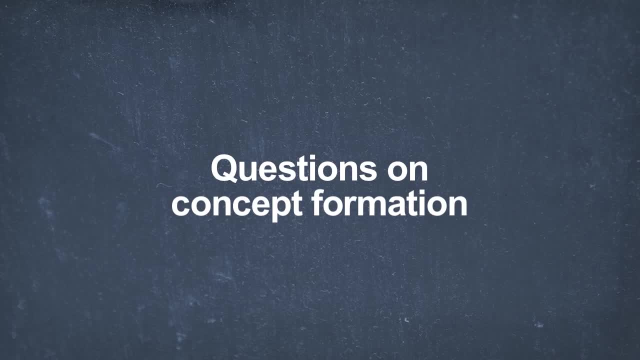 You actually put them together into a new phenomenon, And that is the concept table. That was all of that. I tried to get into the word inseparable. All right, I'll take another question on this section. Yes, What is the status of this discussion of concepts? 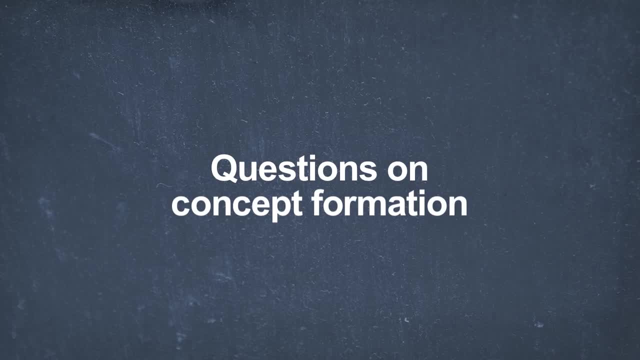 Is it just a description of a process of concept formation? Because concepts I would think are required for proof Are what Are required to give a proof. So is this a proof of concept formation or just a description? I asked on-run. 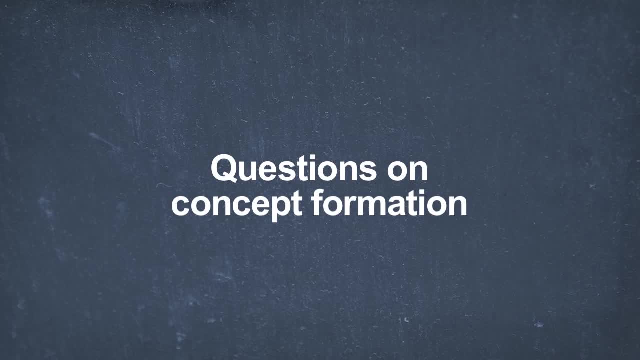 What was the status of her theory of concept formation? Could she give me a proof of it? She said: well, you read my book. You've read the substance of what I have to say. What do you want as a proof? And I immediately said: well, I want some set of axioms. 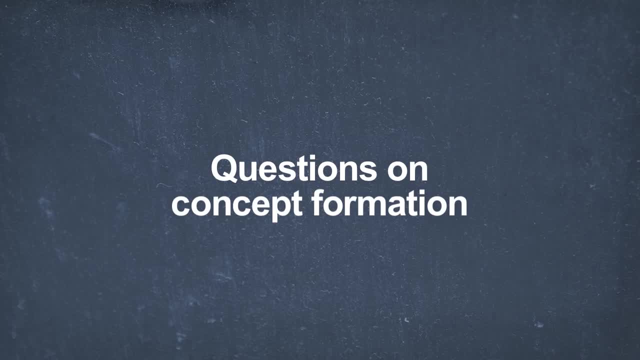 from which I can deduce that this is the way concepts must be given, as in the primacy of existence and so on. Therefore, concepts must be measurement omission. And she said: yes, you could guess what she said, But that is trying to turn it into rationalism. 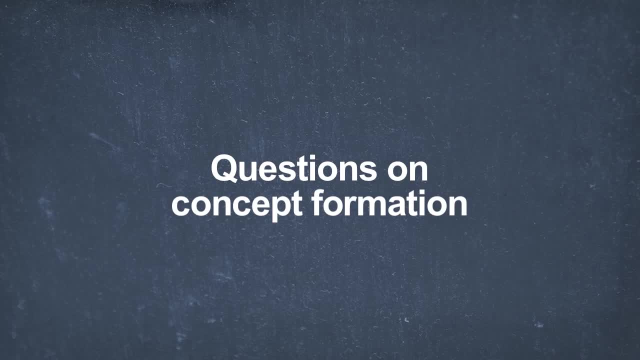 She said: regard this as simply an inductive generalization. Regard it as I observed what my mind was doing. I noticed that I'm omitting measurements. I checked it against every type of concept. I see that it covers consciousness and existence. 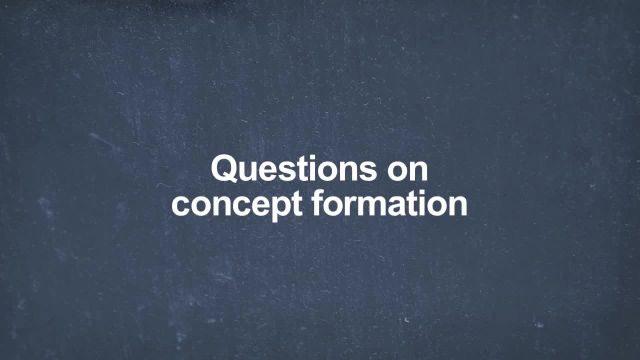 and entity and attribute and higher level and lower level. It integrates all the data. If anybody doesn't check with my observation, let them tell me where it doesn't check. If he found some other process at work, then we'll expand our knowledge to include another process. 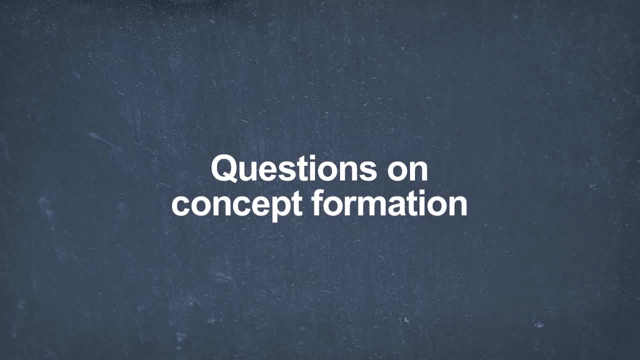 if he really finds it. But she said it's very crucial not to view philosophy as a deductive system With a series of you know a few axioms and then everything else just follows, like geometry. It is not like mathematics. 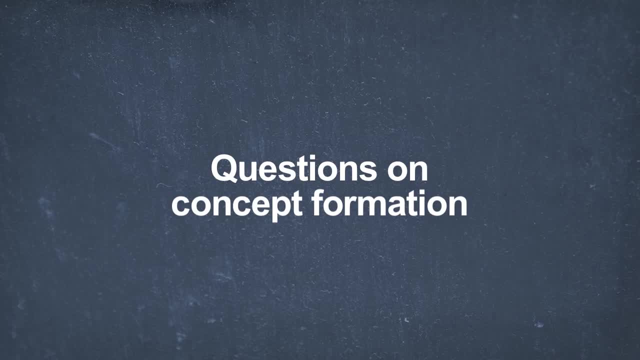 It's continual. turning to reality, It's new information And certainly the theory of concept formation she herself regarded as inductive. That's a good question. I want to just make a couple of points myself before we get to the next section. 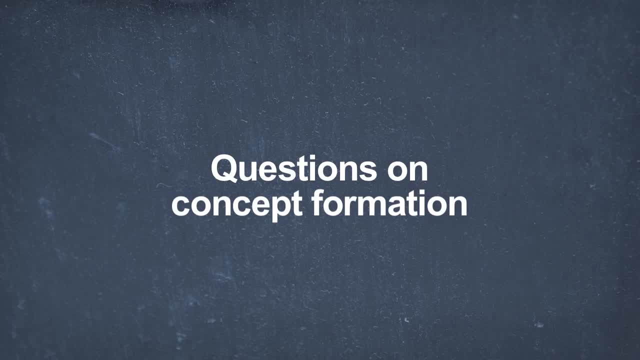 the things I wanted to point out to you, And then I want to go back to chapter 13.. This paragraph near the bottom, at the bottom, about starting: although the unit perspective is crucial, it is important to grasp that in the world apart from men, 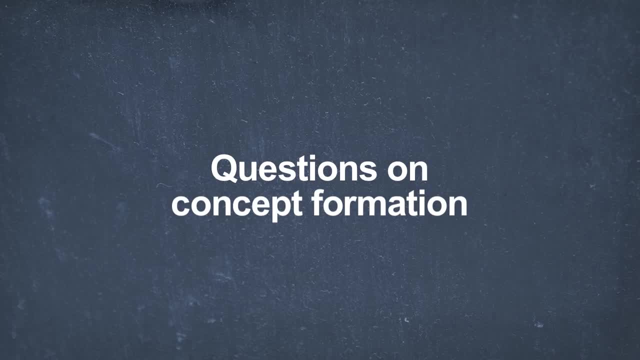 there are no units. What are we there setting up? How many can looking ahead? what is this? why is this point so important? That in the world, apart from men, there are no units. there are only existence. Why is that important? 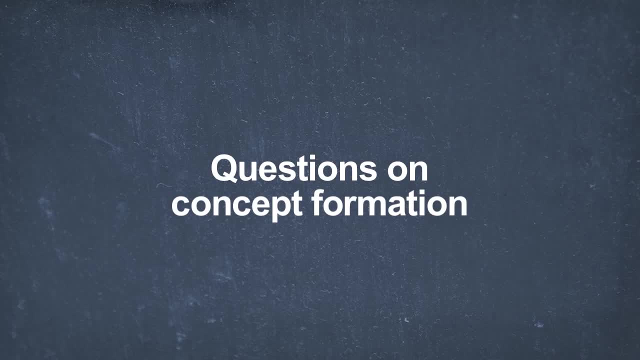 What is the philosophic significance? Yes, Units are inherent in having a construct and only men have constructs. Well, what am I trying to get to with that? This is, of course, Ayn Rand's point. Yes, Units are mental entities. 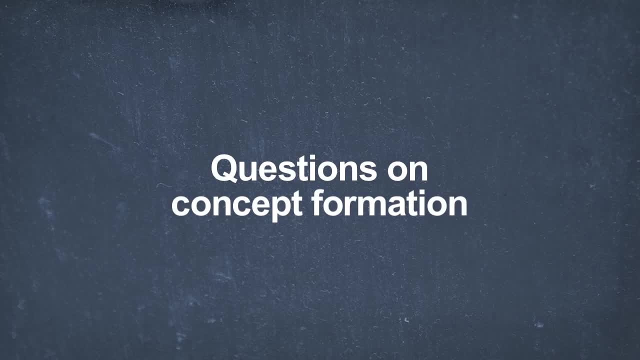 They're mental, but then are they arbitrary? They're not arbitrary. It's a perspective on reality, so that it's dictated by reality, conjoined with objectivity. It's our form of awareness. It's a human perspective on reality. 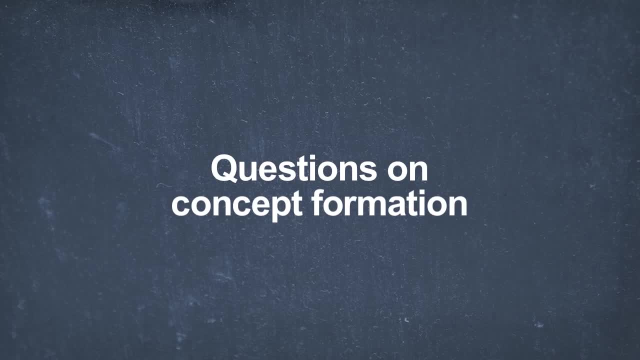 In contrast to what A quote from Ms Rand Note that the concept unit involves an act of consciousness, a selective focus, a certain way of regarding things. In other words, man, you could say, creates units. Reality doesn't. 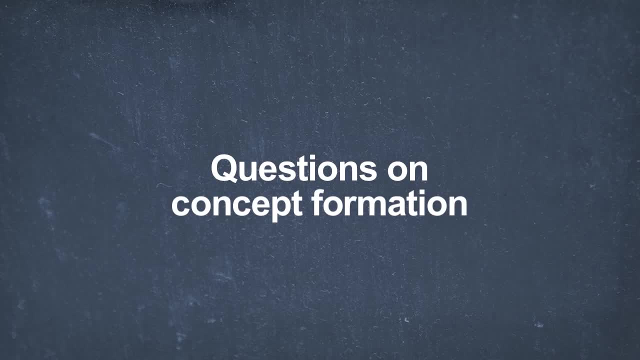 We have to look at things a certain way, segregate things a certain way, create a certain relationship, And therefore units are not quote out there. They are not with an I intrinsic. On the other hand, she goes on immediately. 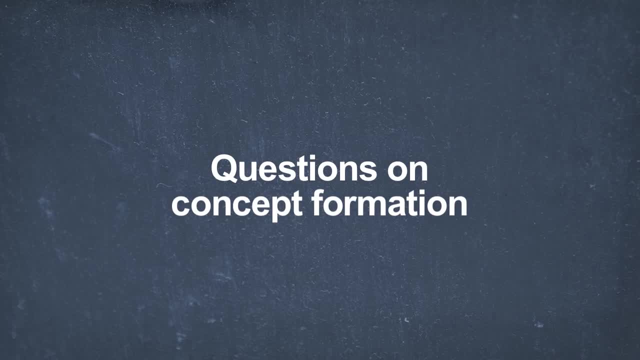 that they are not a unit, is not an arbitrary creation of consciousness, Because when you do focus on things a certain way, certain similarities do obtain certain differences and there's a certain method by which you have to organize the material. In other words, it's not subjective. 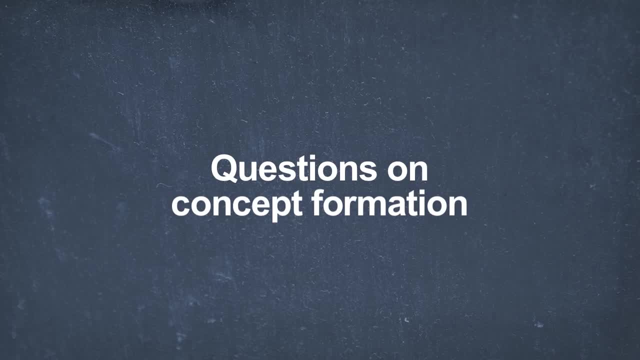 So right, in this very discussion of unit, which is the root of concept formation, is the whole set up of objectivity. A thing is objective- we'll see when we get to the next chapter- if it's a fact as organized by a volitional consciousness. 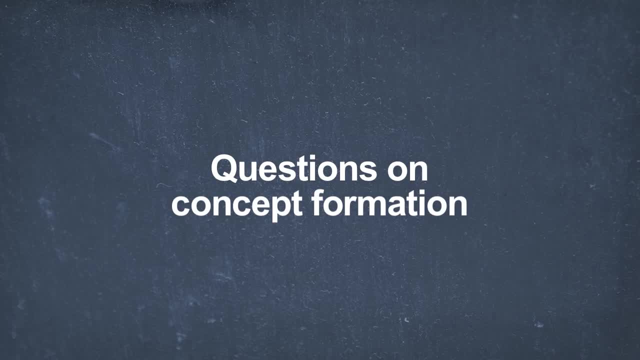 And here the union of existence and consciousness is right in the very idea of unit, And that's what I wanted you to see, that it's we're laying, we're not laying. I mean, this is the fact about the whole conscious perspective. 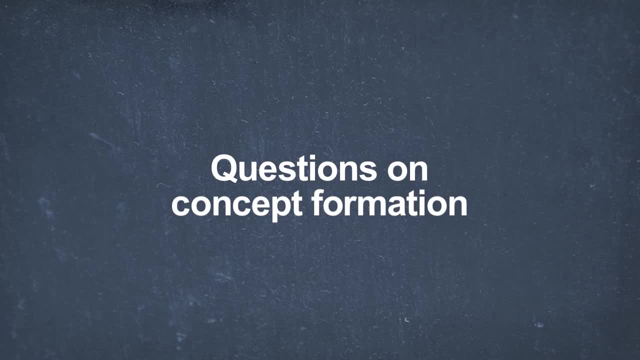 the whole conceptual perspective that gives rise to the concept of objectivity. It goes back to the fact that in forming a concept we have a distinctive human perspective, so it's not intrinsic, but it's a perspective on reality, on facts, so it's not subjective. 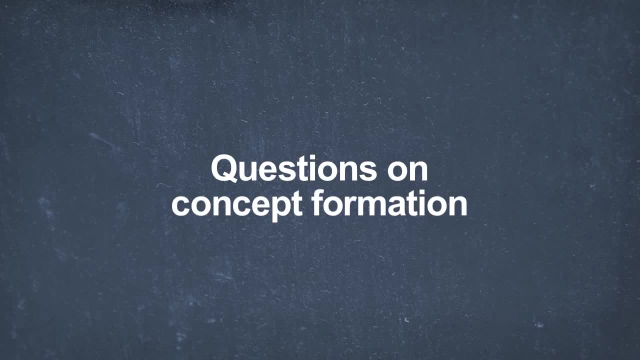 And that's will be essential as we develop. Oh, one other thing I wanted to point out. I think in this section a couple others: Page 116. Near the top, that definition of abstraction is the power of selective focus and treatment. 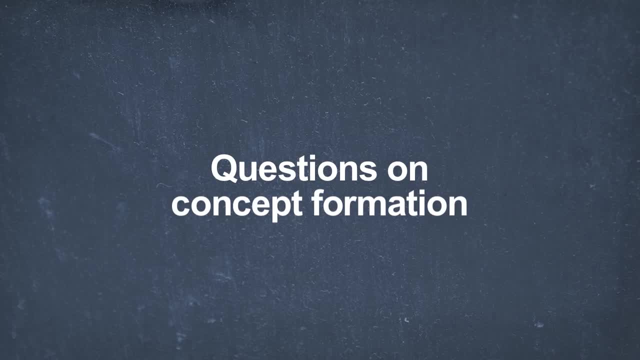 And then I elaborate the power to separate and make cognitive use of. Now that the ands there were deliberate as a result of a discussion with Ms Rand, I had always thought just the power to separate mentally or the power to focus selectively. 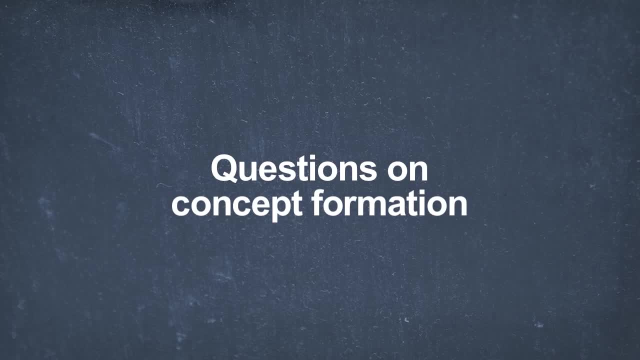 I had always defined abstraction as that, And she said that is much too passive to describe what abstraction is as a process. Abstraction is not simply selective perception. It's not simply gazing at part of what you have Conceivably an animal could squeeze in. 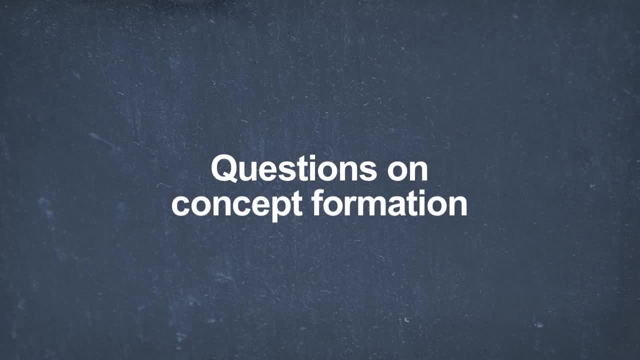 or squint in some way and just look at the underside of the table without the rest of it, Just narrow its focus to some separable aspect. But he is not abstracting. Abstracting, she said, is not simply selective focus. It's selective focus which becomes the basis. 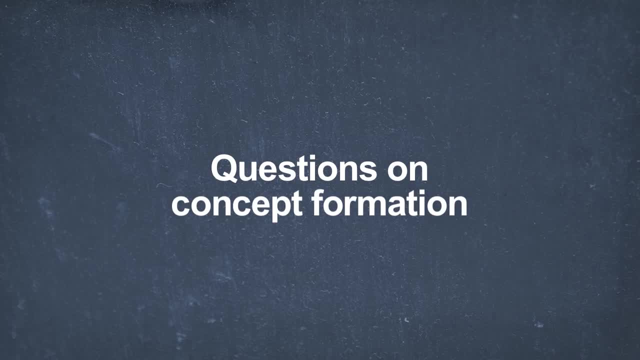 of a whole way of using your consciousness, Selective focus that you then use as a way of organizing all of your cognition. You see it's selective focus as a means to the conceptual level, And that's why the definition has to include selective focus. 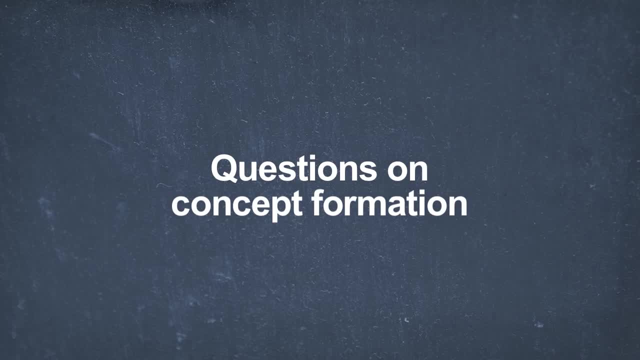 and then treatment, Make use of it, Do something with it, And that is the active aspect of abstraction. I'm just pointing out these little things that you may have missed. And in 118, I must say I think that this is a good line on my part. 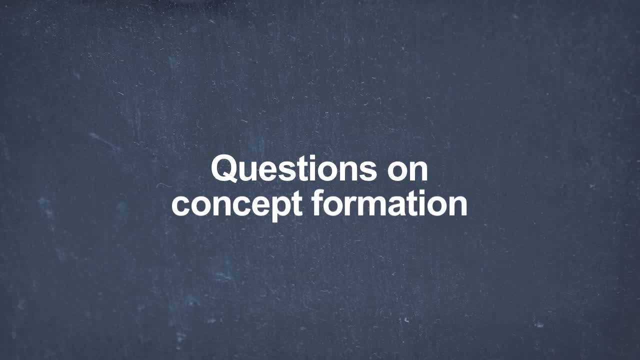 right in the middle, The word is the body and the conscious perspective involves the soul And the relation between those two is different. It's just like body and soul And I found that helpful. I like that. I must say All right. 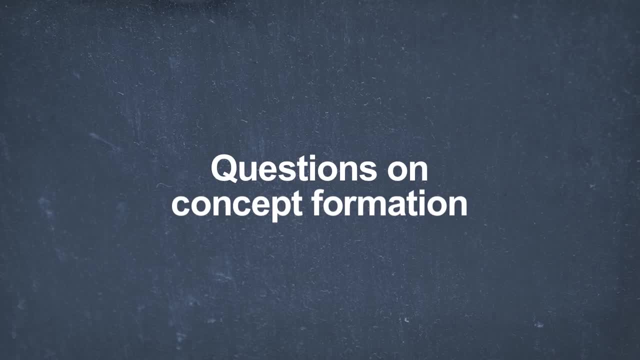 Now let's go to the second section, which is the last I want to do today. Do I have a question? Now? that, of course, is the heart of the whole thing here. Concept formation as a mathematical process: Yes, Considering the nominalists. 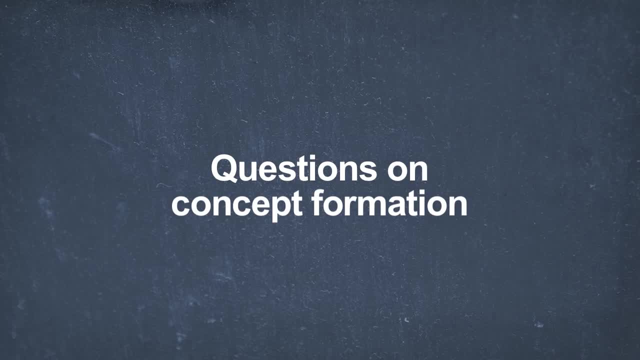 how they come at formation, the concept where they look out at the world and they say: I don't see anything the same between you and I, for example. All characteristics are different And in our view, where you say the mental process, 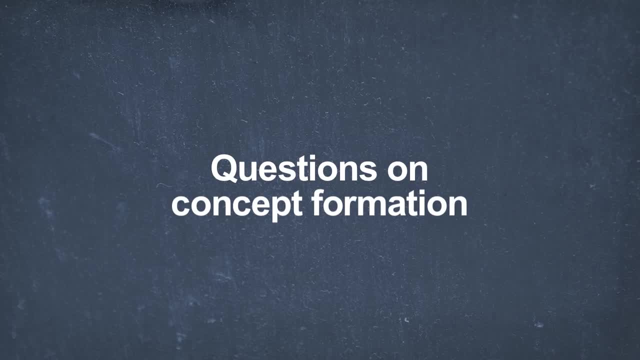 on page 123,. the mental process consists in retaining the characteristics. You could have the word same in there, the same characteristics. Well, could you put the word the same in? No, I wouldn't want to put the word the same in. 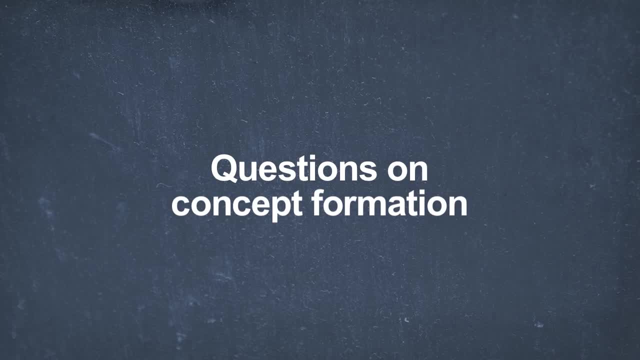 I'll tell you My question was going to be: I'd like you to comment on the way I've been thinking about the nominalists in connection with this. Is it the case that they are viewing every different instance of a characteristic as a different characteristic? 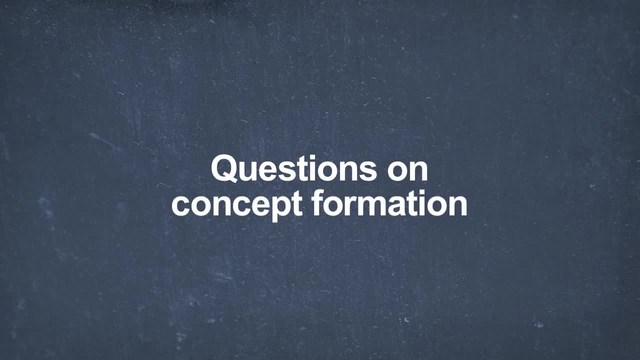 Yes, sometimes they do do that. For instance, if you have a, an arm that's six, what- 15 inches long and somebody else is a 16, they'll say: you have the characteristic of a 15-inch arm and he has the characteristic of a 16-inch arm. 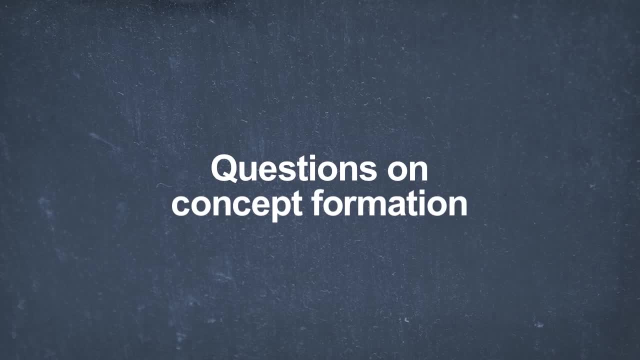 so they're not the same. In other words, they're defining characteristic in such a way that it's absolutely specific, down to its measurement. Well, if that's the case, then you need another word for what's left after you omit measurement. 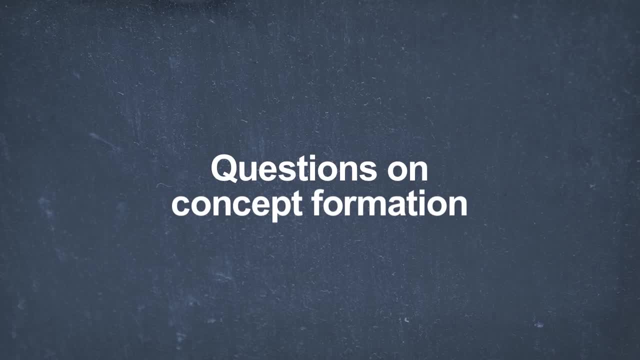 You know, words are defenseless. You can. Everything is quote. a characteristic, Characteristic is that which characterizes something. Everything in the universe characterizes you. Whatever is true of you, a measurement, an attribute, you name it. 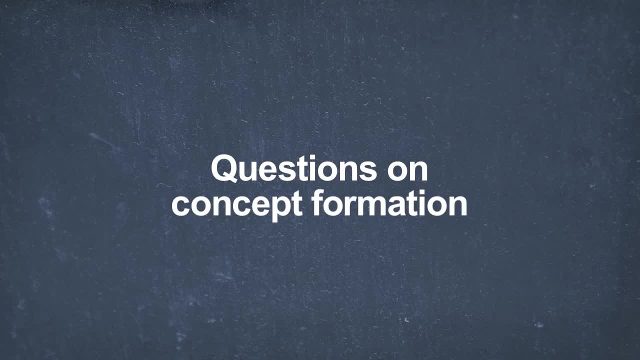 it's an aspect of you, But obviously, when we make a distinction between characteristic and measurement, we are doing it because we're not using characteristic in that all-encompassing, global way. We're using characteristic in a way that's not characteristic. 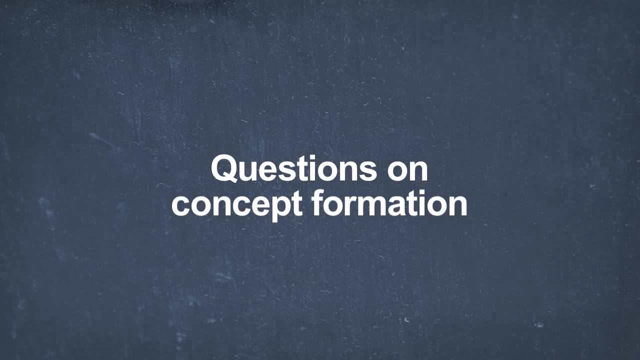 We're using characteristic for the feature, the attribute that ultimately has to be ostensive, such as length, or having two arms, having two eyes, having a rational faculty, having a heart. you see which characteristic, in any given instance, varies in measurement. 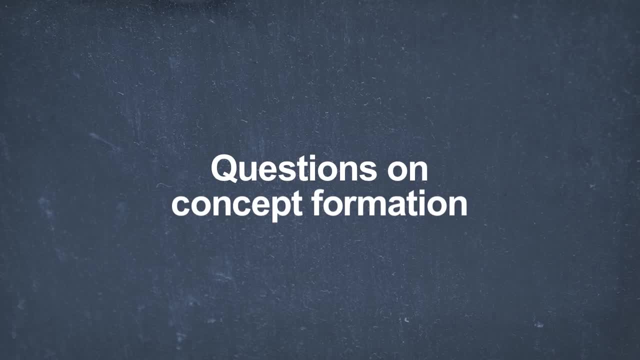 in many measurements, not just size but shape, color, texture and all the rest of it- It varies on a continuum more or less on many different axes. And what we mean when we say we retain the characteristics, it's not just we retain. 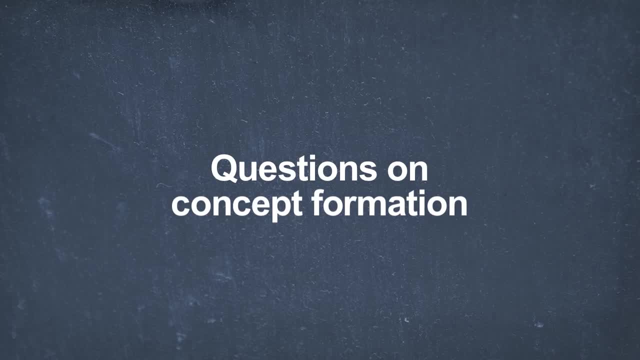 the same characteristics but drop different ones. Given the use of characteristic versus measurement, we retain all the characteristics. but the point is, the theory is that the entities vary only in measurements. What's left when you drop out measurements is characteristics. So if you put the word 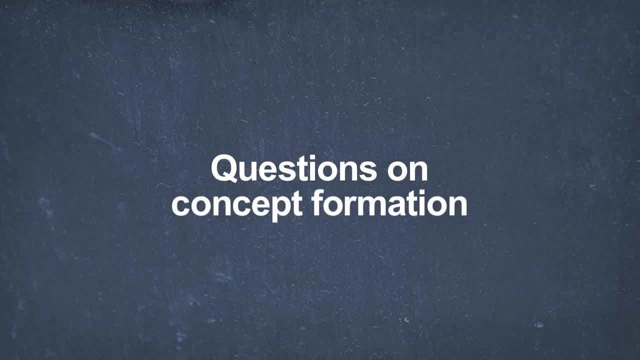 same in there. you see, you'd be switching the meaning of characteristic, and then you would collapse the theory. It's true that the characteristics remaining are the same, but the reason is that we put together in a group only those things which are commensurable. 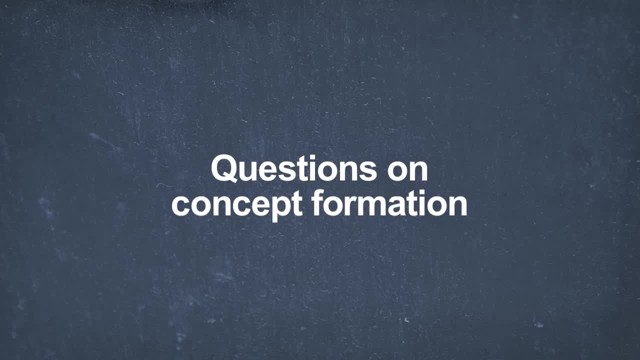 And that means those things which we can relate to the same unit, that is, those things which differ only in measurement. See what I'm saying. Does that answer you? Oh good, On this subject, it's hard to answer anybody, because it's. 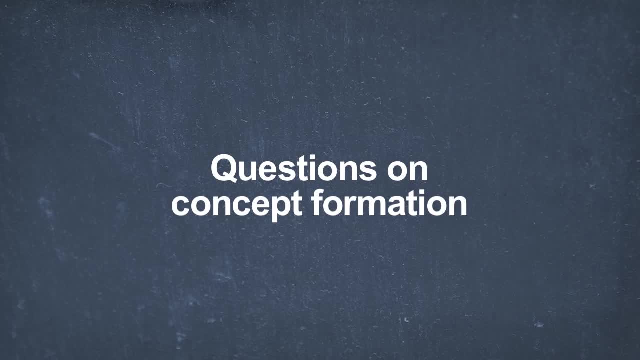 It's not straightforward. Yes, Just a question about optional characteristics and concept formation. Optional characteristics: Yes, I never heard that one Go ahead. Well, the idea that you know a table could have some trim on it, and so 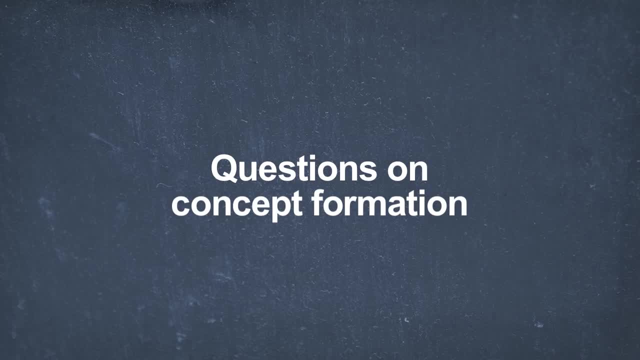 Oh, oh. You know, another table doesn't have to have trim. It could have zero trim in that other table. That's not an optional. I mean it's optional whether you make a table that way, but the word wouldn't apply. 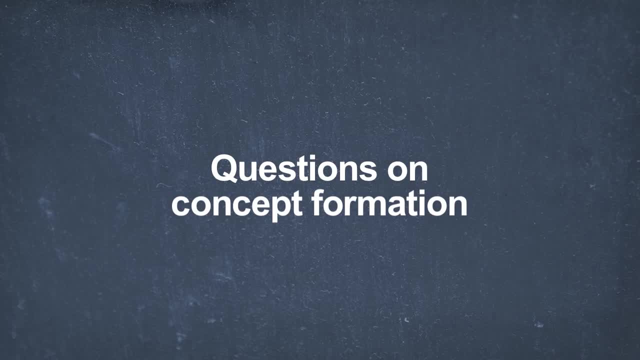 Every concrete differs, Right, But here's the question. Yeah, What I'm worried about is how optional can you get? I mean, you go to a park and you want to have lunch and you say I need a table, So you pull a blanket. 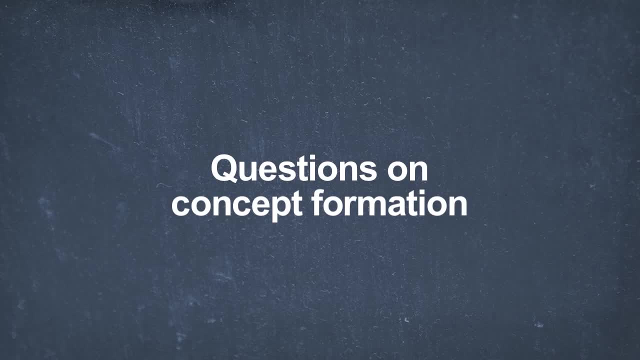 out of your car and you put it down and you know now you're using a blanket as a table. Can you really apply table that way or No? you cannot. And in fact that very example was covered, not the blanket. 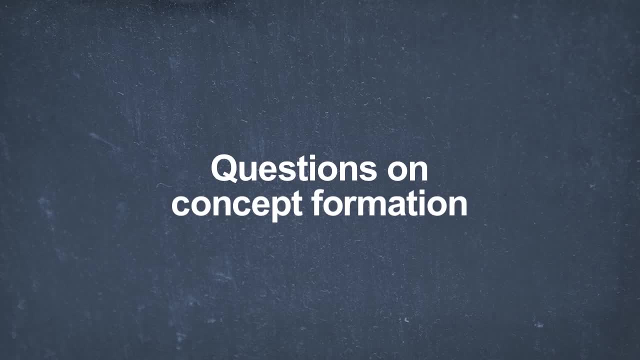 but an equivalent of it in the next chapter. Did you read the next chapter? Yes, That is exactly like the question that Ayn Rand was asked by a professor of philosophy. A table hung from the ceiling. Now you've got a table. 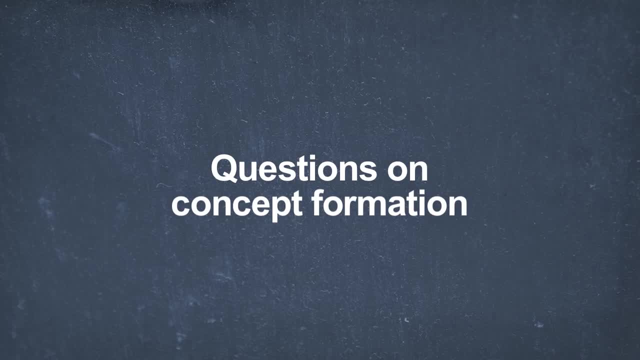 lying on the ground in the form of a blanket. So it's exactly the same thing, And you want to know how do you draw the line? First of all, that doesn't belong to this chapter, because that's the question. Now that we know, 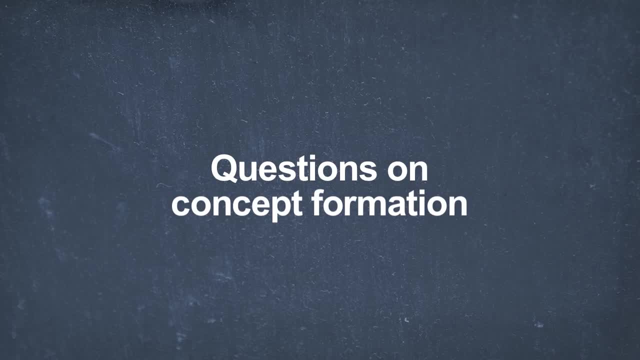 how concepts are formed and defined. when should we form them and when shouldn't we? When should we say that the variation between instances is so insignificant that, even though they vary, they belong to the same concept? as against, The differences are so great that they belong? 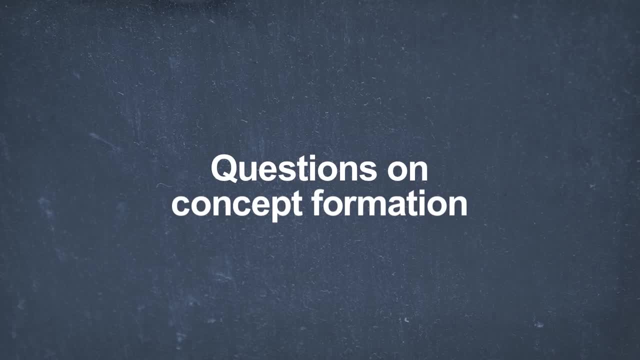 to different concepts as against It's borderline so that they're close to both. That's covered in the next chapter and that depends entirely on how essential are the similarities or the differences, And essential depends on your context of knowledge and you have to then. 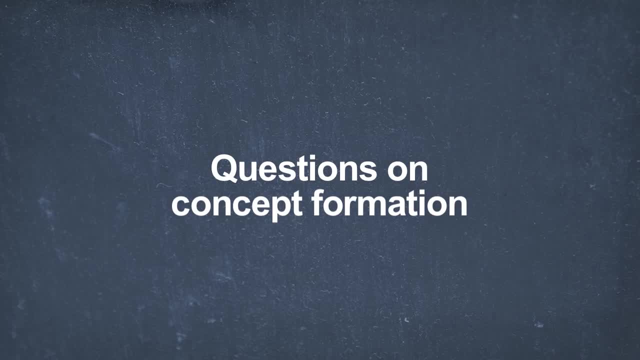 judge according to the material there To give you a quick, fast answer. certainly, a blanket is not a blanket, A table. there are essential differences in the structure and in the uses to which you can put it. A table will hold something and a blanket will conform. 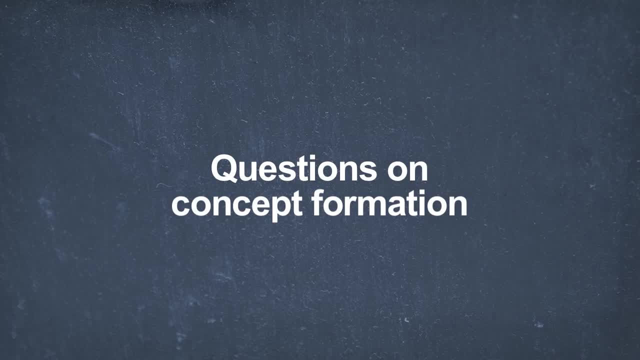 to the roughness of the ground. When you put something, it'll fall down. A table has a certain height and you can therefore have a certain security of things walking under it. As against a blanket, anybody can walk on top of it. The same reason. 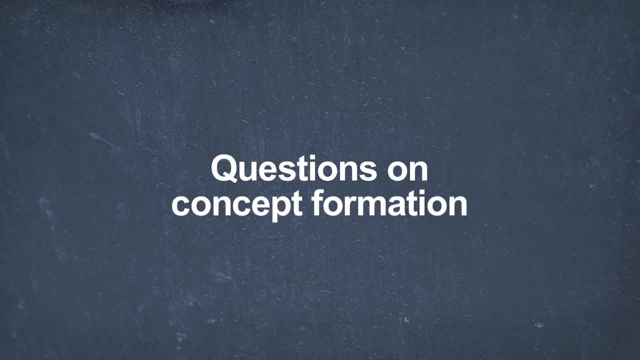 why you would think it's significant not to put your best china out in the middle of the living room floor. So you would say, well, if somebody said to you, well, it's optional, you would be continuously apprehensive. not only that, you have 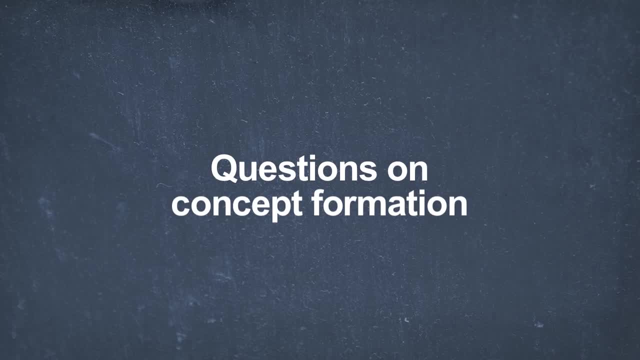 to bend down all the way to get it, but that anybody will walk over and smash it. And that's because, objectively, there's a difference between a surface meant for the feet and a surface elevated to separate away from the part meant for the feet. 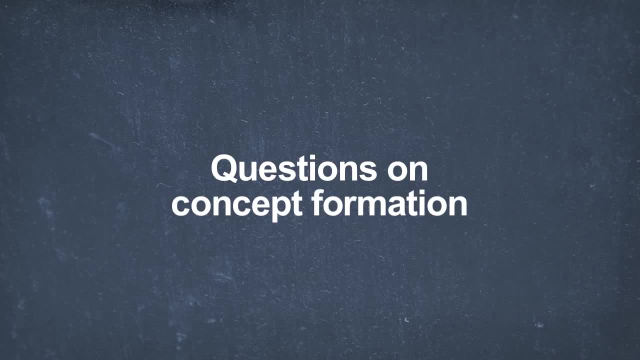 and which is given a sturdiness and flatness so that it will hold things A blanket, doesn't have any of those characteristics. It's not that way and it's not a table Now. I don't want to. you want to give me. 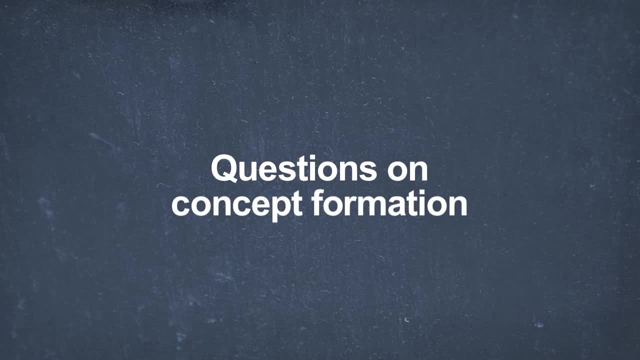 another one now. Yeah, I mean, I guess maybe I should have used another example, which is: you know, you have a hot, you have something hot and you need to put it down, and you wind up using a chair instead of a table. 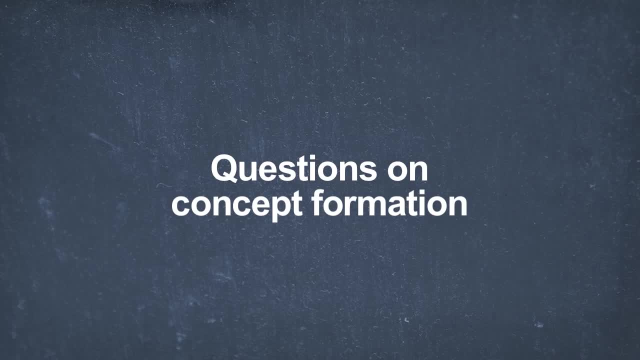 Maybe it's just The fact that you put something hot on a chair doesn't make a chair into a table. It doesn't, nor does it make it optional whether you include chairs and tables because you are able, and it's not even necessarily wrong. 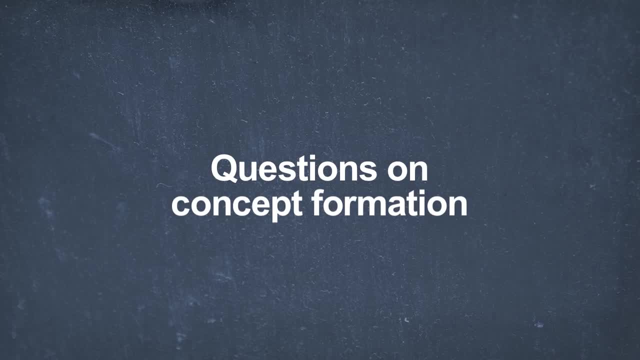 to use an object for purposes other than it is for which it's intended, up to a point, but it's inconvenient to do so, and that's why you use a table when you can. in the same way, you can sleep on the roof. That does not. 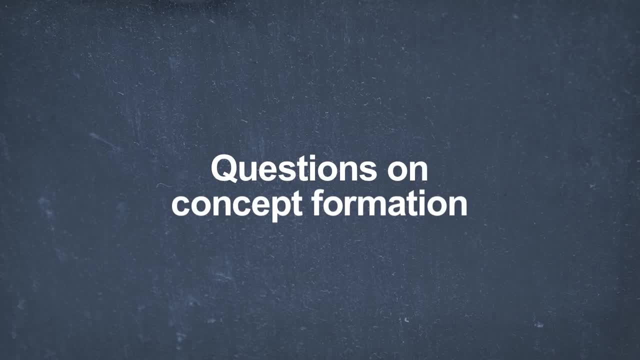 obliterate the distinction between a roof and a bed, It doesn't make it optional and it doesn't say: well, there's a long continuum, you know, and we just draw the lines wherever we want. That would be absurd, and so what you do do. 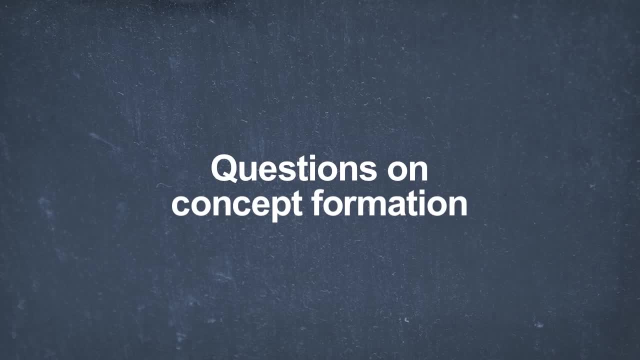 with something is not relevant. If it's a manufactured object, what is its structure and how is that structure by its nature intended? For what type of purpose? That's how you differentiate. You're really taking us into the next. do you see that you're? 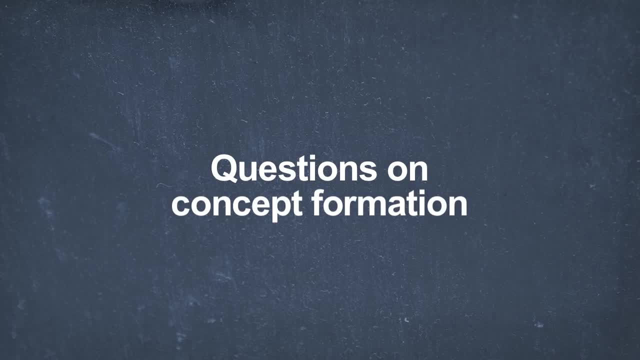 taking us into the next chapter At the back. Yes, I see on page 120, 124.. 124, I think that's right. Yeah, Bottom, this measurement condition applies also to non-essential characteristics. Excuse me, Where are we? 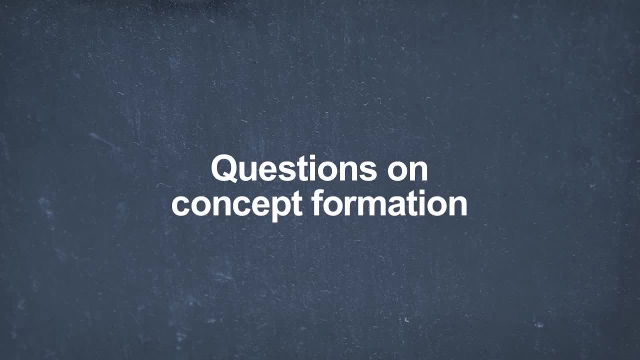 Quoting Rand: all particular measurements not only measure the shape but all the other characteristics of the table. Just tell me what paragraph. it is. That paragraph? Oh, I see where you are. Yes, Yes, it definitely I get it. 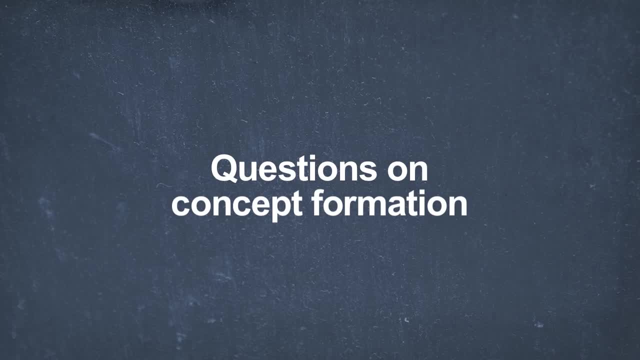 The question is, he's quoting Rand in the very top of 125, few words in the bottom of 124.. In order to reach the concept, the child mind omits all particular measurements, not only the measurements of the shape, but of all the other. 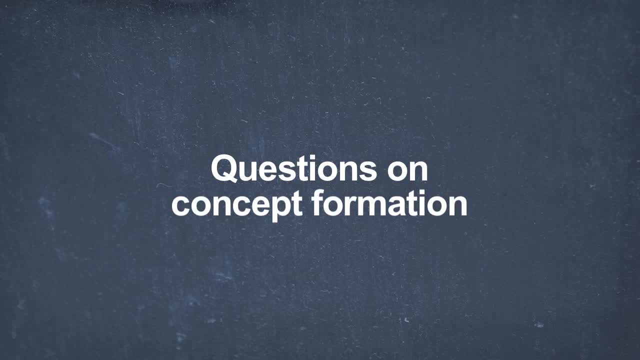 characteristics of tables, many of which he is not aware of at the time. Now, essential characteristic: if I understand you, you're speaking an epistemological term- That which is involved in the development of the world, which is involved, that which is 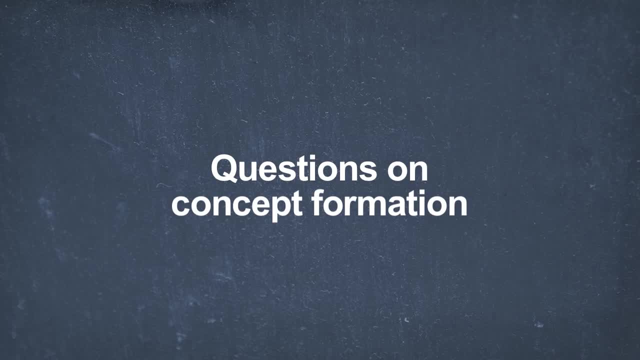 in the definition, that which is selected and turned into the definition. Now, a table has a tremendous number of characteristics that are not part of its definition, although they're implied by its definition. Friends, that a table has weight, That is not part. 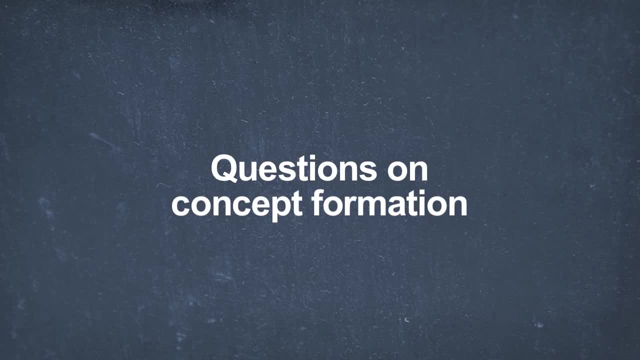 of the essence in the sense if you wouldn't say a table is a flat level surface with supports and weighs something, You don't throw that in because that does not distinguish tables from other things. So you can sit. I get your point. 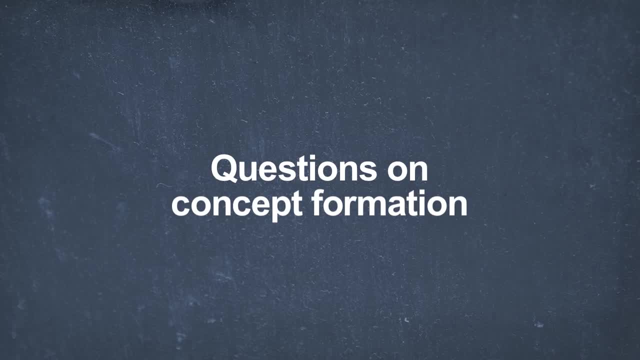 It's essential as a metaphysical aspect of a table. It couldn't be a table without weight, but it's not essential in the sense of part of the definition. Yes, The question is actually on non-essential characteristics. the example that comes to mind. 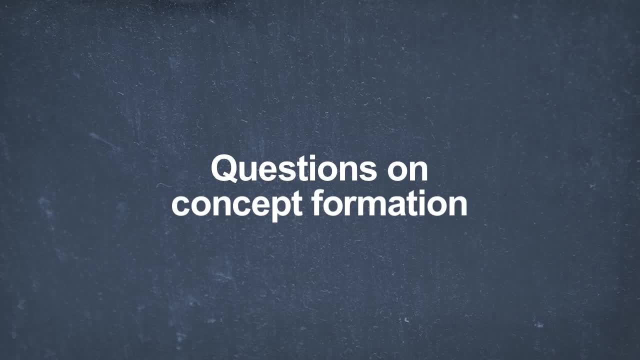 is for a pencil. Is which For a pencil? Yes, The principle of some but any is not applied to an eraser. Is there a pencil that doesn't have an eraser? That's right, So you have to simply make that. 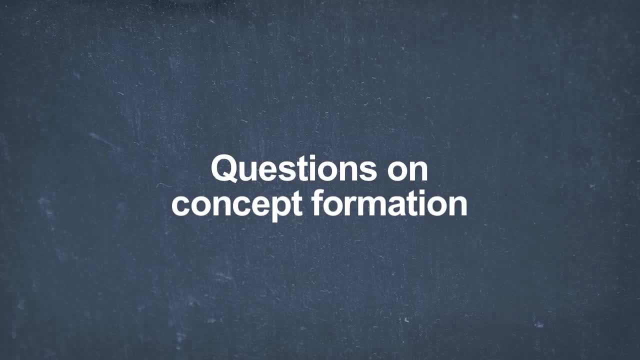 as a subcategory. exactly the way, if it was worth doing, exactly. These are the pencils. I forgot to repeat: Some pencils have an eraser and others don't. And how do you cover that? Is that just a difference in measurement? Well, 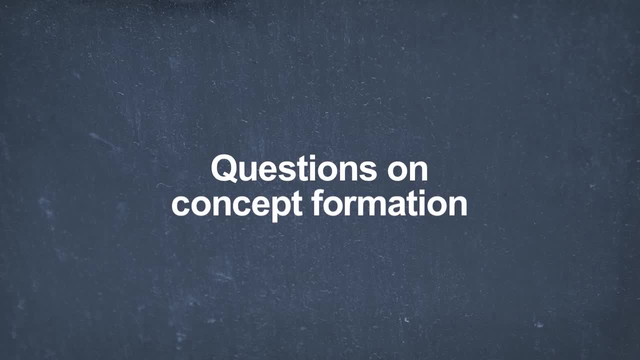 actually it is a difference in measurement because, if you go to how you perceive it, the eraser is a different texture, a different color, perhaps igne at center. All the perceptual observation of the eraser is simply variations on a continuum. 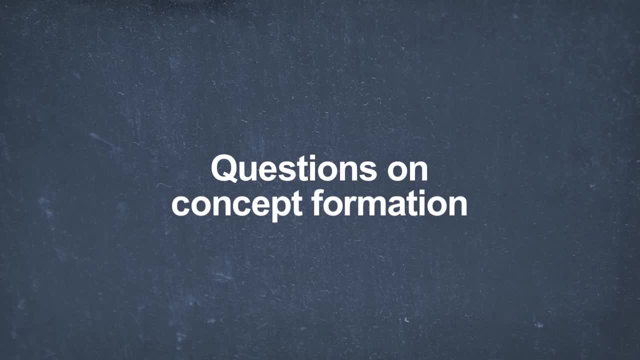 from the way an ordinary pencil feels. Harder and darker, let's say, and squarer, or whatever. But now the better way to handle it, since it's important to us to grab such a thing as an eraser, is to conceptualize. 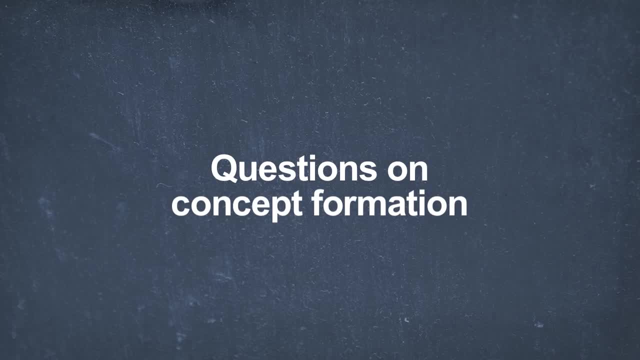 erasers separately, All of which vary from other erasers according to how eraseable they are. That's a degree issue, How big, what their shape, et cetera. They're all different measurements. And then say that a pencil with an eraser 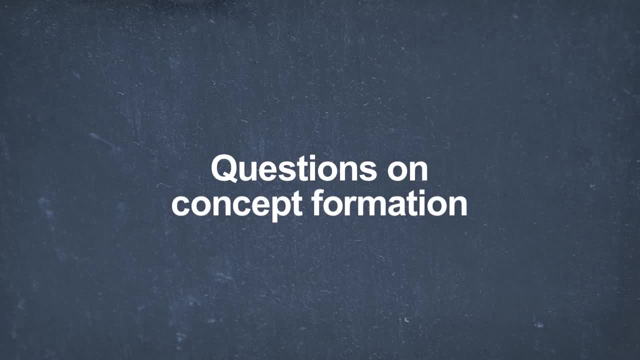 is a subcategory. within pencil, Just exactly on the model of what Ayn Rand does with desk, is a table with drawers for stationary supplies. So it's a subcategory which you identify by means of concepts describing its difference. Now, we don't, I believe, have a single concept. 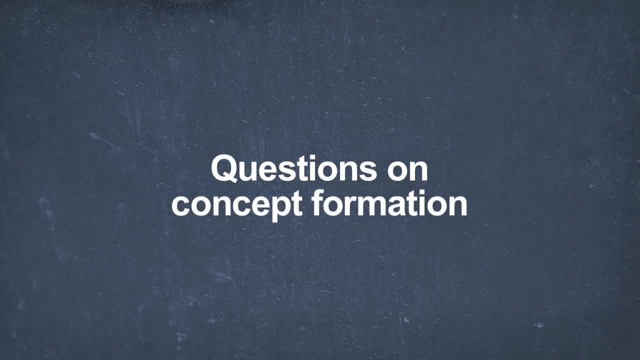 for pencil with eraser, So we haven't formed such a concept. If you have to handle that now, you have to say: I want a pencil with an eraser, And we handle it therefore right now by simply two concepts. 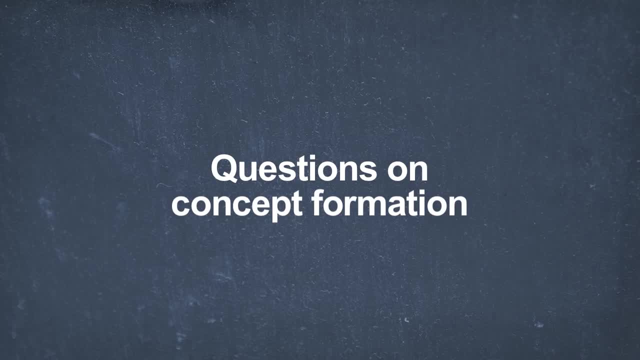 But if it was important, like desk, and it was a continuous thing, if it wasn't taken for granted and you wanted that, you would have to make a special term for it. Yes, On page 126.. Oh, I wanted excuse me before you get there. 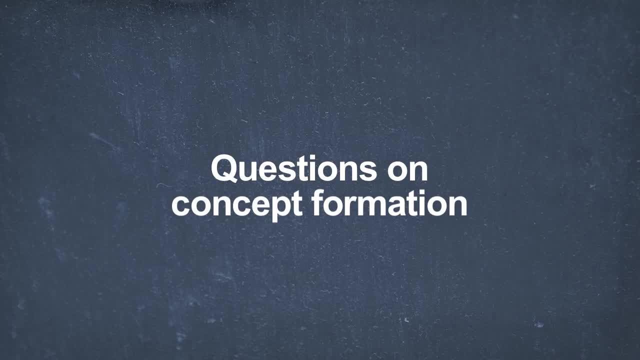 I just realized I wanted to say something about that sentence though, about omitting the measurements of all characteristics- Notice her parenthesis there- on the top of 125.. Many of which he is not aware of at the time. Now, that bothered me. 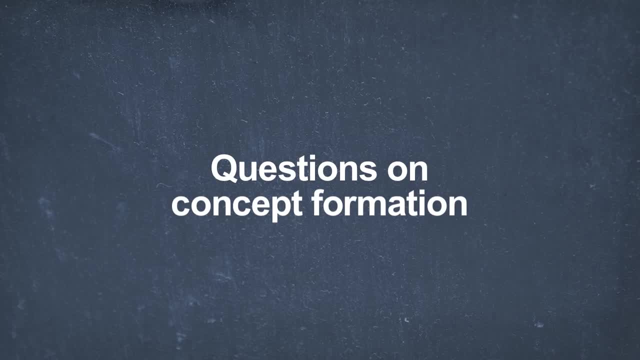 I remember having a discussion with her about that: How can you omit a characteristic you don't know about? I mean omit measurements of a characteristic of which you know nothing? I haven't, let us say, even discussed, discovered weight, yet 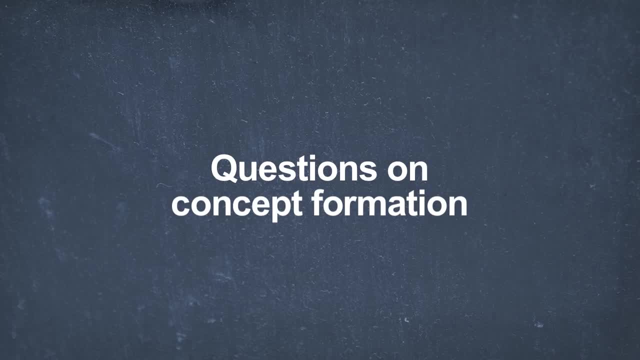 I have no idea of such a thing. I mean, I can feel the heft of something, but I have no concept of weight. How can I, in forming the concept, omit, How can my mind even omit measurements of something of which it has no knowledge whatever? 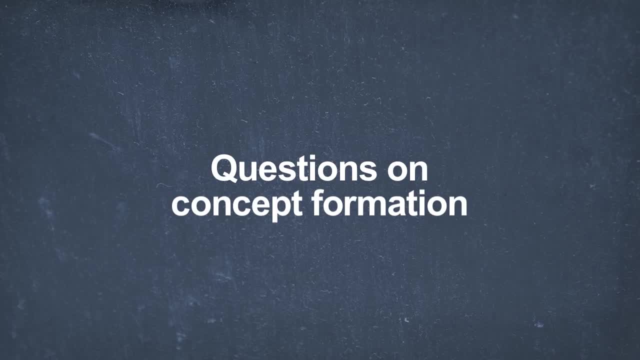 And that was one of the problems I had, and I gave the answer that she gave me essentially on the top of paragraph 126.. The mind doesn't omit measurements in regard to those attributes of which it's completely ignorant. It doesn't grasp commensurability. 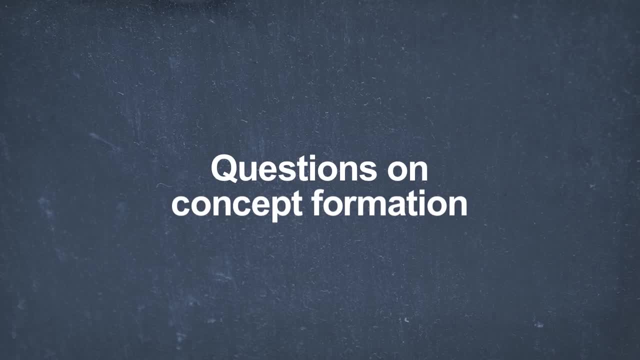 of all the weights to a given weight, even weight if it doesn't know anything about weight and that's outside its field of knowledge. In that sense, the mind-informing table, say, does not omit measurements in the way that it omits measurements of all the things it does grasp. 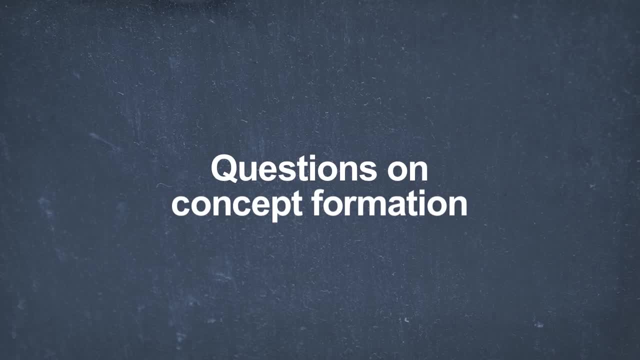 But it omits in a deeper sense. in this way, It's governed by a certain standing order, which is the nature of the conceptual faculty, And the standing order amounts to this. Whatever else I find out about these things, I'm going to treat the same way as the things. 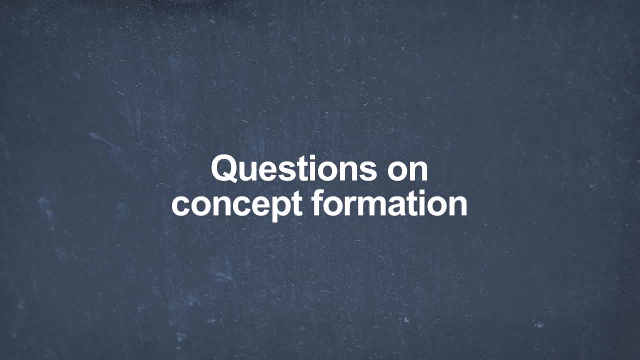 I already know, That is, I will retain the attribute characteristic and omit its measurements. And in that sense, as a blanket formula, in forming a concept, your mind omits the measurements of whatever it knows and says. in effect, whatever else is coming, I'm going to do the 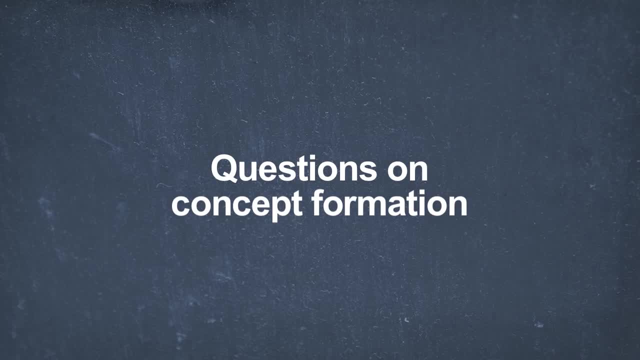 same thing, And thus, in that sense, it omits all measurements present and yet to be encountered. It's in that sense that she means her parenthesis, many of which she's not aware of at the time. It's like it's that issue of the file folder. 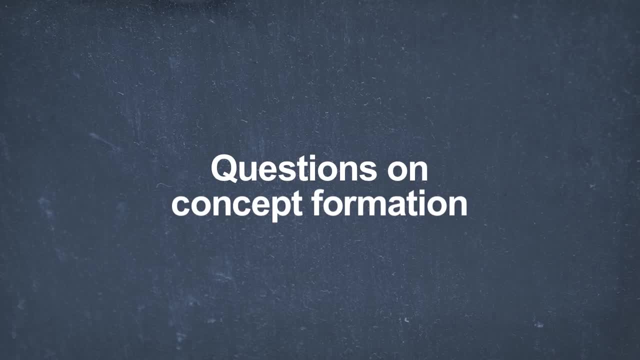 He makes a file folder. Oh, I forgot, he's ahead. He makes a file folder- the child or the adult- and he says and puts in there whatever attributes he knows, plus whatever are still to come, And that's it. 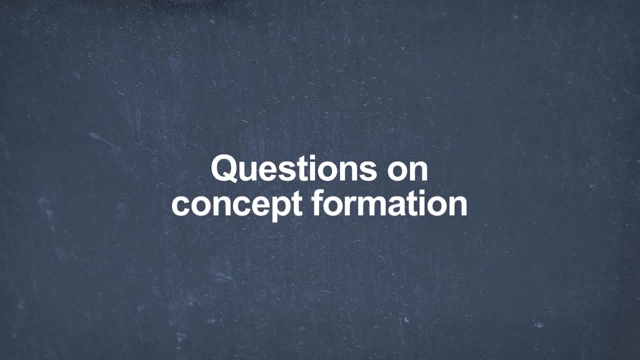 It will be processed. It will hold them all equal. Now you had a question. Yeah, And now I'll get to you. Yeah, Within that same first paragraph. parenthesis on the third and last line. Yeah, Within appropriate limits. Yes. 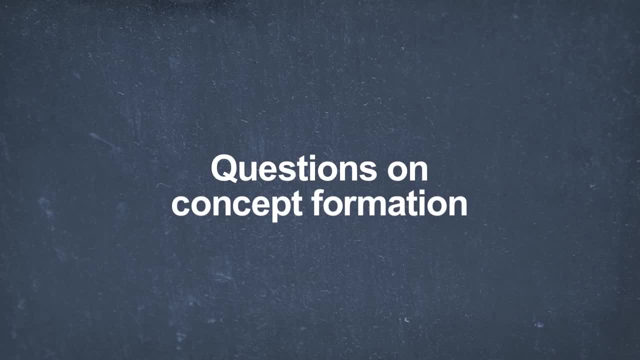 I like that. You didn't explain that to me. Yes, I didn't explain that here. Why do I say omit all the measurements paren within appropriate limits? Because No, Because many, many concepts have certain upper and lower limits of measurement beyond. 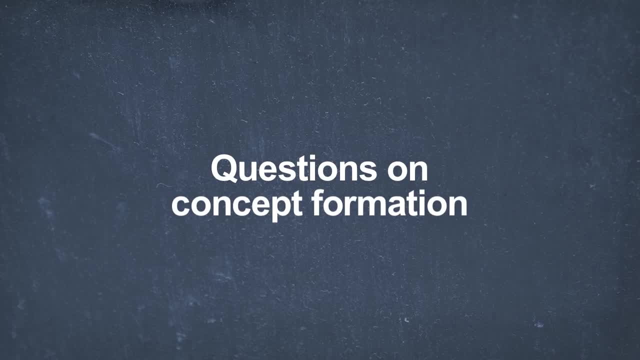 which the concept is not applicable. A table, for instance, cannot be atomic sized. You couldn't say: I don't care how tall it is, going down to one trillionth of an inch below human perception. even I would no longer be a table. 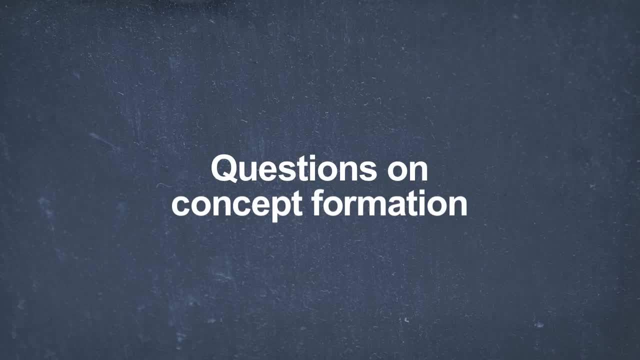 I would be an arrangement of electrons or whatever. By the same token, if you had a table that was 37 miles tall, you know that's extended out into the stratosphere or the outer space. that is not a table. Whatever that is, it is a new phenomenon requiring a new concept, erratically different from. 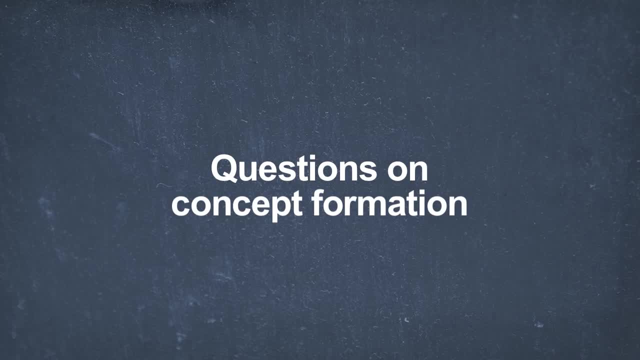 what we call tables, A table that you can get down, pretty small for a table and you got with anybody. cover that by saying a toy table, See, But we have to even say that. But once it gets below that, it's out. 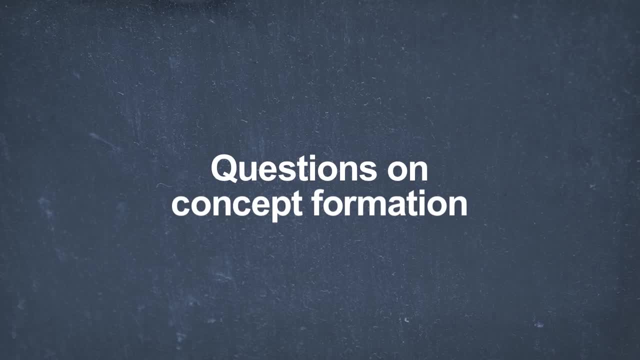 And the same token, it's a really big table. but beyond that, whatever it is, it's some kind of aberration. It's not any longer within the scale of human use, And this is true of a great many concepts on a great many dimensions of measurement. 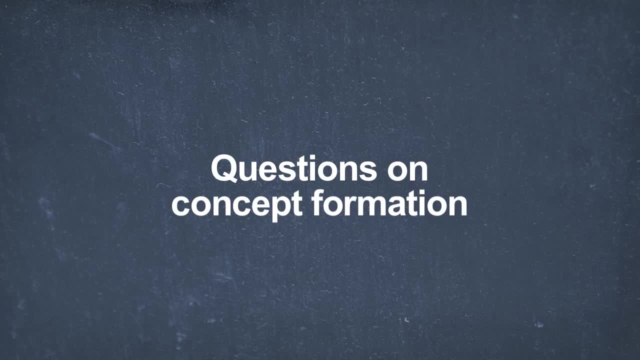 You omit measurements within a range, but there's an upper and a lower. The boundary may not be, you know, really sharp, but there's a fuzzy. Yeah, You know, borderline-type area, But that's why, you know, you can't say every qualification in every sentence, but I want. 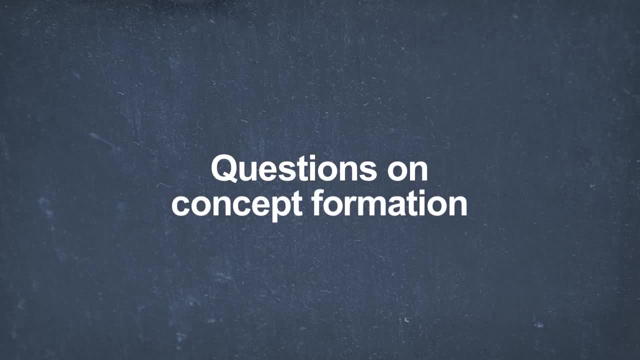 to indicate here that you don't just flatly omit anything to do with measurement, because you'll lose the category you're talking about if you do that. Yeah, Oh, wait a minute, I promised you over here. Yeah, Yes, Getting back to this point about omitting measurements of characteristic- that you're 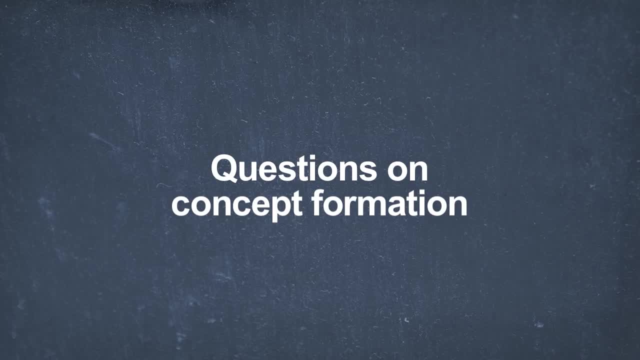 not, may not be aware of at the time. Yeah, Yeah, Yeah. This applies also to the state of general human knowledge at the time, And I can't get away from this, from a maybe what's a preconception on my part, that 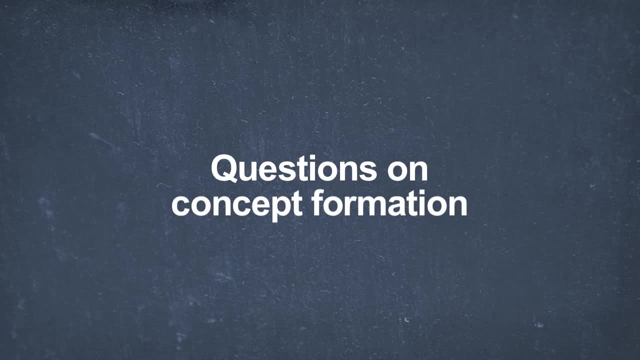 this could lead to a kind of reductionism, For instance, when you omit. somewhere in the introduction to epistemology it mentions omitting a color and says that that's an example of measurement omission because it's quantitative. We now know that color can be measured quantitatively as a frequency. 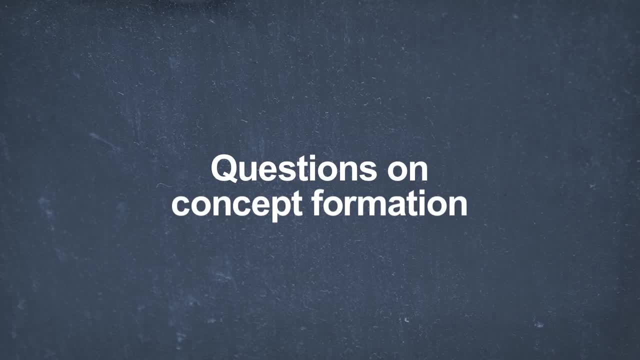 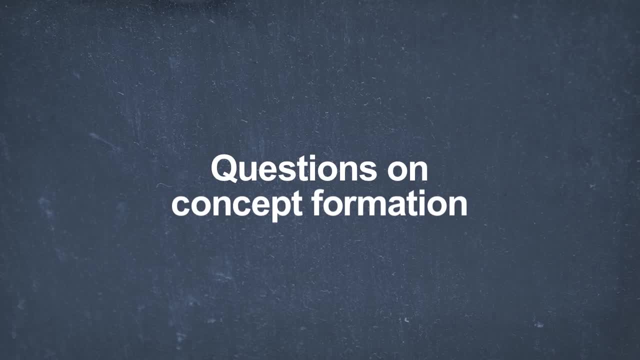 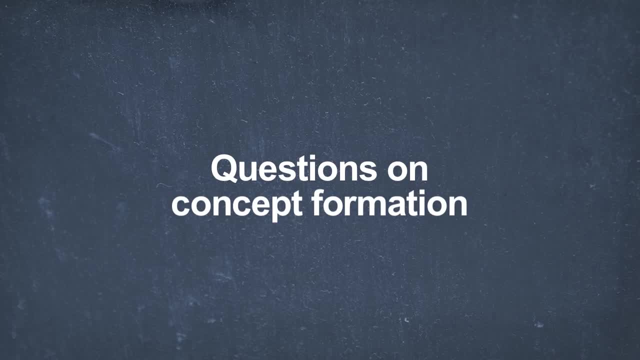 frequency, But in the state of human knowledge. I get your question. this wasn't known. I get your question. it would be appropriate to call that a measurement. Perfectly good question. Let me first state it and get it back. 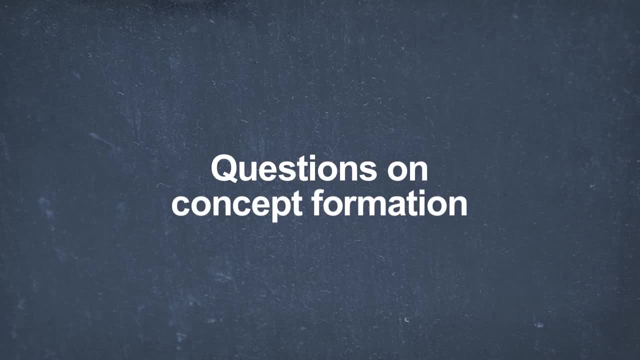 Is there a reductionistic element in this theory of? he gives the? I mean of an improper materialistic kind. He generally gives the example. Ayn Rand talks about omitting the measurements of color And she thinks that you can treat variations in color as differences in measurement. and 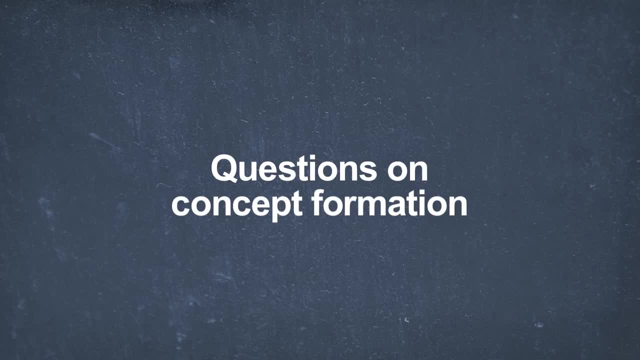 she gives us the example that science has finally discovered light waves, which are actual numerical, quantitative measurement, and that is the underlying proof of it being measurable. And he says: does that amount to saying every quality is reducible to something mathematical? and what's, therefore? we're gonna end up as Pythagoreans, in effect, that what's really. 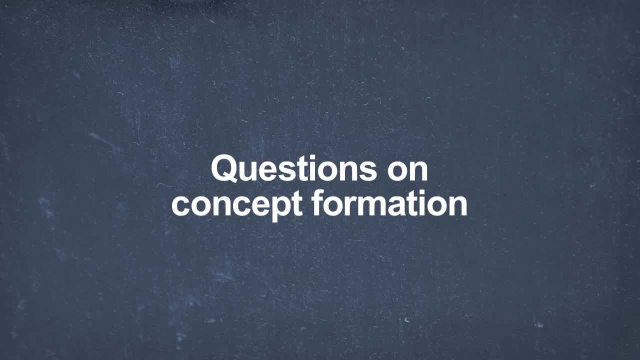 real is only the underlying mathematical structure? No, emphatically not. To begin with. if science had never discovered the light waves, concept formation would be unaffected. She used that simply as illustrative of the fact that, in this instance, we were able to. 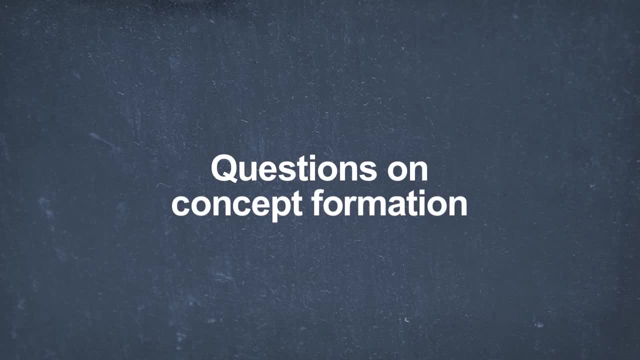 translate our conceptual implicit measurement into actual numerical. but there's nothing in her works that I know of that's. She says this is a metaphysical necessity. nor is it an epistemological necessity, That is, if we never discovered light waves, we would still perform implicit measurement. 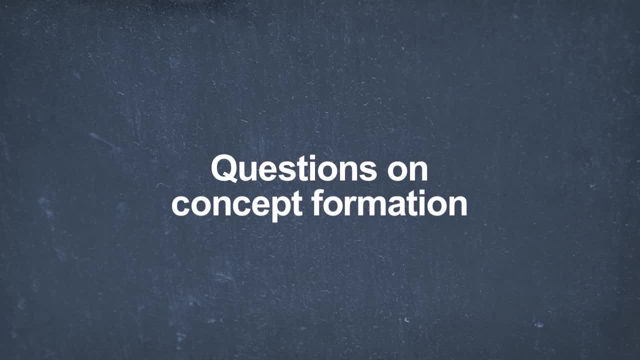 on colors exactly as we did on length, That is, you would see simply a spectrum: darker, lighter, more intense, less intense, duller, etc. And you would be able to put all the reds, for instance, leaving aside the borderline. 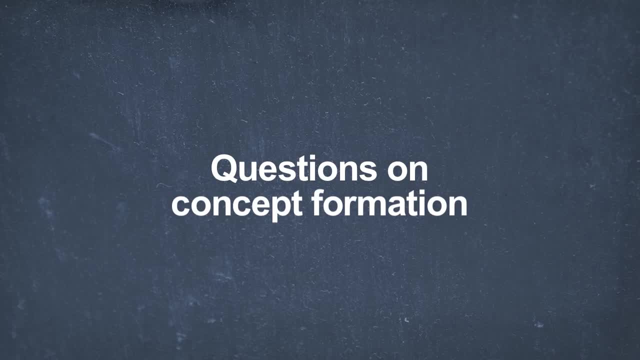 issue here, as against the greens, You would see a variation and it would be that, more or less, which is the implicit measurement and that would apply whether we ever discovered light waves or didn't. Yes, Sure, Okay, So you're saying we would just say it's an implicit measurement and we're omitting it? 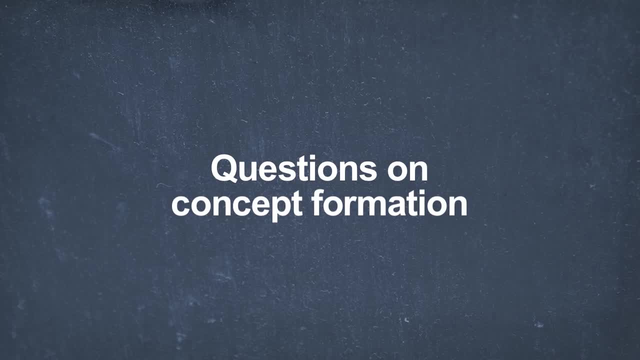 Well, all concept formation is implicit. Yes, Yeah, But if you say it's, If we say it's an implicit measurement and therefore omitting it, therefore we omit it and that's this concept formation. doesn't the word implicit imply that it's gonna be? 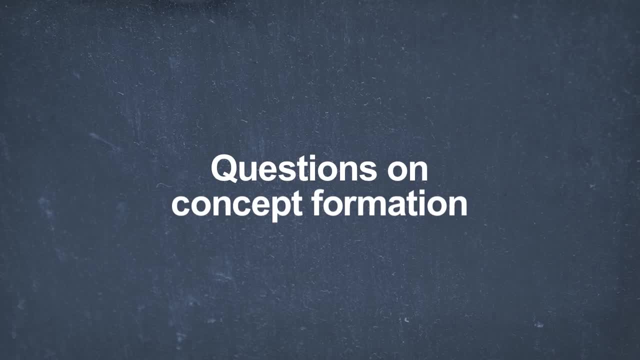 explicit in the future and No, Definitely not Implicit. Now, that's my term here of calling it implicit, simply to say that it is a process that does not, That takes place on the subverbal level, and it does not require or involve the use of. 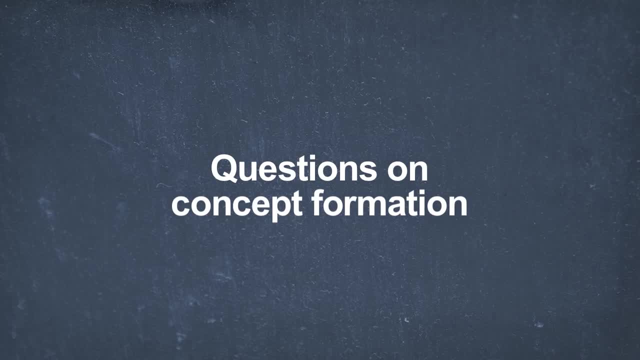 numbers specifically. It does not mean that you will ever necessarily do explicitly and in a tremendous number of cases I don't think we know how to do it To this day. there's a tremendous amount of things that we can't measure. I have a paragraph here on page 129, the second paragraph, to learn how to express in numerical. 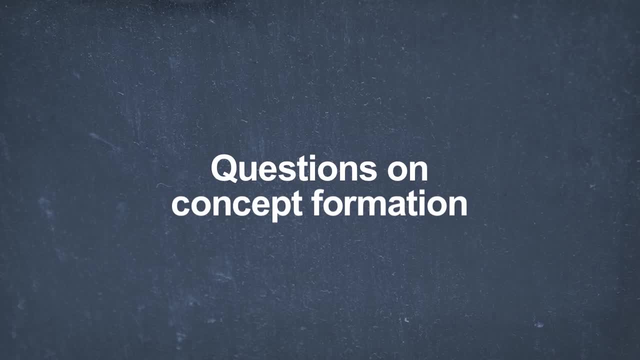 terms. the implicit measurements involved in concept formation is a later development which is sometimes relatively simple and sometimes not. It is not always easy. There's a tremendous amount I'm sure we cannot measure now. That's why That someday we'll be able to measure in the sense of define a unit explicitly and then 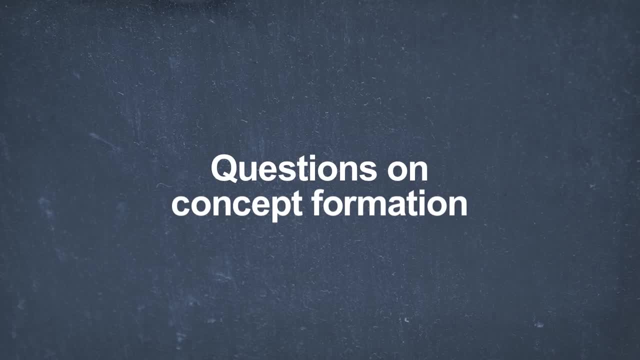 apply it to all the instances. When we say implicit here, I do not mean a process which we can, when we grow up, turn into words. All we can do is put explicitly the content more or less commensurable. That was the essential idea that we get from watching this Spectrum. 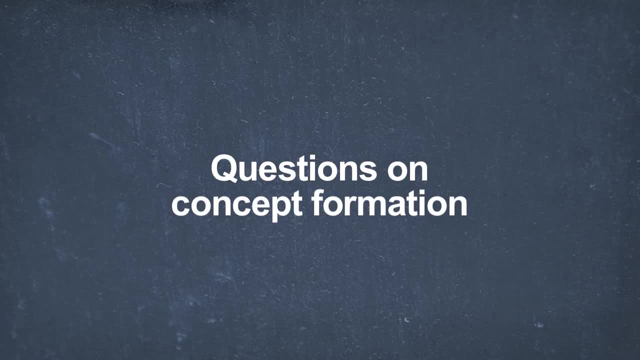 Spectrum or continuum of more or less. That's all we needed for concept formation. That much we can put into words, But the actual translation into numerical measurement is not something that we can do just from having that information. That's far advanced knowledge. 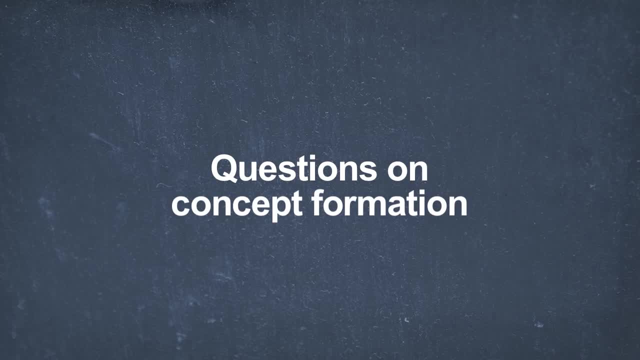 There's no implication that the human race will ever be able to. No, There is no implication that we will ever be able to do it or that there's any timeframe of how we'll be able to do it. We have reason to believe that. 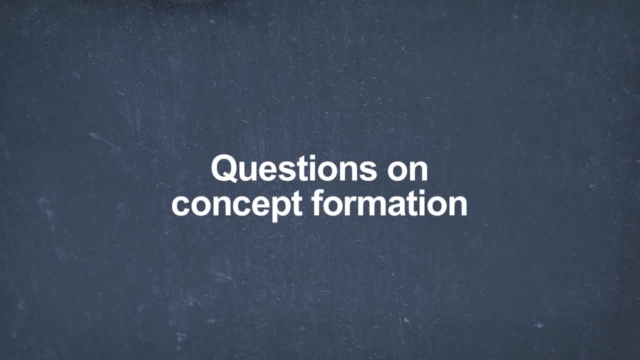 Yes, that whenever we have taken any attribute or quality and science has reached a certain point, we have found a way to do it. But we're not making a metaphysical dogma out of this, because nothing hinges on it. Reality is still what it is and the concept of any given attribute is still reached by 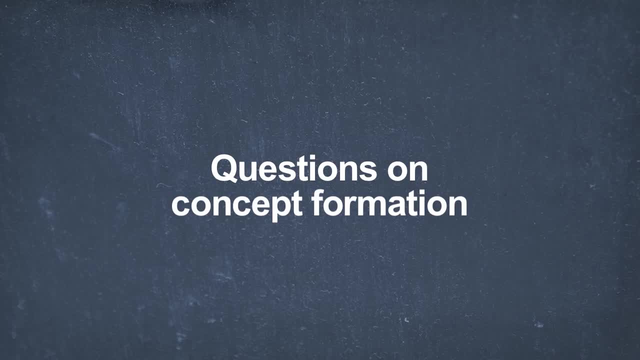 implicit measurement whether or not we reach the stage, So that, for instance, way before they discovered light waves, the concept of colors was perfectly well. So there would be no philosophic significance or point to insisting that everything is ultimately reducible to some kind of mathematical structure. 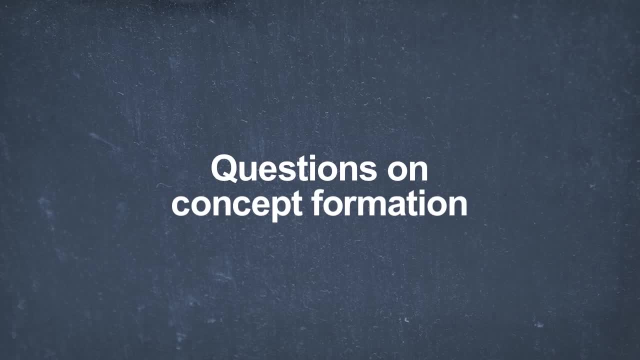 Beyond that, just let me add one further clarification. I don't mean to erase color out of existence either. When we talk about light waves, let's not fall in the trap of saying what's really real is the light waves and color is just a subjective effect on us. 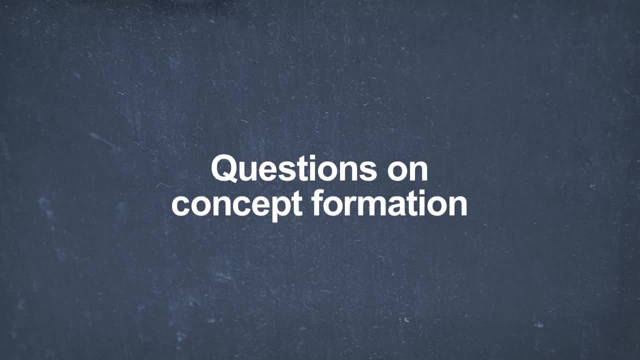 So be careful. We're talking about reducing color to light waves. Yes, What's the difference between like and love being a perfect example of that? Because not only, would there not be perhaps a- Well, I don't know. That's exactly the answer. 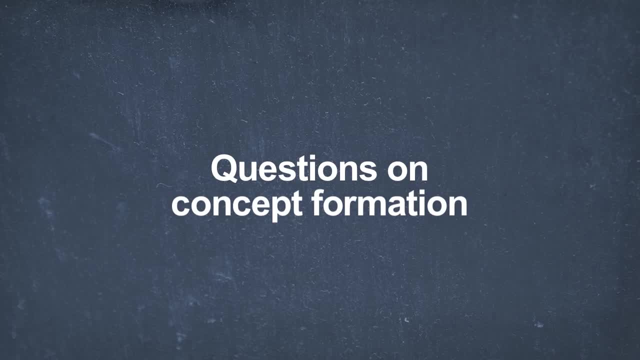 You say, wouldn't the concept of like and love be a perfect example of something that we can use implicit measurement on? We can grasp a more or less in all the different states of liking, and thus we have a continuum from which we can grasp. 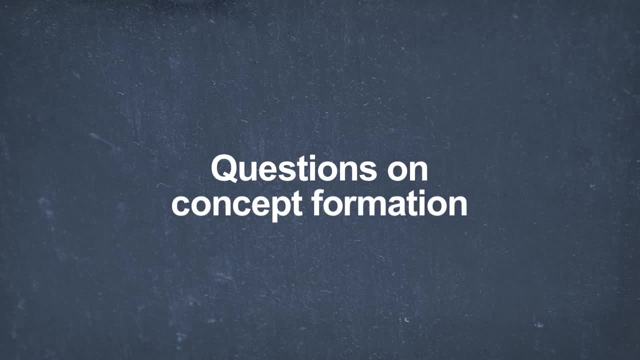 You know commensurability without having any quantitative numerical explicit adult unit? Yes, certainly that is an example, but I don't wanna dogmatize about the next millennium Suppose, for instance. now, I know this cause a heart attack on some people, but I'm just 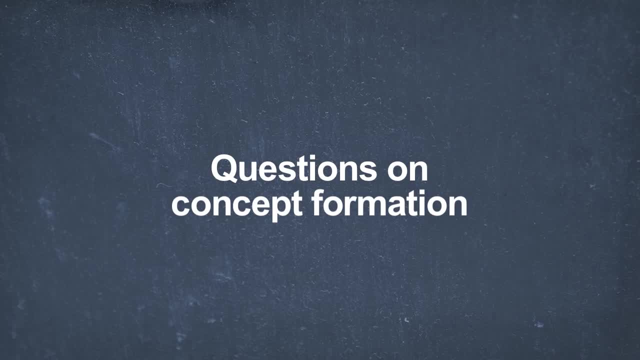 theorizing out of the blue Suppose someday, since the brain and the mind are correlated. Yeah, The various bodily organs are correlated with the brain. There was some little gizmo that twitched whenever you liked somebody it twitched in the brain. 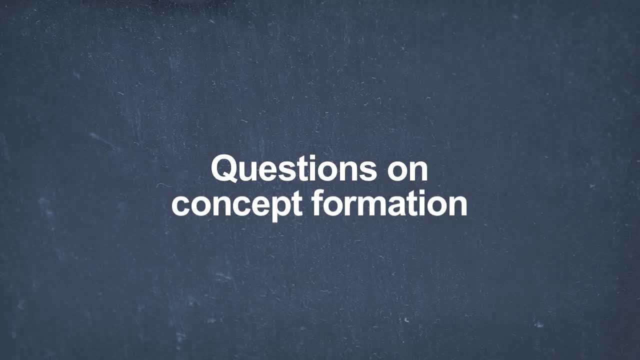 And the more you liked them, the more it twitched, et cetera. So that, in effect, was the substratum, the physical correlate of the experience of liking, and you could detect that and measure it. Then someday you could say: he likes her 3.8,. you see, 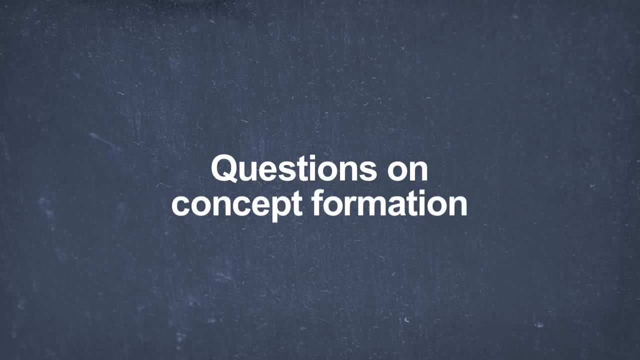 Now we can do that. Now I don't say it necessarily has to be a physical thing on the side of thewithin the brain. I leave open. I just don't know. And if you don't know there's no use saying I can't conceive of what it would be. 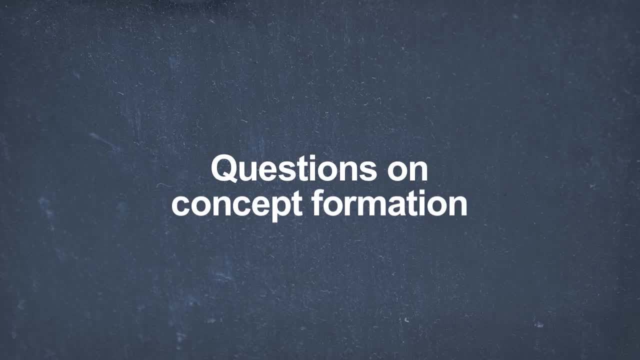 Because that is using your ignorance as an argument. All we can say, philosophically, is this: We can perceive this continuum. We can therefore conceptualize what science will one day be able to do in terms of translating our implicit measurements into numerical measurements. Okay, 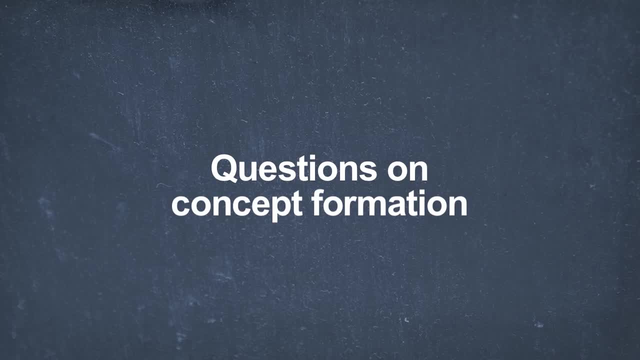 We can't say. I don't know whether they always can or can't- I would be curious to know. but you'll never find out in this life. So once you know that you're not gonna find out, I lose interest because there's no next. 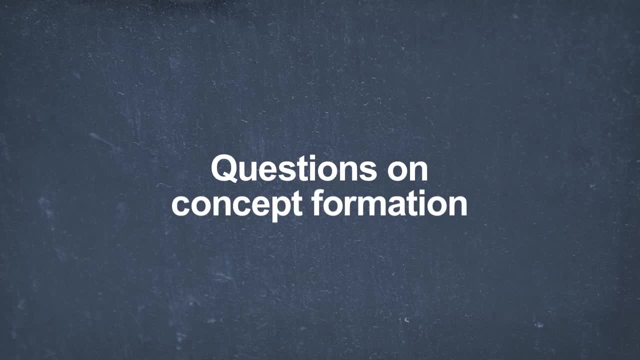 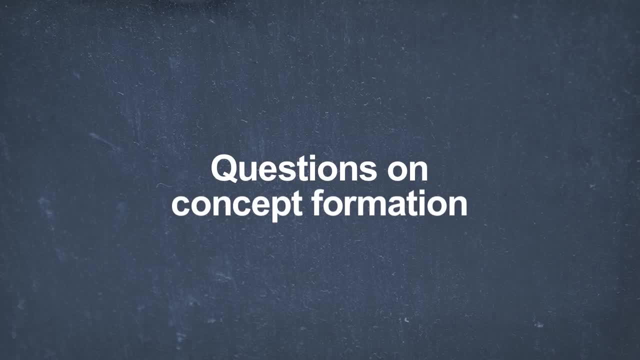 Yes, Yes, Yes, Yes, Yes, Yes, Yes, Absolutely. Just try it again A lot more precise. Okay, Someone in the audience wants to know: on the broad spectrum model, is there an assumption about all attributes being real, both actualized and potential? 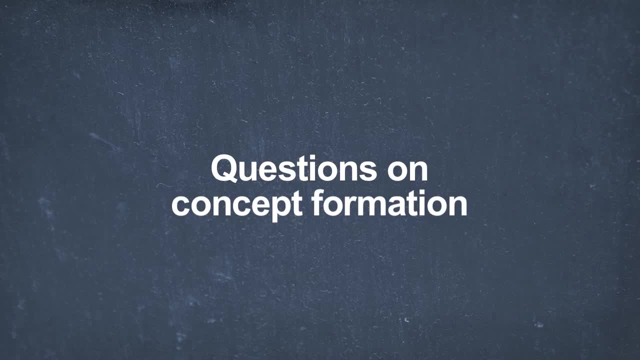 mistке, What do you think of the notion of applying that prospective to concepts in our usage here, to recognize a resemblance between the open and the nature of different? What does happened? He went to the hospital, He went to the doctor of concepts as, for example, incorporating new units. 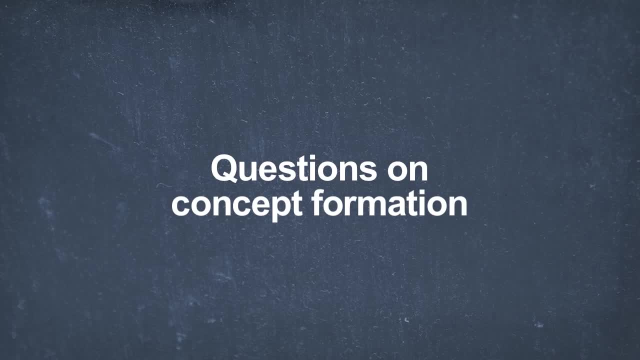 as they come along, or incorporating these knowledge to modify the concepts that they make. Well, I want to cut you short, if you will, because you're making a specialized reference to Aristotle and I don't think it's really of general interest. 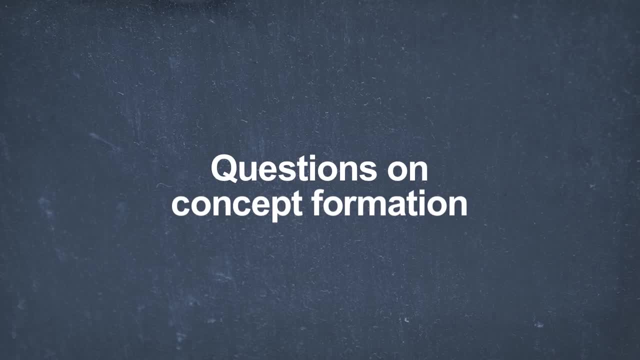 nor do I think I really get you Open-ended, as Ayn Rand is using. it applies to the relation of the concept to its instances. That's one primary use And it means it includes all the instances, past, present or future. an unlimited number. 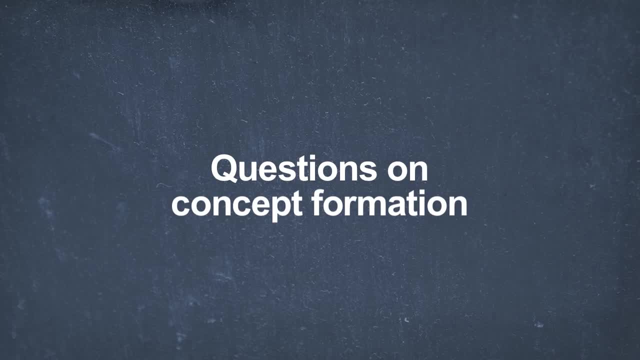 You can also use open-ended to mean it stands for or subsumes all the attributes known and unknown and therefore still contains room for further attributes to be grasped. Now you can use the word potential. It has this potentiality. 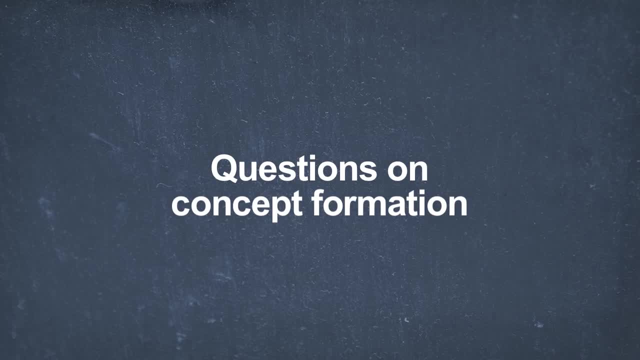 But I don't think it adds anything to say there's actual versus potential attributes, because that makes metaphysical what is really important. It's really only the distinction between what we know and haven't yet discovered. And because Aristotle uses potential and actual in so many different ways, I would 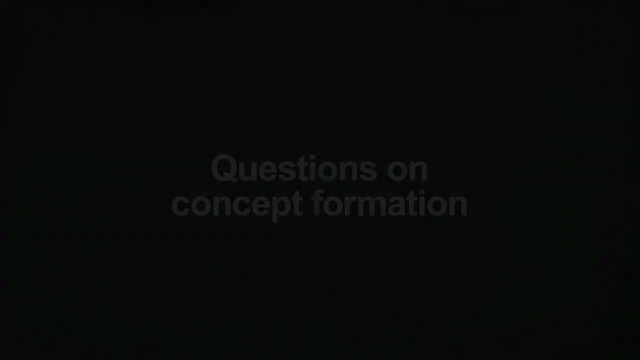 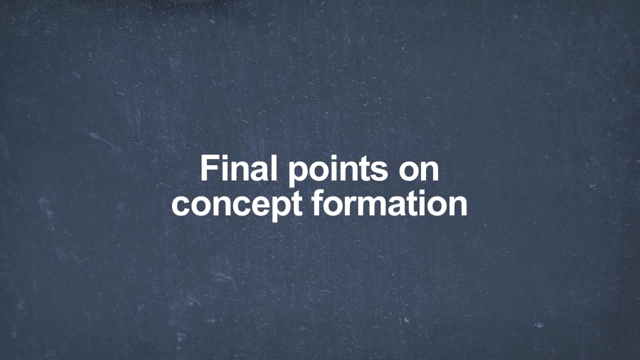 be very hesitant to import his terminology to this point. Now I know we're out of time. I wanted to make one last point, if you turn to 1.33. Because of technical difficulties. the following sentence of Dr Picoff's: 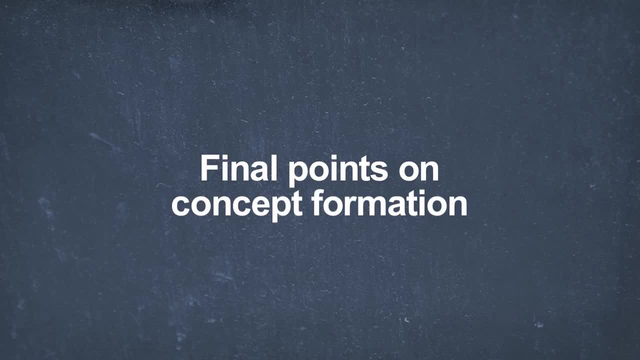 did not get recorded. I want to stress the point that in concept formation, even though we omit measurements and use a human method, we do not create any cognitive distortion by doing so, And this point is made in paragraph three: Concept omits measurement. 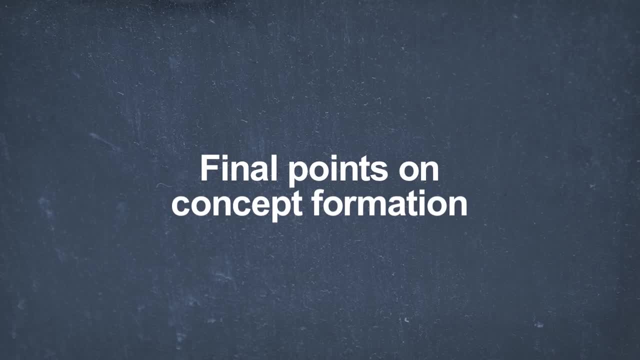 It's not as though it leaves out, distorts, alters or changes its reference. It includes everything about them, including the fact that they're commensurable And, as a matter of fact, if you want to, you can use concepts actually to tell you. 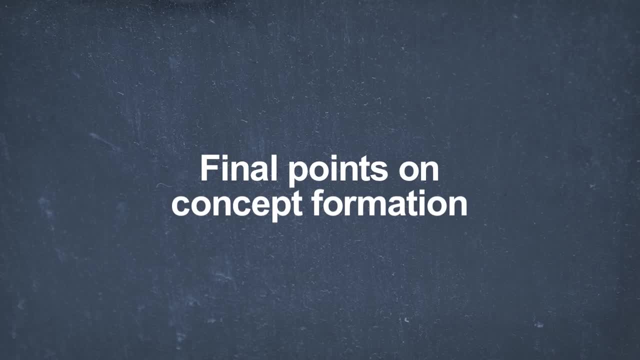 the particular measurements, One single concept. man won't tell you that, But if you use a whole cluster of concepts, you can discover a ruler and then use it to measure your height and say Rose's height is exactly this and her weight is exactly this. 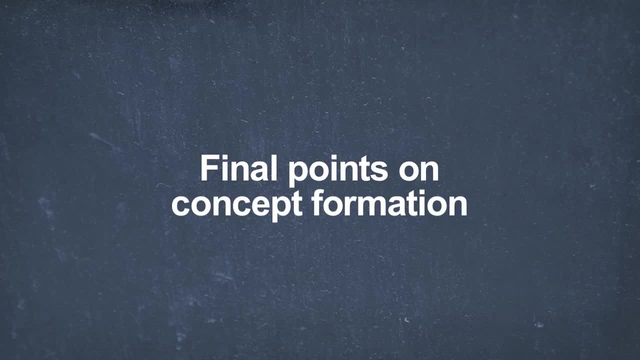 And I can state page after page after page of description in specific measurements. All of that is using concepts and the sum of it captures, captures, her. I'm saying this because there is a whole tendency in the history of thought to say concepts are blind to one aspect of reality. 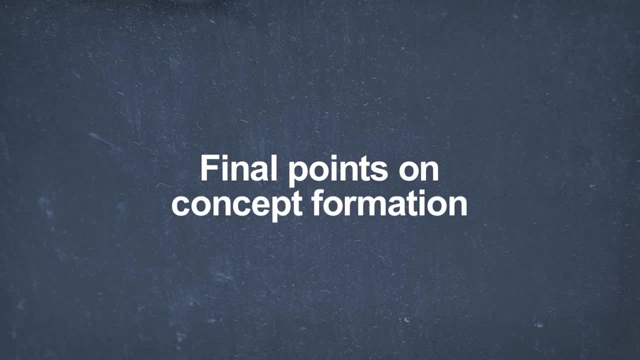 They capture what's common, but they omit or leave aside, or leave us blind to what's unique, And therefore they're a distorting mechanism. Unfortunately, that comes from against his intention, from Aristotle's approach, because for him, since the issue is metaphysical, 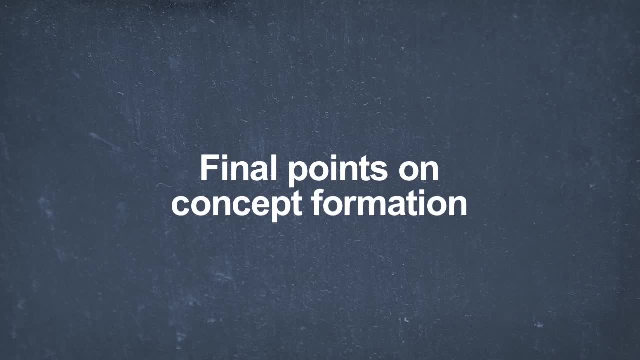 there is sort of a nothing in particular which each of us has in us, Which is unique, which makes us this and which is unknowable, And I want to stress that objectivism has nothing to do with that point. The method we're talking about is not a partial awareness. 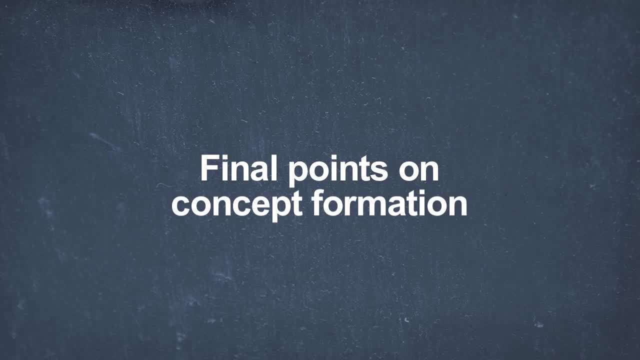 and it doesn't in any way introduce a cognitive distortion. The concept includes everything, including the fact that the units are commensurate. All it doesn't do is specify the different relations they have to a unit. That's it. It leaves it open for you to specify. 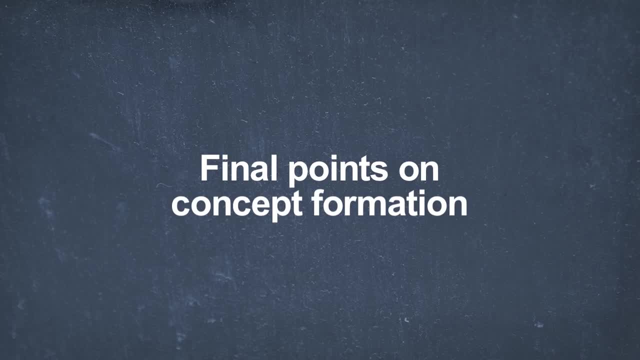 So no one can ever accuse concepts of being. they're human, but that does not mean they are subjective or anti-reality. Now I hope you see in conclusion why this whole topic, technical as it is, is very important. Now, 132, I allow myself one of the very rare. 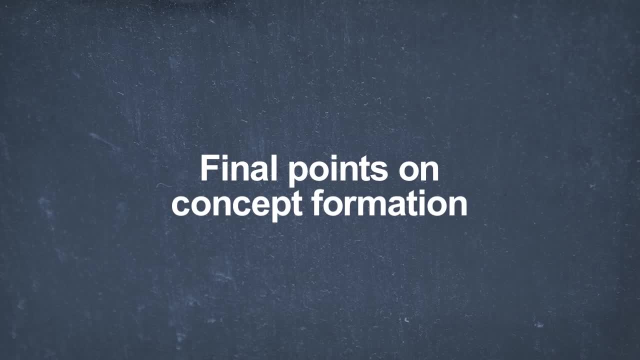 emotional metaphors in this perfect world, or purposefully dry thing when I refer to cancer remission, metastasizing- And the point is, of course, that this is really a life and death topic- I do think a proper theory of concepts is necessary. 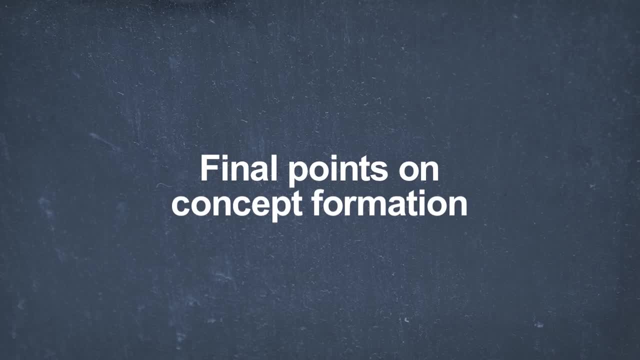 as I say in the middle, paragraph 132,, to save the world It's not enough, but you won't get anywhere without it. And then I like, if I say so myself in conclusion, that next sentence, the fact that concepts are valid, whether we 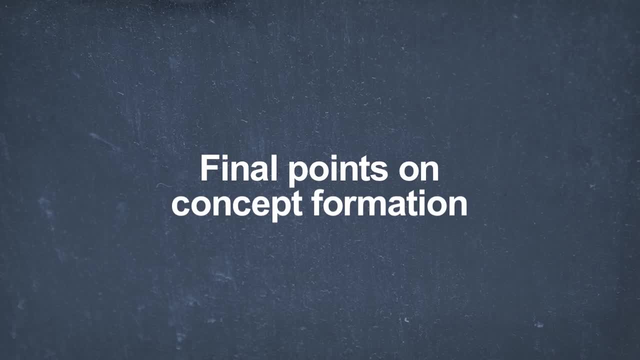 know it or not won't save us, not unless we do know it. And why is that? What would be the answer? Someone says: well, concepts are valid whether you know it or not, So who cares whether you can validate them?